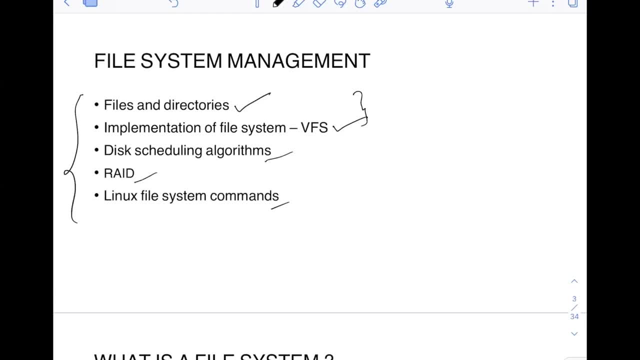 this scheduling algorithms, uh raid and linux, uh file system commands. so some of the linux file system commands i will cover in this video itself and some in the next part. basically file system management part two. basically whatever is left, i will cover that in next video. let's start with. 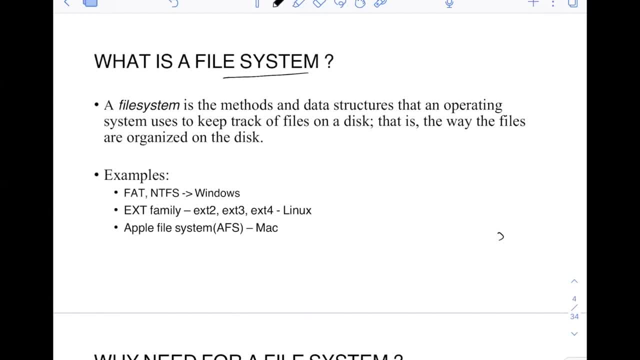 what is a file system? so this is one of the definition of file system. if file system is the methods and data structures that an operating system uses to keep track of files on a disk, that is the way the files are organized on the disk. so the definition of file fiction is very 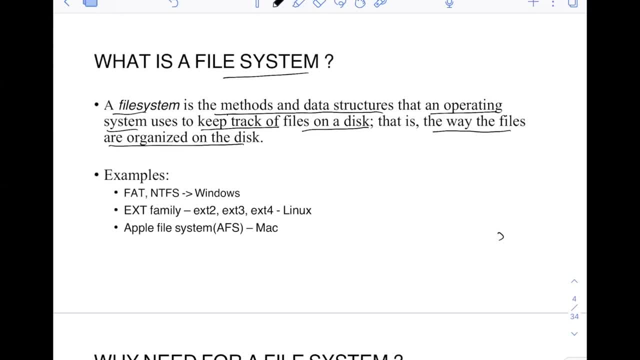 very important. so you should understand what actually is file system. so file system is a very important concept in operating system. so do not think that the disk itself is the file system. that's wrong. so you have the files, so you have the disk, basically right, where you store some data. so let's say this is: 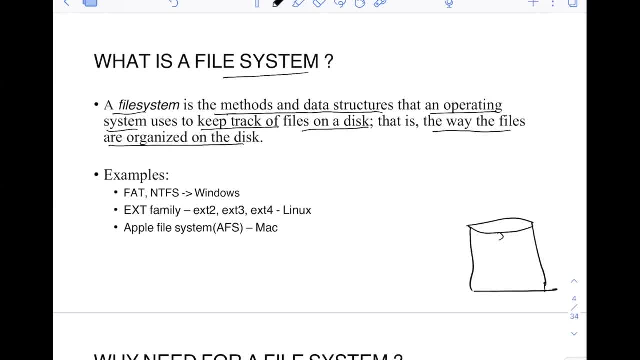 the disk. now, i mean there has to be something right, uh, which manages the disk, so which helps in writing the data, reading the data, searching the data. right, because see we as the users, for example, we, uh i mean we are, we are mostly telling the operating system or the cardinal right. 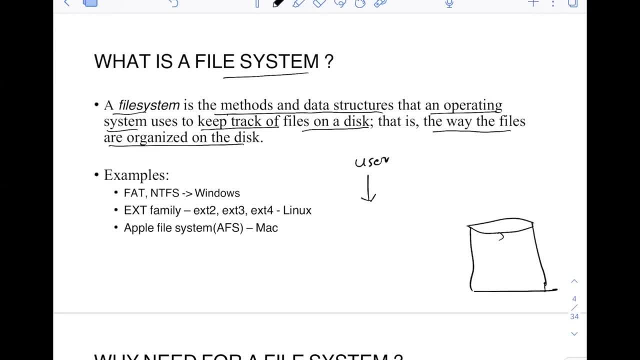 so the people user will be there, and then there will be kernel here, okay, and at last, uh, let's say, there will be your devices, all your hardware devices will be there, and of course, one of them will be this box. right keyboard will be there, disk will be there. uh, ram is there. we have already. 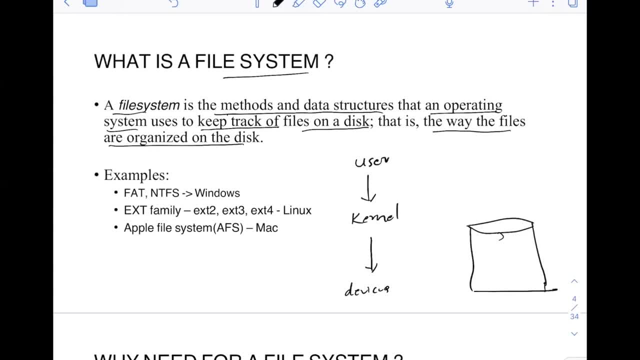 discussed about ram already right in memory, uh management, and here we are discussing about uh, i mean disk and other hardware devices, basically in file system. so here we have, like, in this device, you have the disk also there, right? the user will typically say, okay, i'm want to read, to read this file, i want to write this file and of course, all of this has to go. 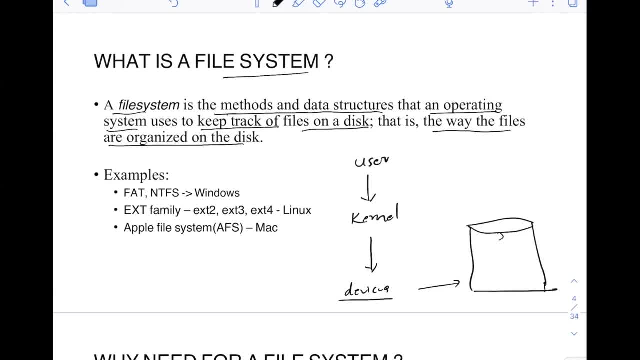 through kernel, because kernel is the one that manages all these hardware devices. so whenever you tell the kernel to read or write the file, okay, now the kernel- i mean kernel- has to talk to this uh disk. right, so how can, how, how, how can the kernel talk to this disk so it uses the file? 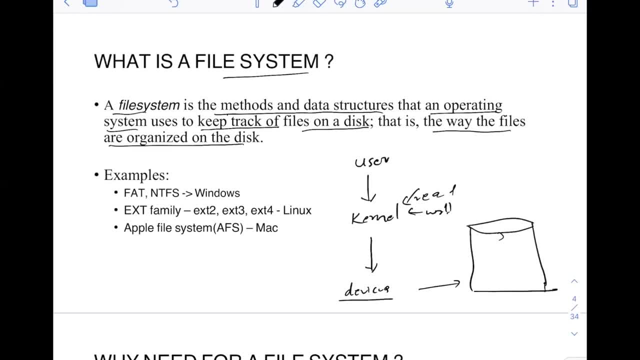 system. basically, to talk to this disk, right, and this file system has a lot of data structures, animators that are used by the kernel. when it is talking to this, hardware devices- and hardware device, of course there is the disk. here now some of the famous examples of file systems like in: 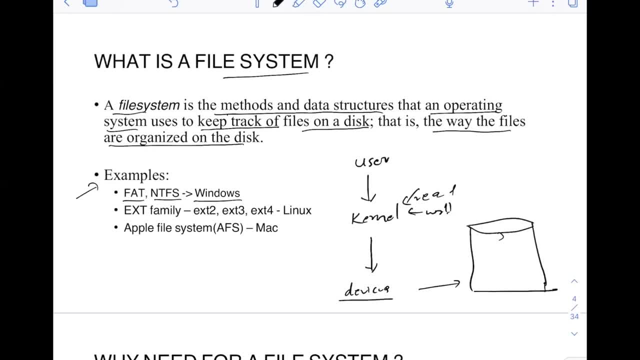 windows you have pat and anti-fs. these are some of the famous file systems in windows. in linux you have ext family file systems like ext, ext2, ext3. now you have ext4 also. right like this is the different versions of ext. now in mac you have afs or apple. 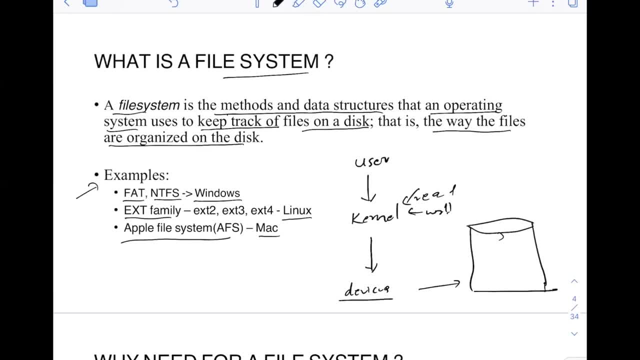 file system. so these are some of the file system that i'm discussing here, and there are a lot of files. i do remember one thing: like whatever i am discussing in this video, i am discussing all of this in terms of- mostly in terms of linux operating system, right? so? 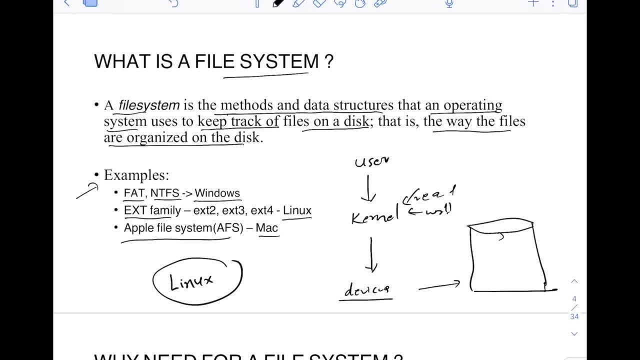 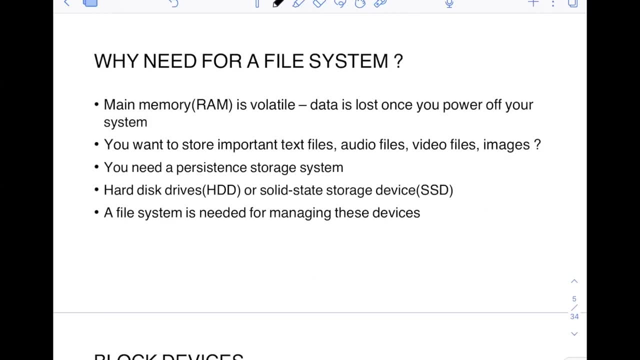 whatever concepts i am discussing here. so i am discussing file system with respect to linux operating system mostly here, not with respect to windows or mac mostly. but yeah, some of the concepts may be applicable to all the operating system, right? the next question is: why need for a file system? so what is the need for a file system? why does open system? 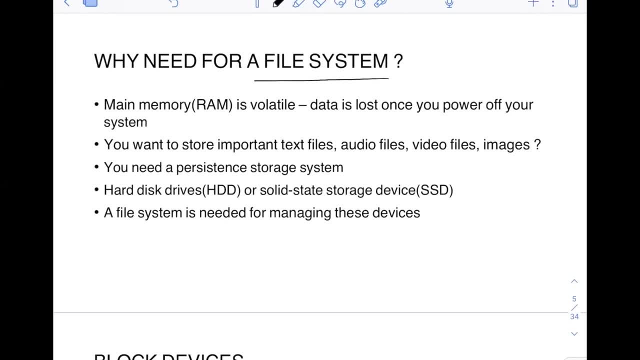 needs the files makes the file system okay. so main memory, ram or of course ram we have discussed- is volatile, that is, data is lost once you power off your system. so main memory or ram is like used for storing temporary data. you cannot store permanent data in ram. 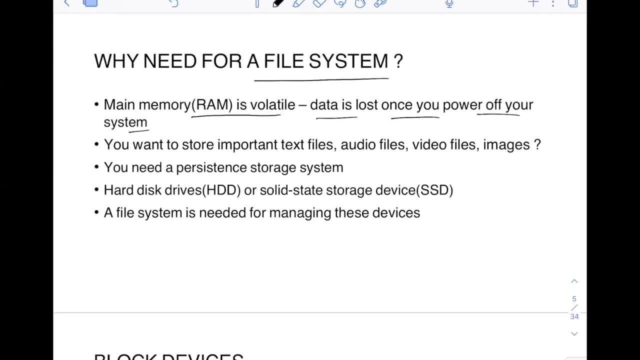 so for permanent data you have to use some other form of storage. so let's say, if you have to store some important text files, audio files, video files, so you have to store some important text files, images. now, these are not temporary files. you need this all the. 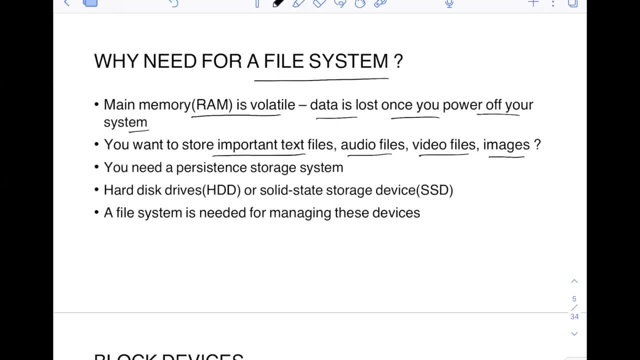 time on your system. so you cannot store these on ram because of course on ram if you power off your system it gets lost. so you need a persistent storage system and that's where basically uh, hdd or hard disk drive or ssd, solid state storage drives, so this type of 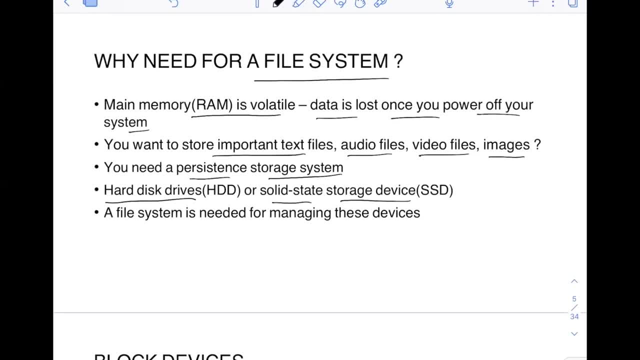 devices helps in permanently storing this data. now, of course, you have these devices and gd, ssd, but still the operating system needs something to manage this device. so you need a hard disk or hard disk drive. for example, you have a hard disk drive which is a file. 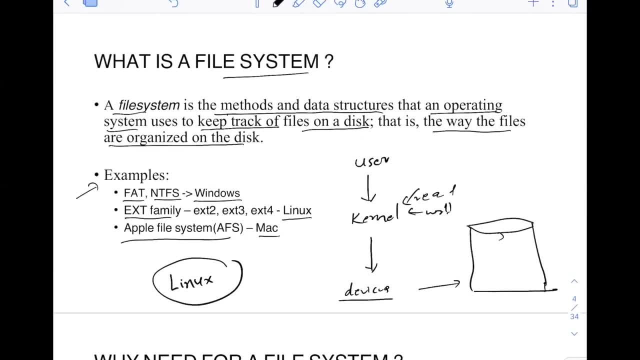 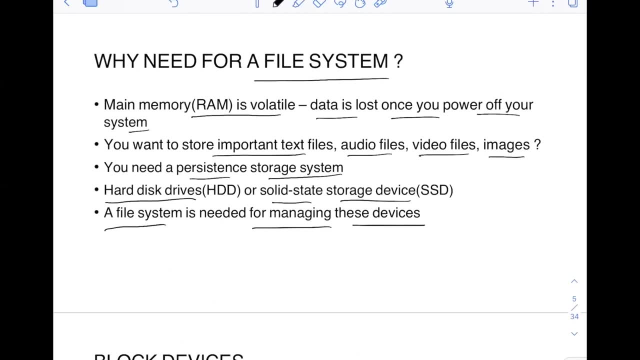 system. it's a hard disk drive, so it can manage all these devices, right. so that's where file system comes in. so five, six term is needed for managing these devices and all of these examples: right, uh and tfs, uh, fat, ext, family, uh, file system, side, afs, right, all these are. 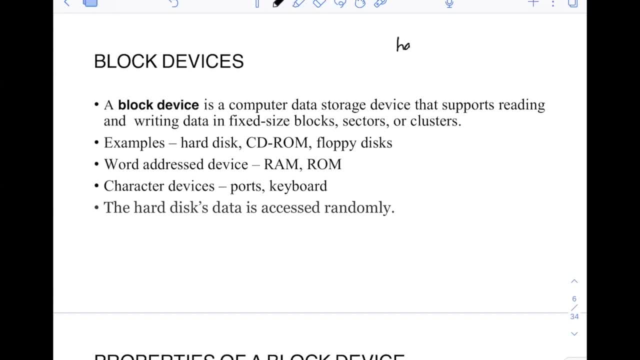 five, six terms which are used to manage hard these hardware devices. let me also discuss about blog devices. so till now i have discussed mostly about hard disk. okay, so hard disk. of course hard disk is one of the most popular. i will say i mean storage device, right where 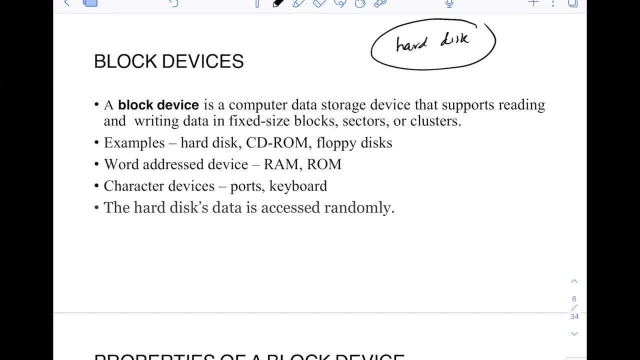 where you can store data permanently. hard disk is one of the popular one and, of course, hard disk is also one of the popular blog devices. i will discuss what blog devices is, but there are other blog devices also which can be used to store data permanently. a blog device is a computer data. 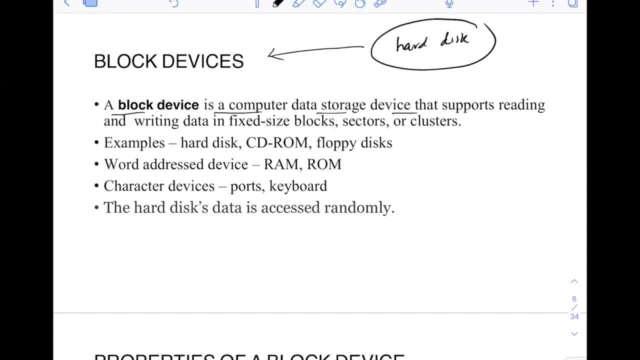 storage device. of course, it's used for storage purpose and for storing data permanently. that supports reading and writing data in fixed size blocks, okay, or sectors or clusters. this is very important in fixed size blocks, okay. so if you have to read or write to this blog device, you 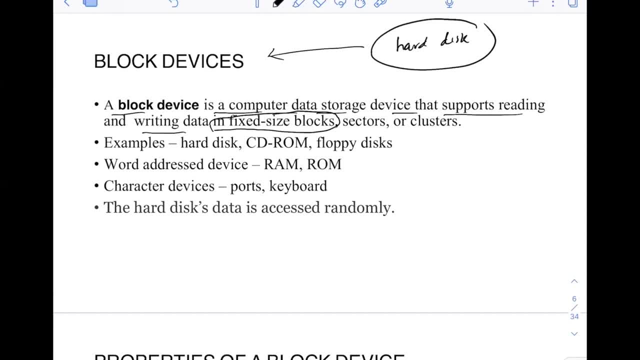 have to. i mean not you, of course. operating system has to do in terms of fixed block size. okay, of course you have other types of devices also, like word address devices, ram. we have already discussed ram and in ram, if we need to access data, you need to access data in terms of words. so a word is. 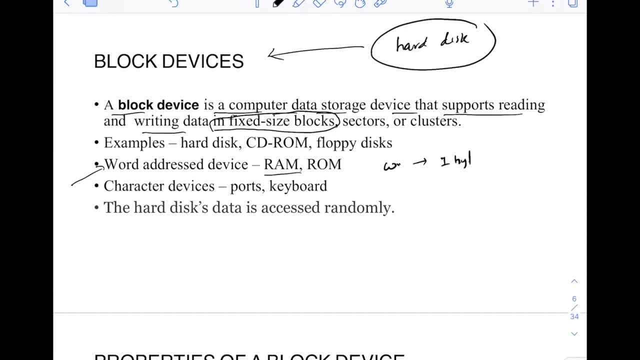 typically, mostly it can be like one byte to around eight bytes, so it can range from something one byte to eight bytes. okay, and ram and rom are examples of word address device. you also have character devices that are ports and keyboards. so here the accessing is done character by character, not by, not word by word. 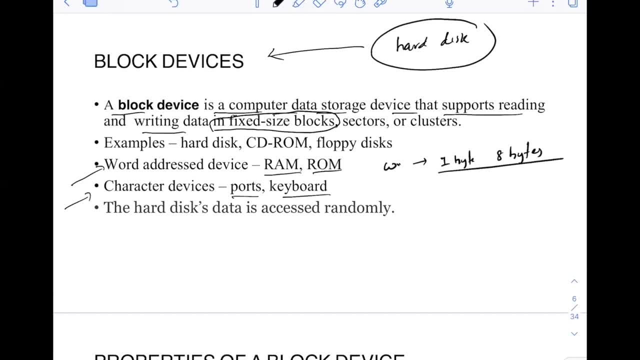 or not. block by block, it is done here by character by character. that's what happens in your keyboard, right, when you type character on your keyboard, that character is read right. probably some reads your data character by character. so in block device the reading or writing is done in form. 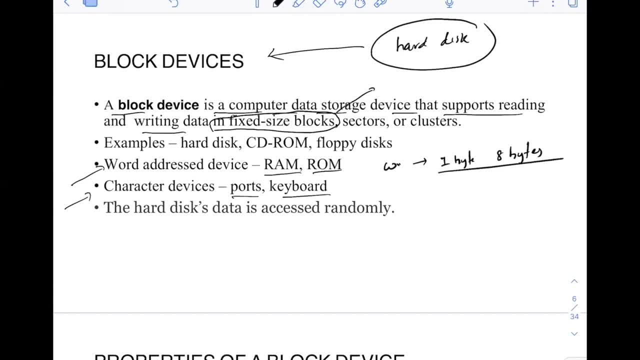 of fixed size blocks and there's this size of i am in. this fixed size block is typically very big, that is, around 512 bytes, and it can of course go greater than this also. it can start from 512 bytes and it can go maybe 1024 bytes, for example, right or more than. 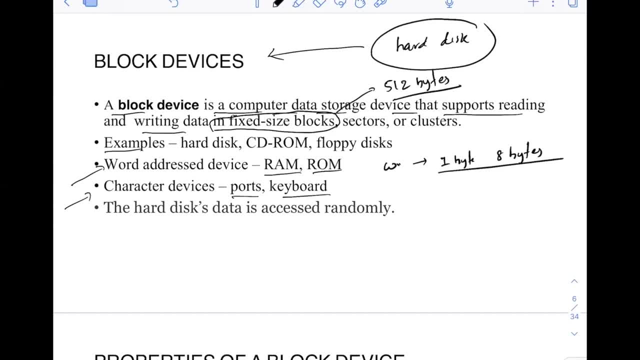 that also now, of course. famous examples of block devices are hard disk, a cd-rom. you would have used mcd-rom a lot during the old times now, nowadays, it's not. it's not used a lot. similarly, floppy disks also are not used a lot nowadays. also, the hard disk data is accessed randomly. 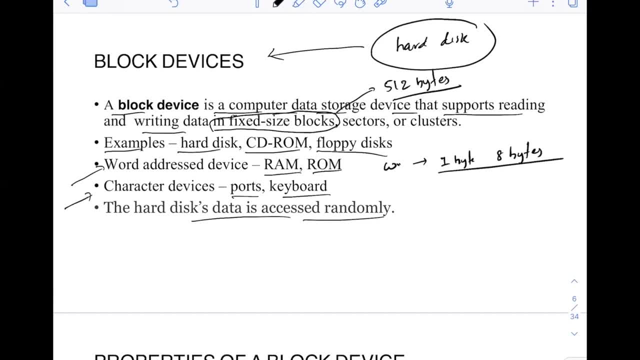 now, this is very, very important: like in character devices, what happens, the data is not accessed randomly. in character device the data is uh ordered by sequence, right? so when you, you know on your keyboard, right when you type w, o, l, f, right? so your operating system will read first w, then o, then l. 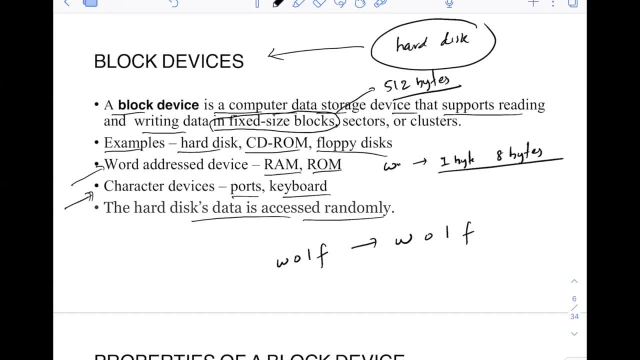 then f right in sequence, it will read uh in word address device ram and raw again. of course the operating system can randomly go to any position in ram. that's true. but in hard disk case is a bit different, because hard disk uh, as i told, the size of right, the size that uh. i mean that you. 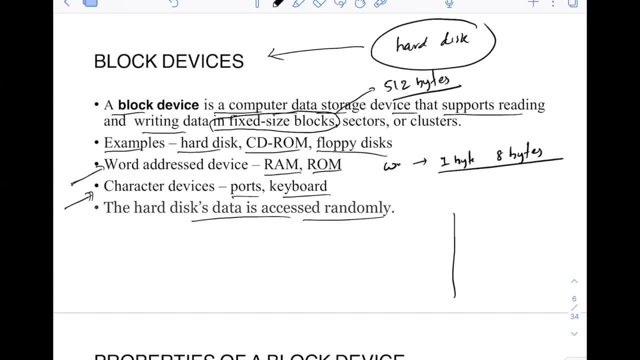 can access, right, is very big: 512 bytes. so basically let's say this is a hard disk. okay, now the data access can be something like: okay, first operating system needs data from somewhere here. the next time we need from somewhere here, again from here, from here, again from here, right, it's randomly from. 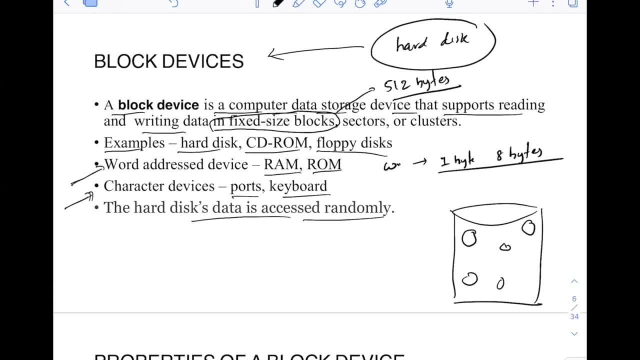 any position on the disk. that's why it's- uh, i mean retire access randomly. the same thing happens on on ram also. right same things happen on ram. sometimes candle will be accessing data from here, sometimes from here, sometimes from here, okay, from anywhere. but of course ram is very, very fast and here the 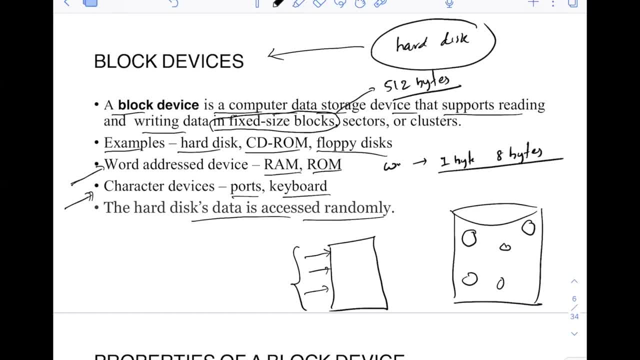 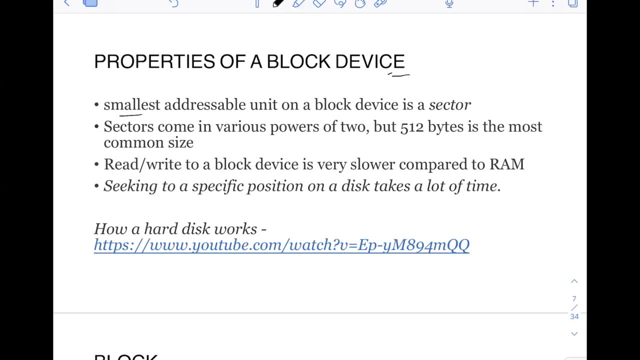 i mean you have word address device. ram is a word address device. this is like you have blocks, right? you have blocks here that also a big size, right, 512 bytes. so that's the main difference. i will do some more difference below, properties of a block device. so the smallest addressable unit on 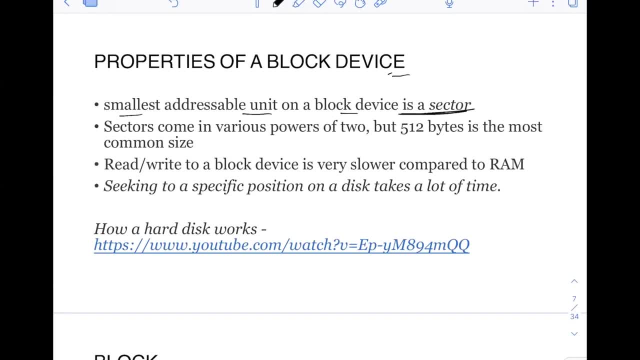 a block device is sector. okay, this is very, very important. this is i mean on a block device. the smallest unit like that you can- i mean access basically- is called sector. sectors come in various powers of two, but 512 bytes is the most common right. that's what i told, right for hard disk, uh, i mean like: 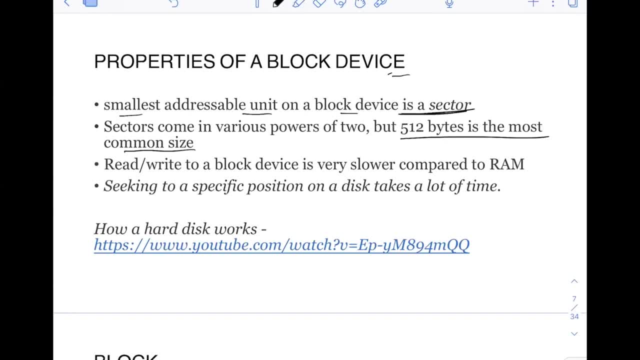 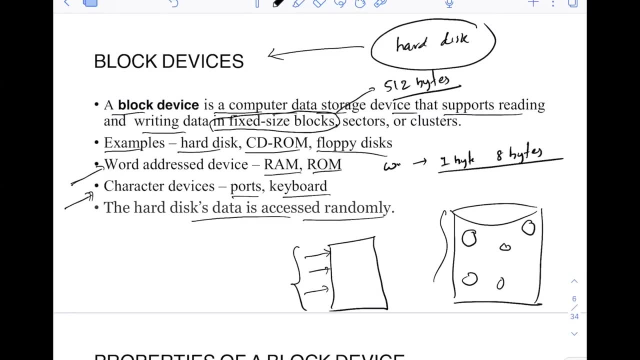 if you want to access right hard disk, you have to access, of course, in terms of blocks, and the most common size here is 512 bytes. okay, there's. there may be one confusion here, like why i'm calling this blocks. okay, i mean, what happens actually happens is in most of the books, or? 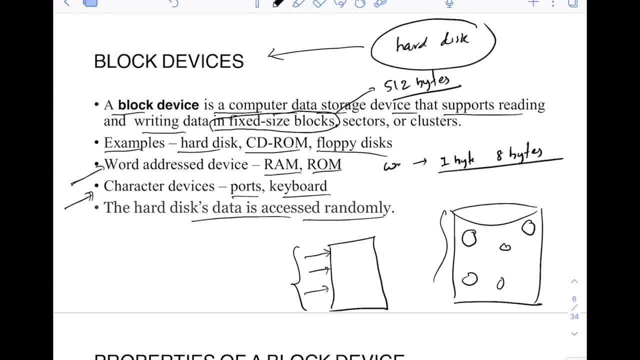 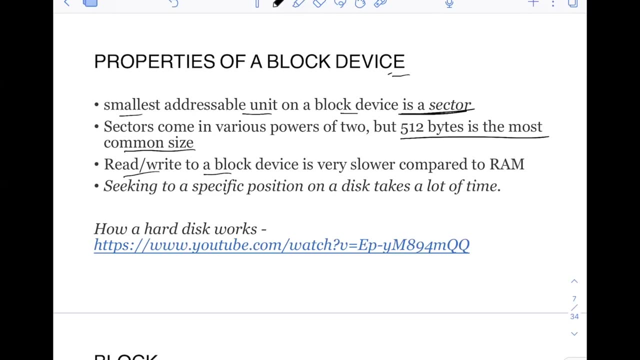 most of the context people will say: i mean people will use the words blocks and sectors interchangeably. they will not differentiate between these two. but of course there are difference. okay, that i will discuss a bit after, after some time. okay, so read and write to a blog device is very. 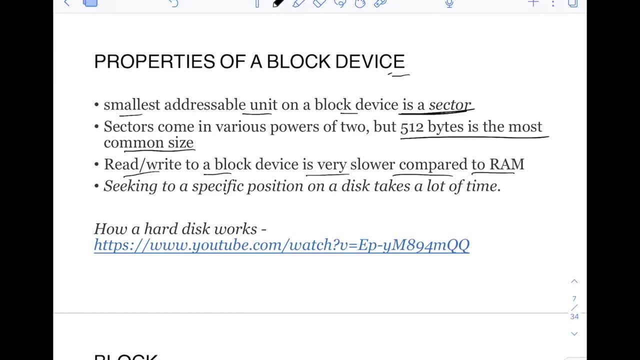 slower compared to ram. this is very, very important point. so when you are reading and writing to a blog device like hard disk, cd, wrong floppy disk- it's very, very slow operation and in ram it's very fast. for reading and writing to a ram it's very, very fast. now, what makes this block devices very 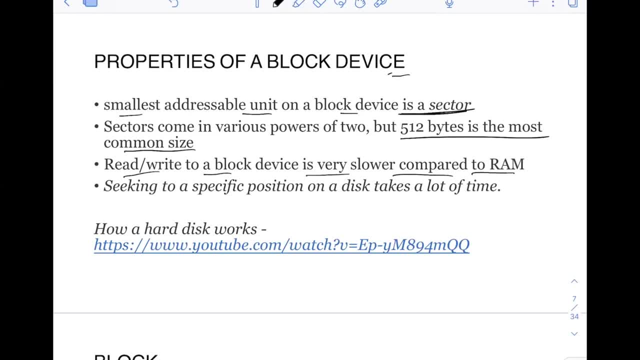 slow. one of the reason is that i mean let's say. i mean let's say, for example: okay, this is your again hard disk. okay now, if you let's say, if you want to write at this position, let's say, if you want to read or write at this position, so first the disk. uh, i mean the way the disk works. it has. 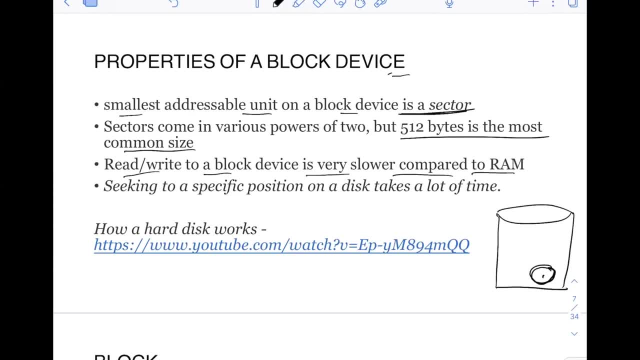 to locate this location, and locating this location itself takes a lot of time for the disk. that's not in case of ram. in ram it's very easy to locate any memory, but that's not in a block device like disk. okay, it takes a lot of time to just seek to one specific position and, of course, for reading or 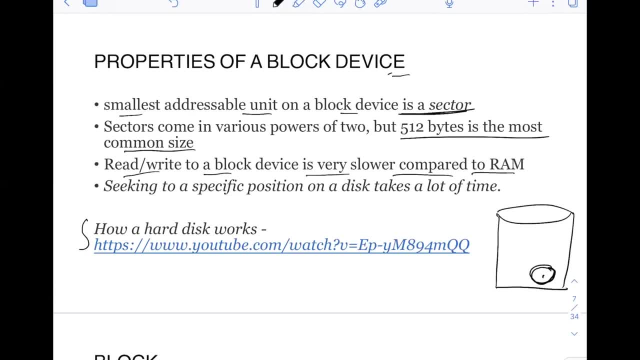 writing also it takes a lot of time, okay, and of course there is a video here. i pasted the link here. you can watch this and understand how actually a hard disk works. i mean you will see the concept of sectors, rotations and how i mean how hard this hard disk works. i mean you will see 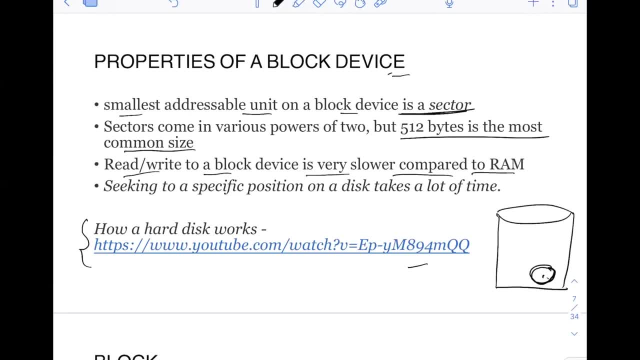 how a particular position is found and how it is written. and i mean read right. you will see that in this video i am not covered in. i'm not covering all those details in this video. now let's move to blog. okay, as i was telling you right in, i mean, in most context, people do. 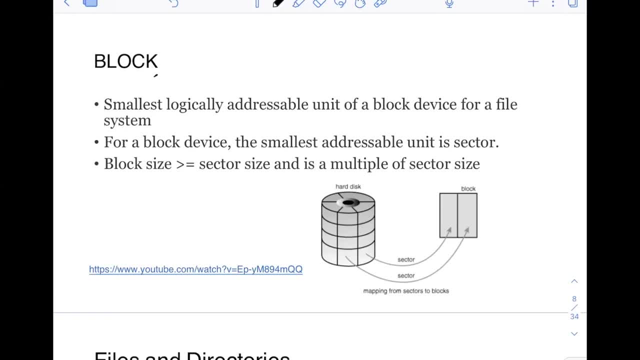 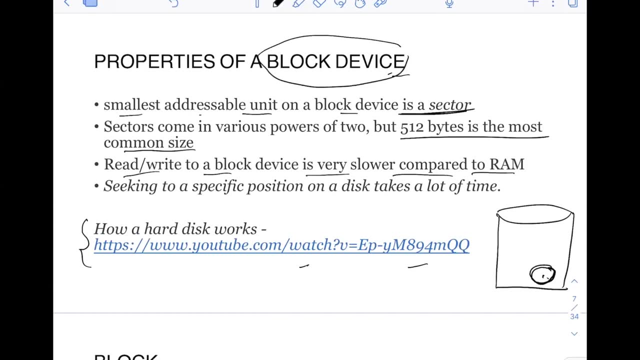 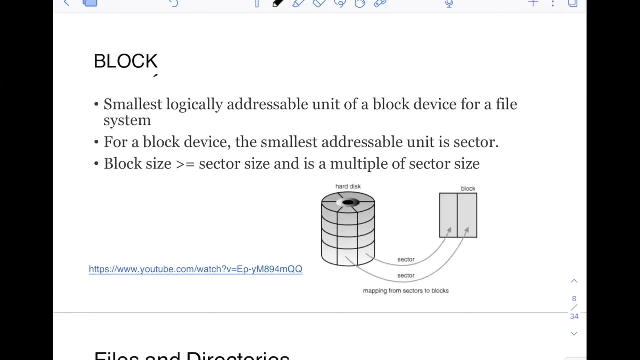 use blocks and sectors interchangeably. but there is a difference here. i told right sector is the smallest addressable unit in a blog device. so in a hard disk the- i mean the smallest, i mean addressable unit will be- will be called as a sector. now what is block? the smallest? 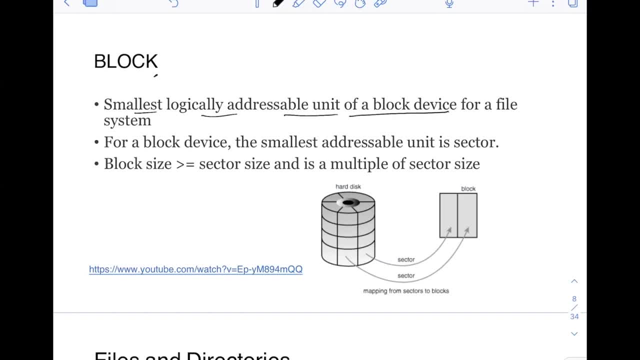 logically addressable unit of a block device. but we see, this language is important. of course, block is also the smallest addressable unit of a block device, but for a file system. okay, now for the disk itself. see this, see this diagram here for this hard disk itself, the smallest unit. 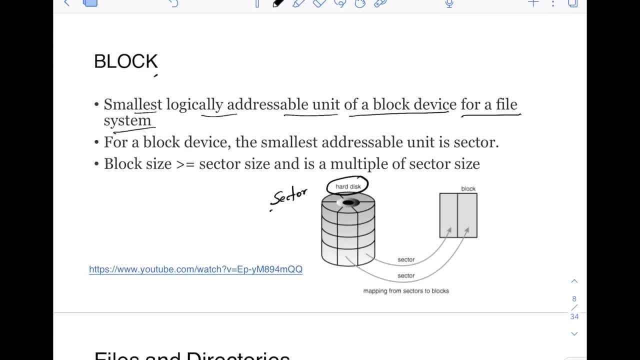 is called sector, okay. so whatever this hard disk will do, whatever operations it will do internally, it will always do in terms of sector, okay, whatever operations it does. so your file system will never see these sectors. they will, i mean this file, whatever file system you are using on your 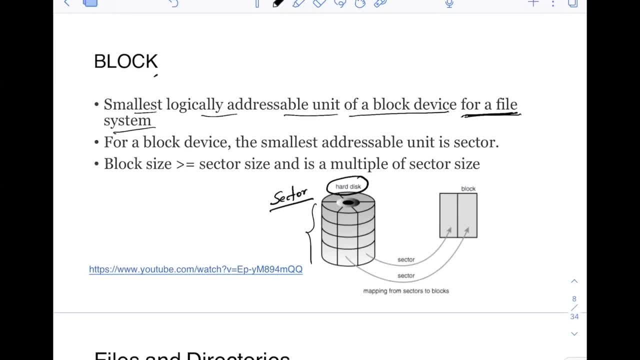 operating system. they will never see these sectors, and they will. they do not understand what sectors are. what they understand is what blocks are. okay, they basically haven't. so basically, i mean block and sectors are, i mean, quite same actually, but of course they are for different uh purpose. sector is used within the hard disk internally for its operation, and blocks are used. 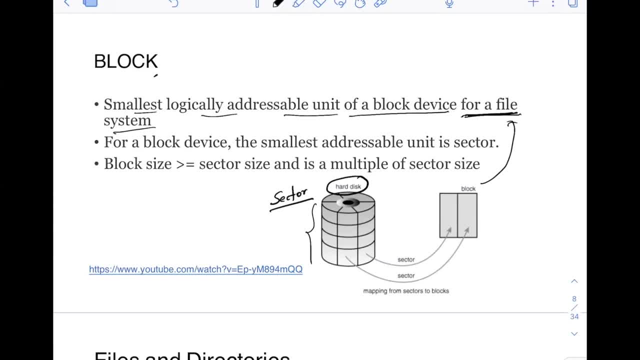 uh file system and of course there will be mapping between each sector to this block. basically, so you can again uh remember the concept of memory management. if you remember, in memory management the process has its own, like logical pages were there for uh, a process, right, the process memory. 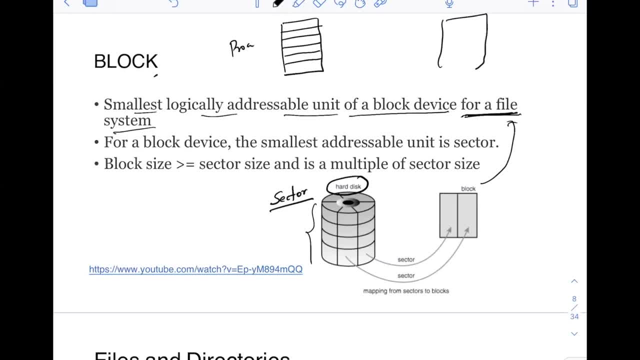 was divided into logical pages. and then you had main memory which was divided into multiple frames. right, and this logical pages where was mapped to some frame? similar thing is happening here also. so you have the sectors here in the hard disk. that is a part of the hard disk, again similar to the ram. 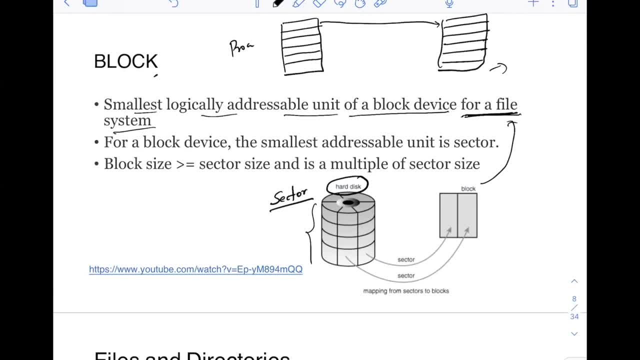 you have sectors here, and for the- i mean for the file system itself- it sees these sectors as blocks. okay, it will see that. okay, for example, this sector is kind of this block here, so different names, right. so whatever operations the file system will do, it will always do in terms of block. 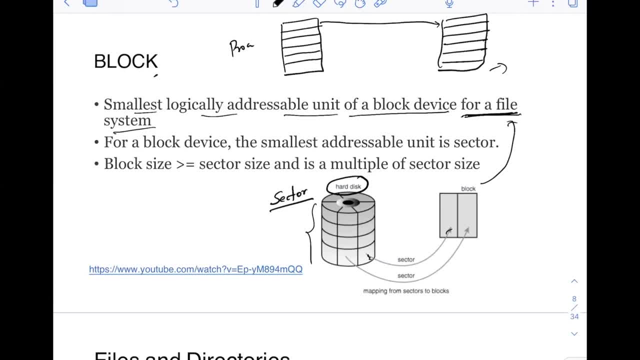 and of course, the operating system will tell, okay, that, okay, right to okay. take example of this, for example: okay, uh, you have a file. let's say, okay, that is all. let's say, maybe a thousand thousand bytes, okay, these are thousand bytes. and let's say each of this sector is of 512 bytes. okay, 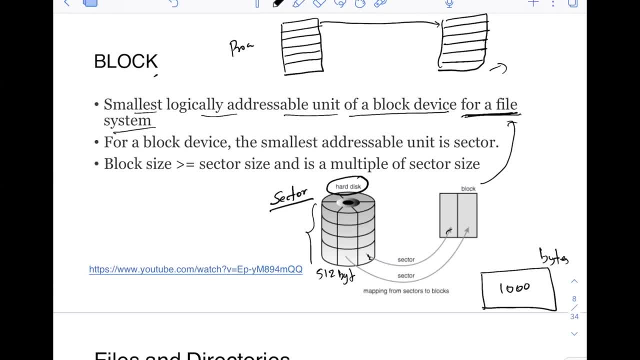 each of these sectors and of course, the block size also is, let's say, 512 bytes here. okay, now, of course, for storing this uh file of thousand bytes, you need at least two sectors or two blocks, right? so, of course, uh, the file system, what it will do, it will tell that. okay, right to this, this block. 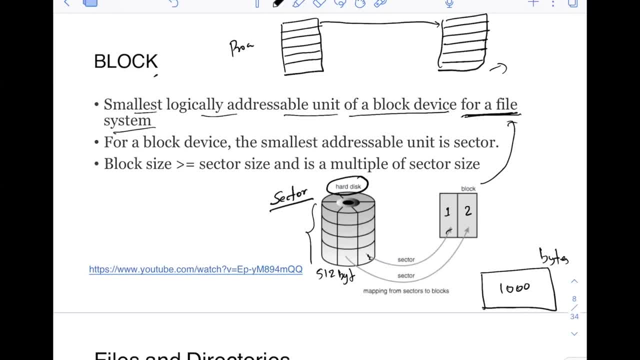 number is one, this is two. the file system will order the hard disk to write to these two blocks: okay, one and two, and then the hard disk will see that okay, these two blocks are basically mapped to these two sectors, so the hard disk will write to these two sectors. now for a block device. 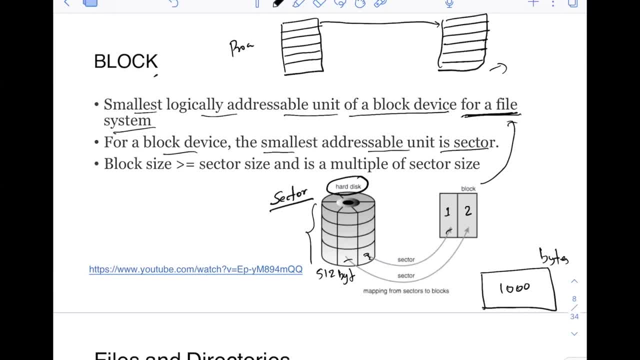 the smallest addressable unit is sector. okay, do remember this. this is a very important point. for a block device like hard disk, the smallest addressable unit is sector. but for a file system, right for a file system, the smallest addressable unit for any block device is: 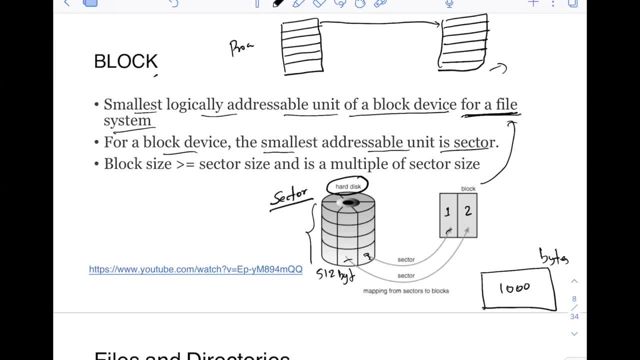 a block and there's, of course, a mapping between sectors and blocks. now the block size is always greater than equal to sector size and is a multiple of sector size. so if i'm in the common uh sector size, 512 bytes, so this block size will always be either equal to 512 bytes. 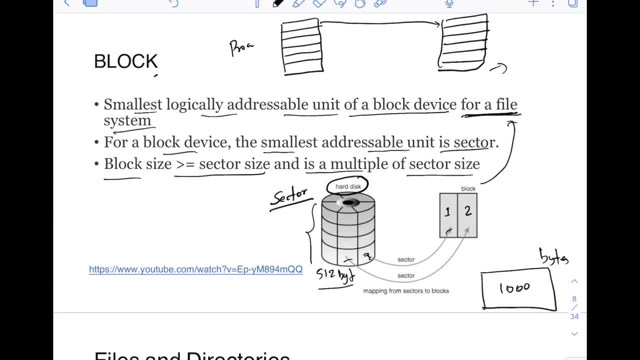 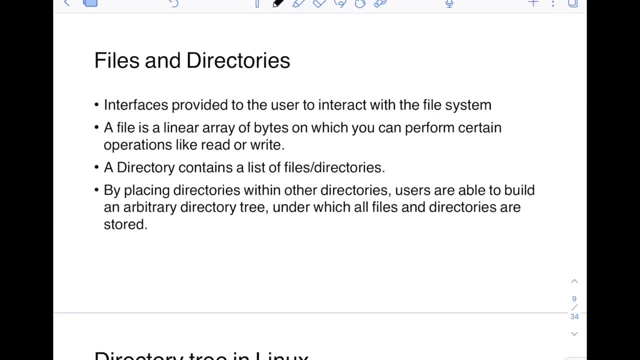 or maybe multiples of this. maybe it can be around 1024 bytes or maybe 2048 bytes in multiples of this. okay, so that was all about, uh, just understanding the basic concepts of what a file system is. examples of file systems: uh, what is different between sectors and blocks? right now we will. 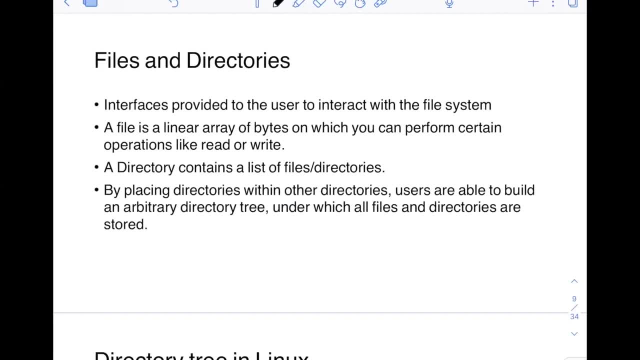 discuss more about files and directories that actually you use in your day-to-day work. right, whenever you are on your laptop or on your desktop, you do create files, you delete files, you read from files, you write to files, right. so we will discuss about those operations here now. what are files and? 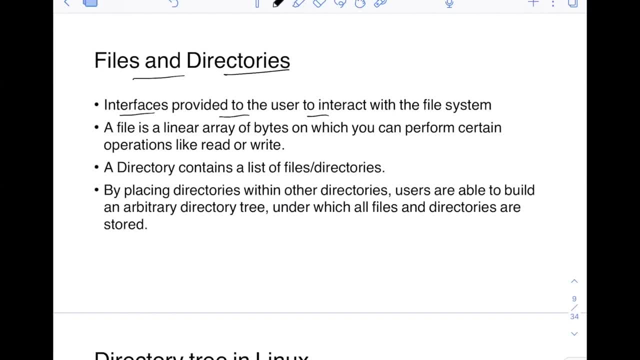 directories. so these are interfaces provided to the user to interact with the file system, right? so how do you interact with the file system? you interact with the help of files and directories. a file is a linear array of bytes on which you can perform certain operations like read or write. 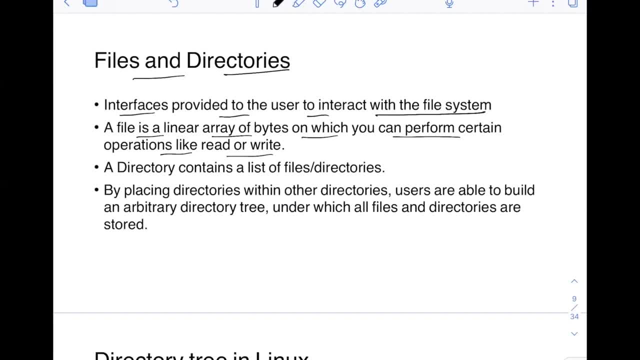 so of course, uh, whatever, your file is right. so it's a linear array of bytes. so in the arrow, some data is there. you are showing some data on the files. so what directory? a directory contains a list of files and directories, right? so of course you can have files, you can have directories in the directories, you can have. 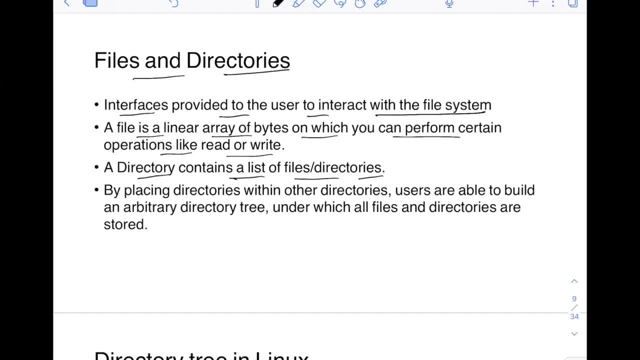 more files, more directory, and this can go on right. it's like a recursion, right. so i mean, let's say example, right, you have, i mean, one directory here. in this you can have multiple files, you can have a lot of files. now one one of this, uh, can be again that directory. in this directory you can have again. 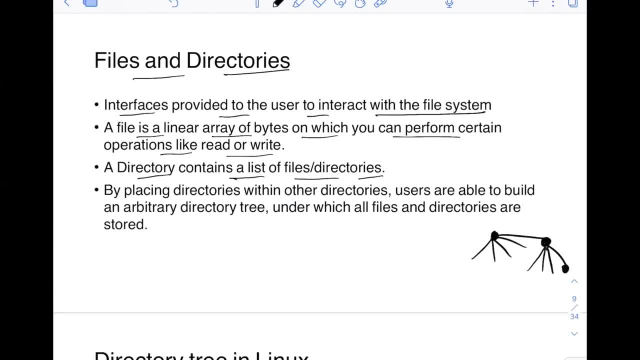 i mean more files and again one of this kind of directory- right, this can go on. similarly, maybe let's say this is also directory. there can be multiple files here, so it's like a recursive tree goes on. by placing directories within other directories, users are able to build an arbitrary 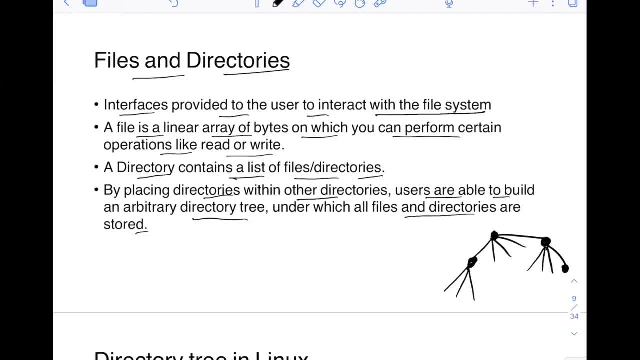 directory tree under which all the file directories are stored. that's what i was showing you, right, like users are able to build a kind of tree with the concept of these files and directories. now let's discuss about. as i told you initially, i was discussing mostly about linux open system. 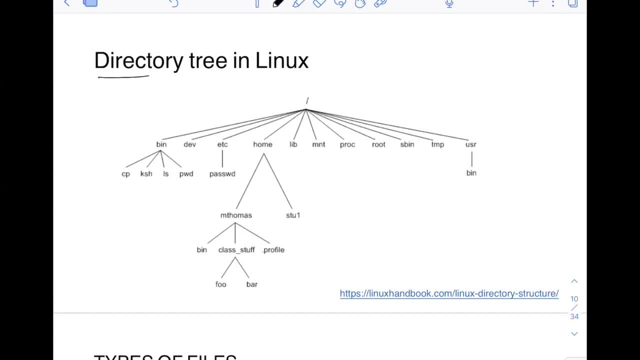 like file system in linux operating system. so let's see the directory structure, directories, tree structure in linux. so you have, of course, the root directory, that is, this is the root directory, and inside the root directory you have nine multiple different directories. important ones are been uh, dev, etc. home live, mnt, proc, root, sbin, tmp. 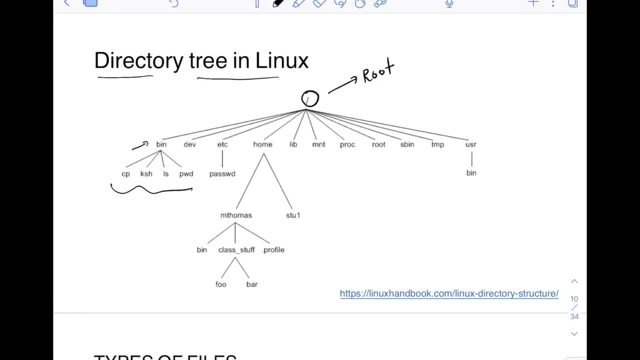 user right and in bin again you can have like different, for example maybe file sets of let's say right, like pwd, ls, ksh, cp. these are different files in bin. similarly in home, like you can have two different users, m thomas and s2, s2u1 and m thomas directory you can have again. uh, let's say 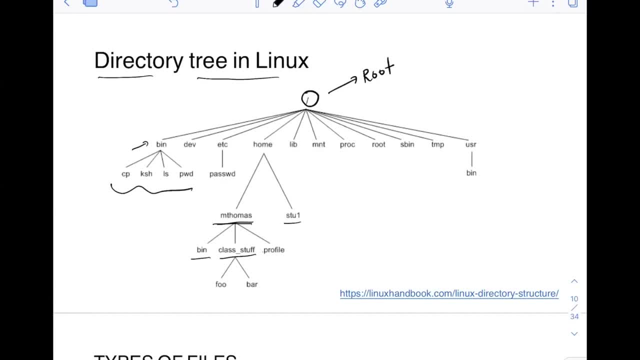 another bin directory, another class type, directory, dot profile, uh, let's say file, and again class stuff. you can have full file, bar file, right. so it's basically. uh, it's a, it's a directory tree, basically right, that's, that's what you see in linux and if you, if you, if you have used linux, 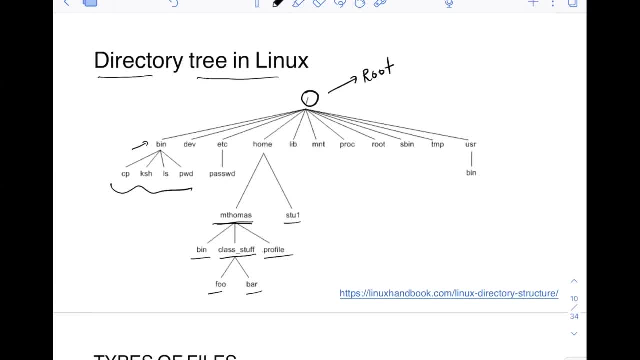 any of the linux operating system. right, you would have seen this, this type of folders in those and files in those, and of course i have a lot of files in those and of course i have a lot of files in this directory. i have pressure link here, like if you want to understand what is actually stored in. 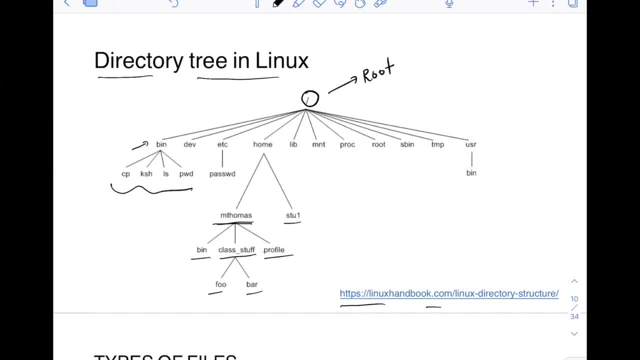 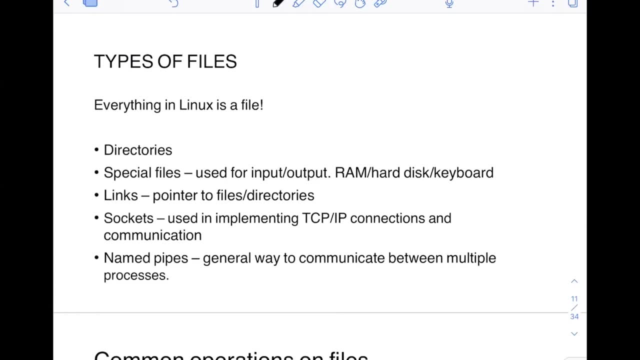 this, bin this, dev this, etc. you can read this link right. this will provide you a good idea of that. what are different types of files in linux operating system? now, this line is very, very important and this you will hear or read a lot of times. everything in linux is a file. 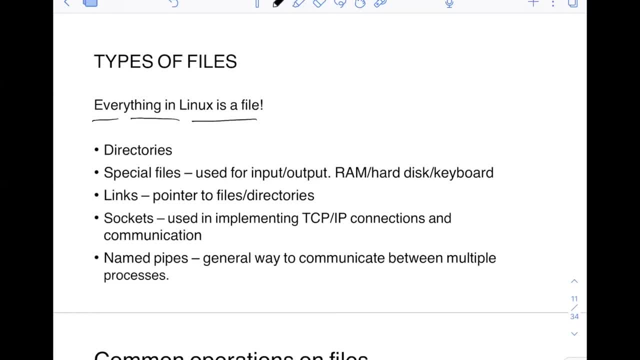 and that's right everything. basically. i mean even whatever your hardware devices are, right, even i mean the linux, right, your linux orbit system sees those also as kind of files itself. even your ram, it sees the ram also as a kind of file. all your hardware device, right, whatever you have, it sees them as file. your keyboard itself, right, it sees the keyboard as a. 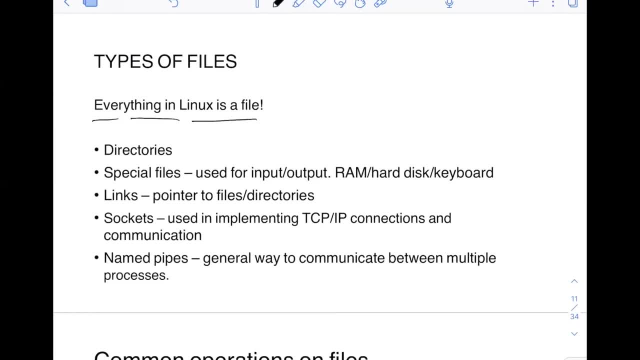 kind of file. so all the operations are done with the help of files itself in linux. that's why it's called: everything in linux is a file. of course different types of files are there. directories is also a special type of file itself. that you will see later on. so directories is also a type. 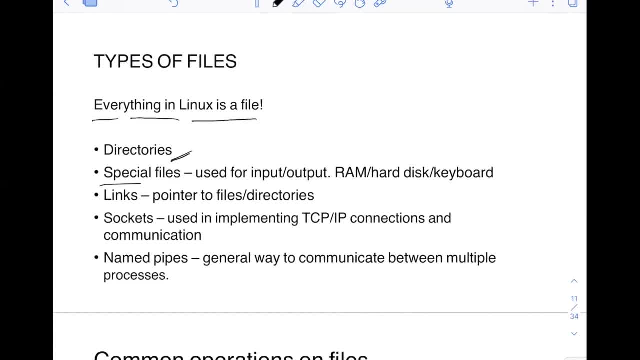 of file itself. in linux now you have a special file. you can see the directory is also a special files that are used for input output, as i told you right, everything like ram, hard disk, keyboard, all of these are uh kind of files itself. i mean all the operations through this right. so whatever. 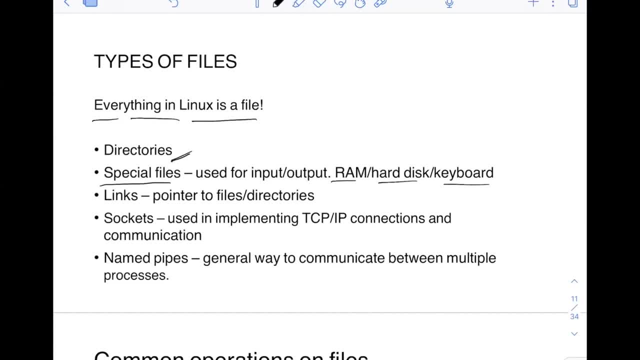 operations are done to ram, hard disk, keyboard. those are those. all are done through some files. so these are special files, basically because these are used for special purpose of input and output. then you have links, basically, so i mean there can be links also in linux, basically so. 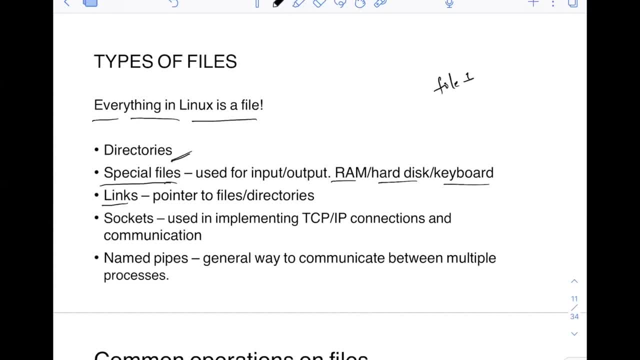 like you have. you have file one, okay, file one. there may be something like file two, okay, and this file to me pointing to this file one itself. so if you open this file, right, since this is pointing to file one itself, i mean when you open file two. 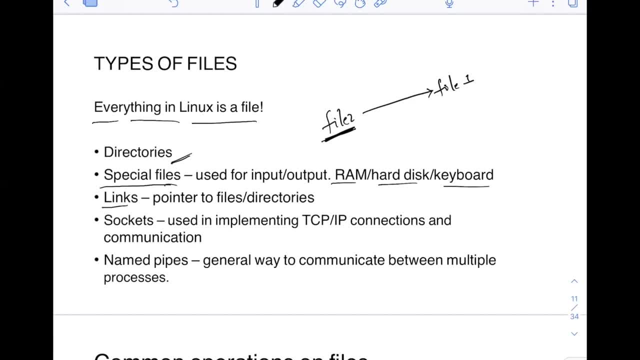 the file one, i mean you will see the content of file one itself, because this is pointing to file one. that is the concept of links, pointers to files and directories. then you have another important types of files called sockets. so even the network connection, right, that happens, uh, like, of course. 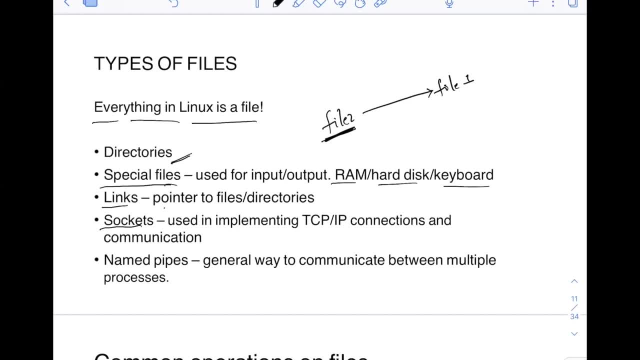 connection. that happens. those also helps. i mean it happens with the help of these files called socket files, right. so basically the communication that is happening right in tcp ip, that helps with. that happens with the help of socket files. the pockets are used for a special purpose of. 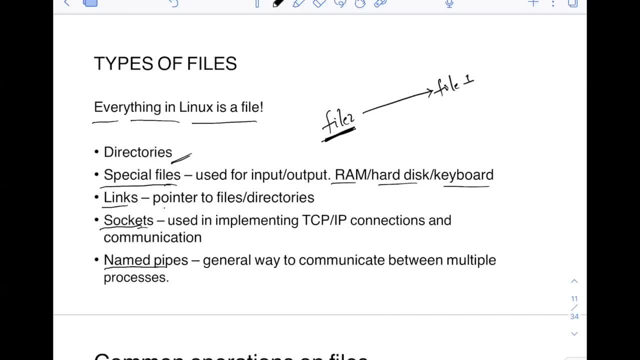 uh, communication in tcp ip. okay, so let's say, if you in mpcp ip you have one client here, right, one server here, and of course there will be client process, server process and they will be communicating right, basically using tcp ip protocol, and of course on the client side you will have some socket files, client socket files- on server you have. 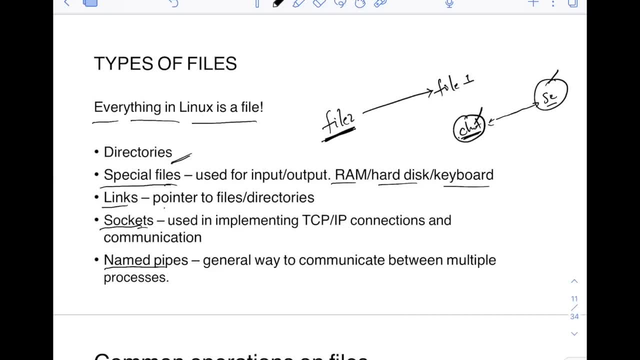 server socket files and those will be helping in the communication. so named pipes are a bit different. sockets are only used for tcp ip connections and communication. named pipe can be used for i mean different, i mean multiple other purpose. so if you want to process, are there right? 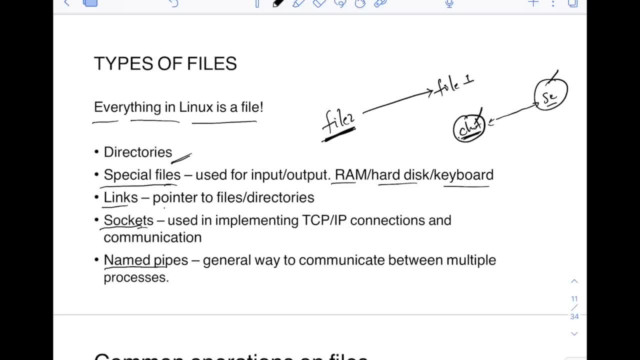 these are not client and server. these may be two processes on your system itself and if you want to communicate between these two processes then you can use. they use a named pipe and this is general way to communicate between multiple process. but sockets are not the general way. these are mostly used in tcp ip connection communication. 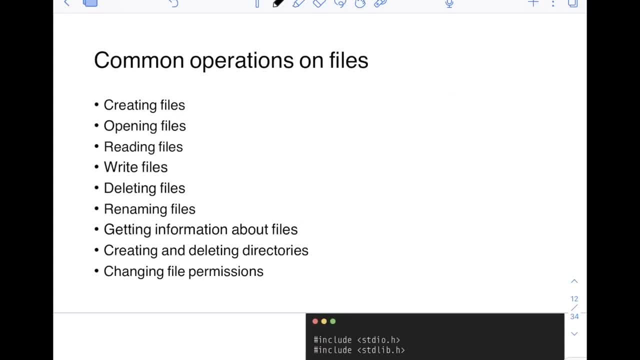 what are the common operations on files? so of course, you would have done this all like creating files, opening files, reading files, writing to files, deleting files, renaming files, getting information about files, creating and deleting directories, changing file permissions. so these are some of the common operations that i have listed here on files and you'd 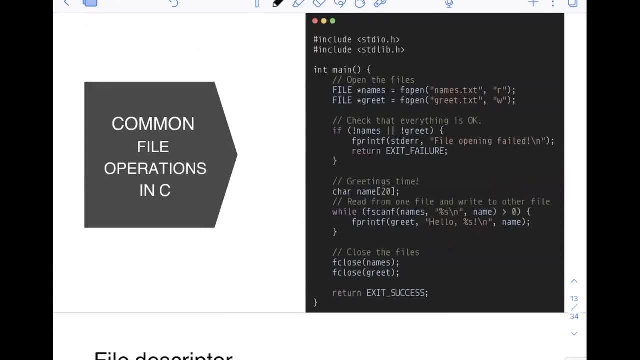 have done a lot of this already. let's discuss about common file operations. uh, in c. so i am just showing you a program here which is written in c programming language. and basically, how do you open a file in c? how do you write to a file, okay, how do you close your file? so all of these operations are done here. so what this? 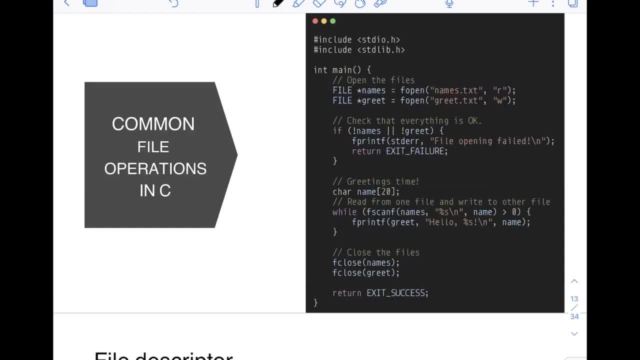 program is doing is so it has. i mean it is it has two files, names and, uh, i mean it is opening one file, that is namestxt. it is opening another file, readtxt. right, if you see here, let me change the color here. yeah, so you can see there are two files, namestxt and green dot txt, and and both are being opened. 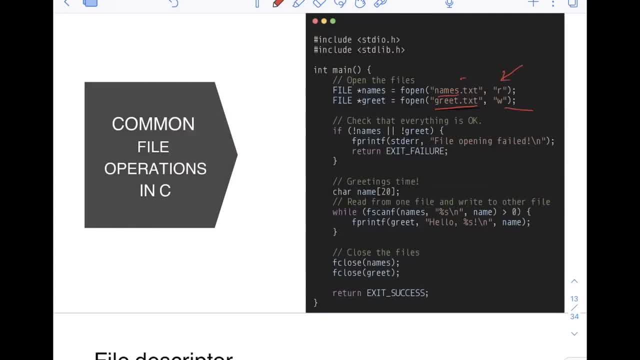 in this and one is used for reading purpose. r is here, one is used for writing purpose. okay, so basically what this program is doing is it is it is reading all the contents from namestxt. so whatever content content is there in namestxt, it will read those and then write those contents to this file, gridtxt. that is opening both of. 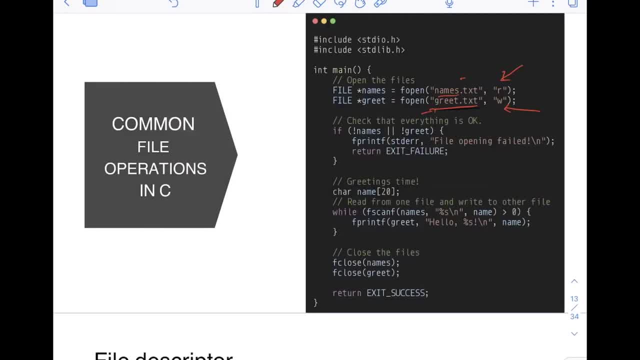 these files. so f open uh function you have in c for opening the files. so it is using that already, checking that everything is okay, and it is just checking that the files were opened correctly. if it is not, of course it will uh give some error like file opening failed. okay, now let's. 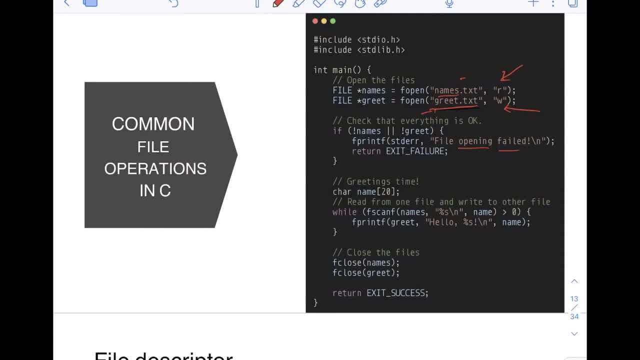 say that the both of files are opened successfully. what happens after that? what basically? uh, the program does it. it has just created this uh character name 20, right for storing some data. okay, now you see this f scanf is there right f scanf here. so f scanf is used for reading data. 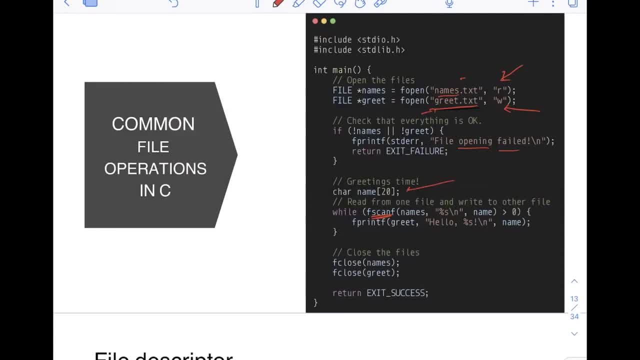 from the file. so it is reading, uh, from this names, right, this names, this test. so basically, now i'll be referring to this file with this names pointer- that that's what i've used for opening that. so it is reading from these names here. so it is reading all the data from names here and if you see it is. 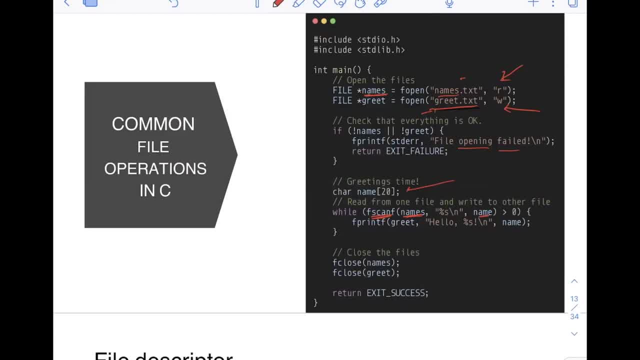 storing in this name variable here whatever data is there, of course it will be line by line, okay, and then it will write to this file: f. printf is used for writing, so it will write. whatever data is there, it will write greet and grid is, of course, if you see it is used for this gridtxt file, the reference grid, right, so it. 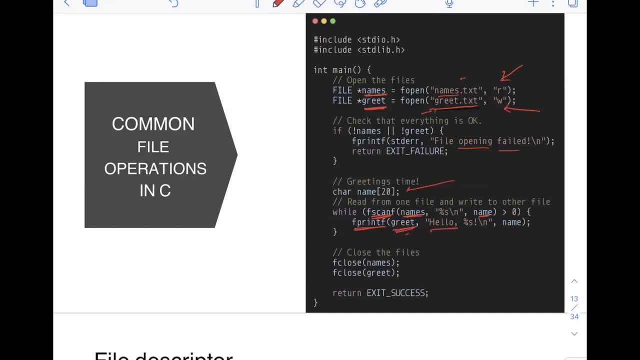 will write to this uh, gridtxt file: hello and whatever is i mean. i mean models, as is there. basically, it will replace what is here in this name. so of course, let's say, if this names or txt contains shivam, okay, and then let's say ravi, okay, that these two names is there in this. 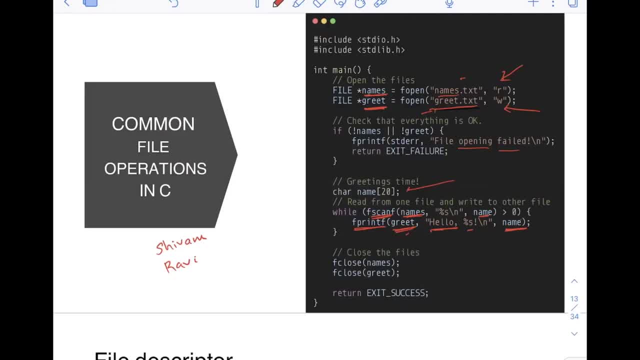 namestxt. so in the first f scanner it will read, because it is in line by line. it will read she um and it will store this in name variable. okay, then in the next line it will. so it will go to another file, gridtxt. okay, let's say this is the file gridtxt. it will write to this file that it 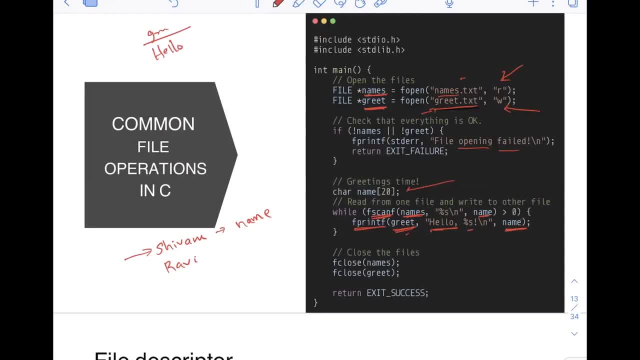 will write hello first, okay. then followed by whatever it has read from this first file. so hello first. it will be shivam here, okay. so again, a second time it will be ravi and write hello. and now, since there are no contents here, because if you're only checking, greater than zero, right, whatever it is reading is greater than zero. but 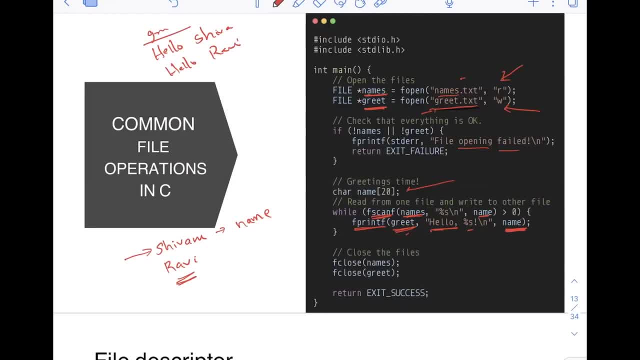 of course, after this there are no contents. so this will not be satisfied and control will break from here. and finally, what? and we are done with what we wanted to do, so we will close both of these files with f close, come, f close, uh function. so we have closed both of these files. so here are some of the 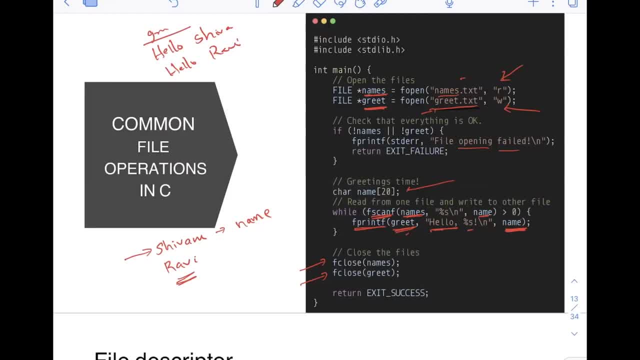 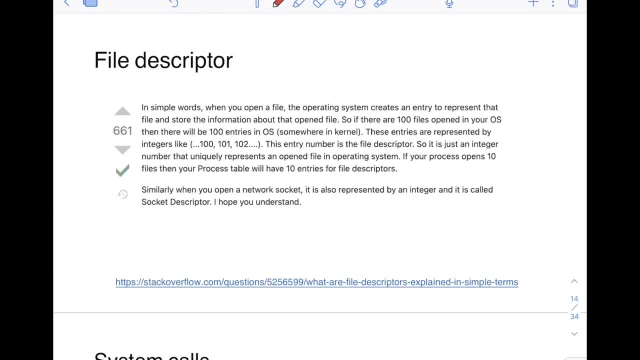 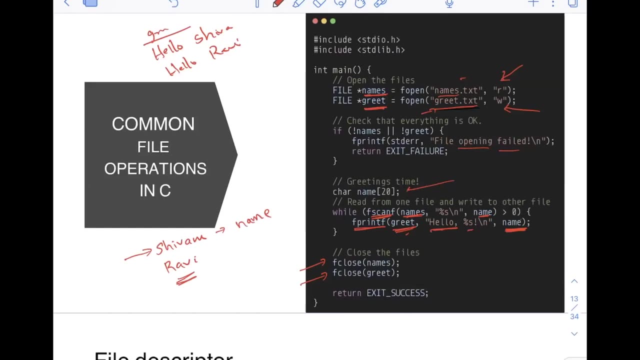 basic operations. uh, uh, i mean what and what you can do in, uh, c language, programming language. now let's understand the concept of file gridtxt, file descriptors. the reason why i am- uh, i am going to explain- file descriptor is that so, when you are opening these files here, right, these files, names and grid, so what actually? 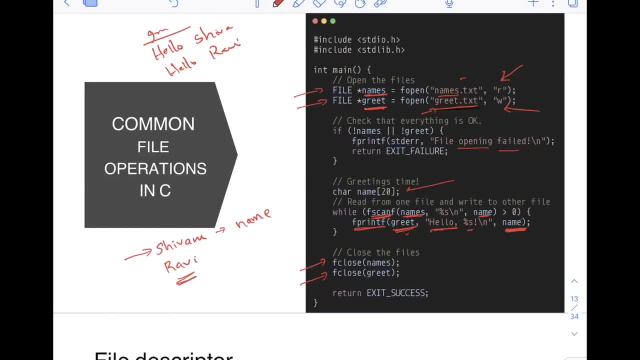 happens is that a new file descriptor is getting created and that's what is getting returned here, right? this names pointer will be pointing to that. so one uh file descriptor will be created here for this f open command and these names will point to this one. okay, similarly, another file descriptor. 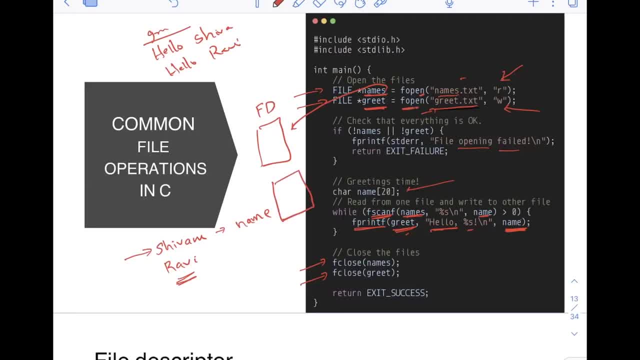 will be opened for this open f open command and this grid will then point to this one. okay, so that's why understanding file descriptor is very important and even if, when you are closing this right, uh, file descriptors, you see these names and grid are basically file descriptor, and when you 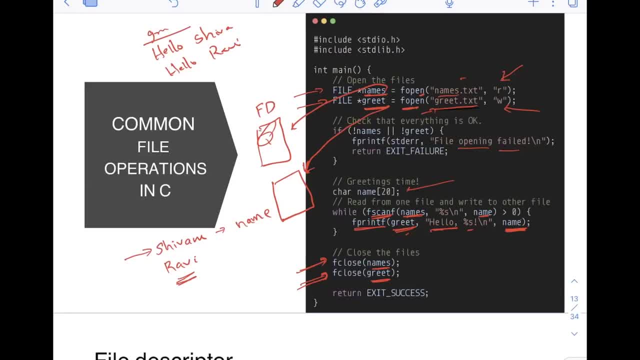 are closing them. i mean this basically. basically, kernel has allocated some memory for this file descriptors, right, so they will get destroyed. basically, these file descriptors will get destroyed when you close this. and if you do not close this, you know what? and there are issues, right. basically, you are not, you do not want to use this, but this file descriptors are still open. that is wrong. 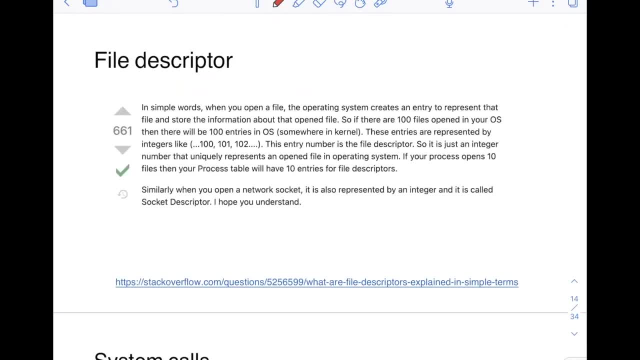 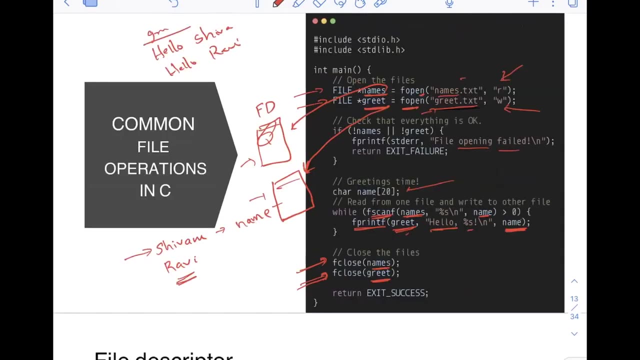 basically so what is file descriptor? so this i have copied from a stack workflow answer. in simple words, when you open a file, the operating system creates an entry to represent that file and it store the information about the open file. that's what i told you, right? whenever you open a file, some data structure is created for storing information about that file. 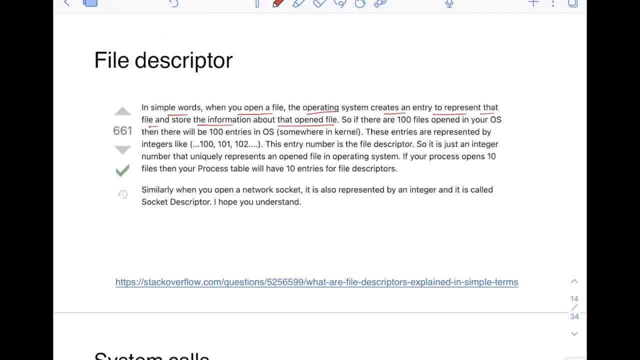 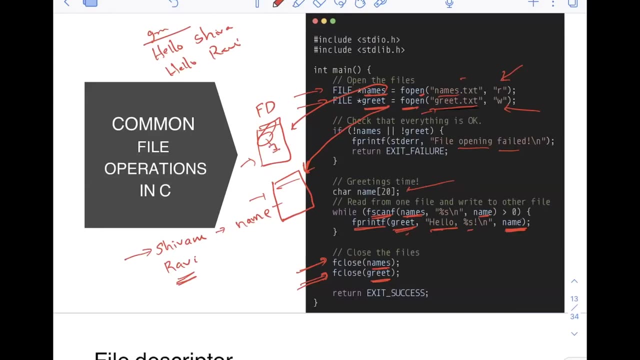 right, that's. that's data structure is basically your file descriptor. so there are 100 files opened in your operating system. there will be 100 entries in os somewhere in the kernel. these entries are represented by integers, so basically each of this file descriptor will have a unique id. so let's say this is one, this is two, just an example here. 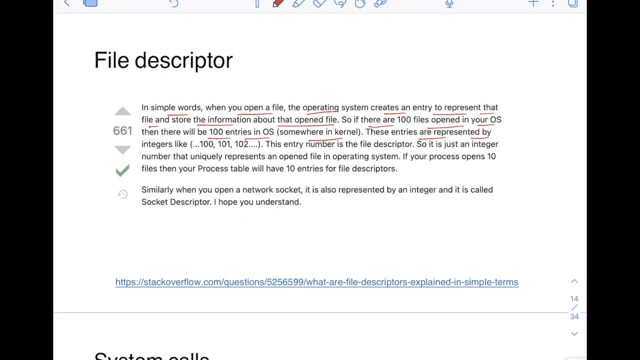 integers like one zero one. i mean one zero one, zero one zero two. like this entry number is the file descriptor here, so it is just an integer number that uniquely represents an open filing operating system. if your process opens 10 files, then your process table will have 10 entries of for this file descriptors. so do remember file descriptors are very important. 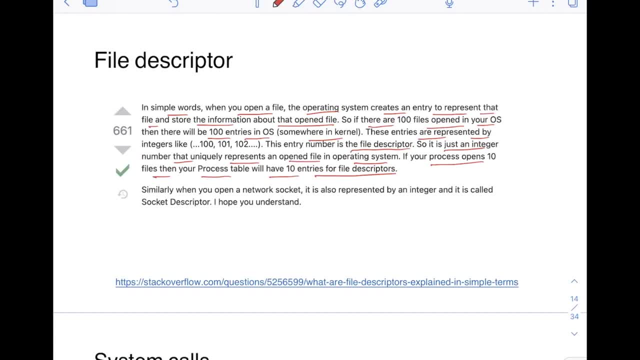 whenever you open a file, a new file descriptor is getting created to store a lot of data about those files and, of course, each there is a unique number associated with this file descriptor. similarly, when you open a network socket, it is also represented by integer and it is called: 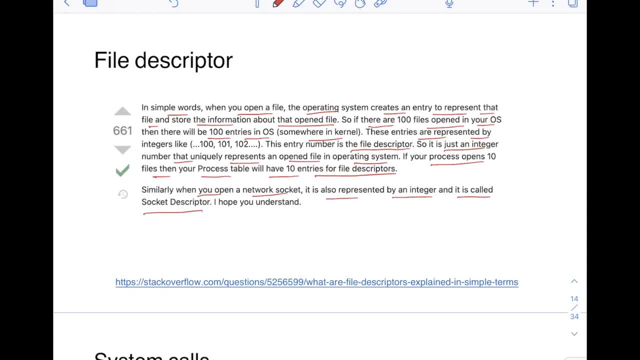 socket descriptor. right that i have that, that i have covered networking community working about sockets. so whenever you create sockets, a socket descriptor is associated with a socket descriptor with that, but here you have file descriptor now. okay, let's understand this again. so now another another reason for taking this example of this c program was that you understand that okay. 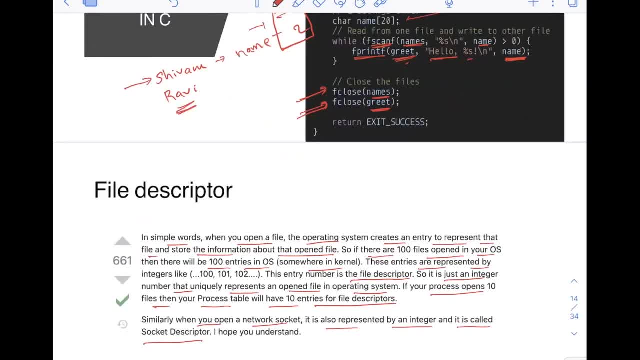 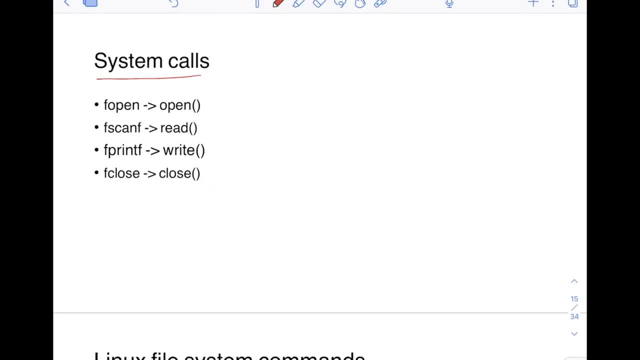 what this f open is, what this f close is right, but you also understand that. okay, what is the exact system call? they are calling on the background. so when you are using f open in your, in that program it is actually called calling the open system call. so open. 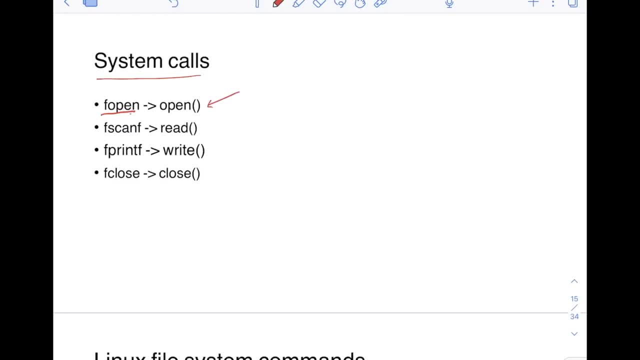 system call is used. uh, of course, this is implemented in the kernel itself and this is used for opening a file and app. open is basically kind of a library function that i'm using. right, this is the kind of library function that i'm using in your c code and this, open, is actually the system code. 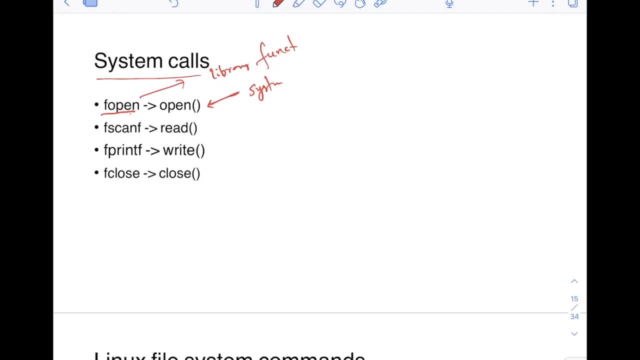 that actually helps in opening the file. similarly, for f scan up, you are using i mean the read system. call for f print up: you are using write system. call for f close: you are actually using close system call. okay, do remember the difference between library function and system cost. 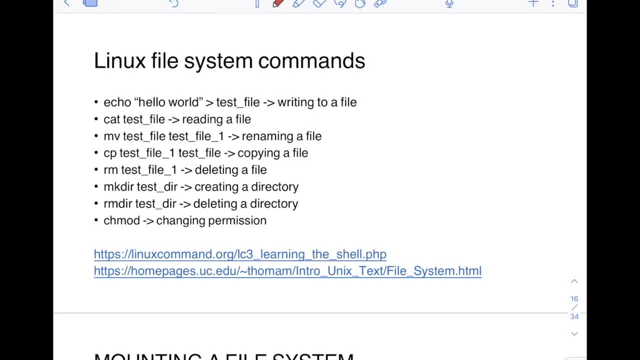 okay, now in linux. uh, as i told right in this video i will discuss most about linux operating system, so i will discuss also some of the important commands- uh in i mean- that are associated with linux file system. like, i have written the commands here, but what i will do is i will 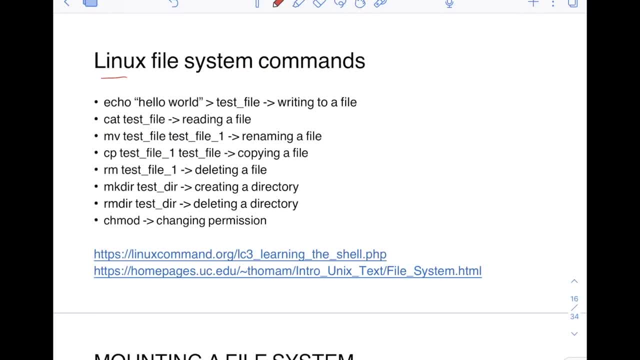 show this uh demo right on the shell itself. uh, so that you can understand these commands, what they actually do. okay, and of course, i have some reference here at the bottom also that you can use these commands in details. you can use that, okay, so let me go to a shell and try to run this command. 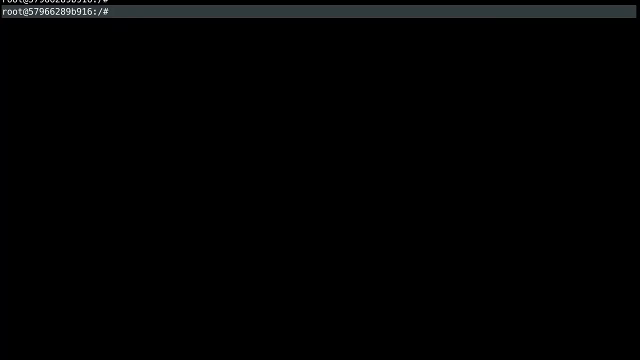 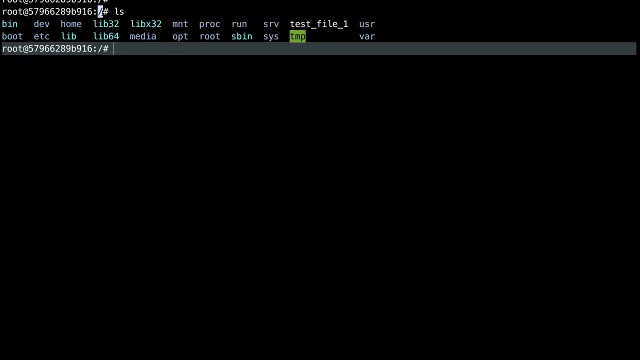 so now i am in a linux shell here, so what i can do? first i can run ls command. okay, so you can see right, at present we are in the root directory. you can also verify that using pwd, so it will tell you what is the present working directory. so you see, the answer is root. so basically you are currently. 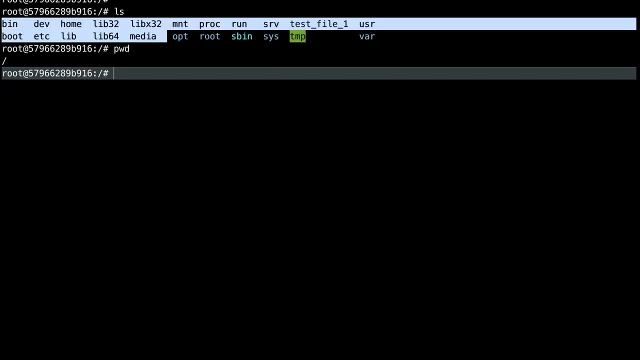 in the root directory and in the root directory these are the list of directories and files that are present here and that you would have seen in the diagram. i have shown that the linux directory right the same thing. same types of folders were there and directories were like bin, dev, home, all. 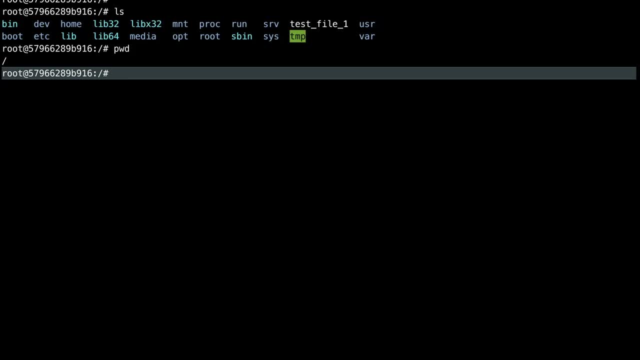 of this, right, and then i can go to some other directory, like i can do cd, okay, and then i can go to maybe, let's say, home directory, right, and i can list it here. of course, in my home directory there is nothing. there are nothing here, right. 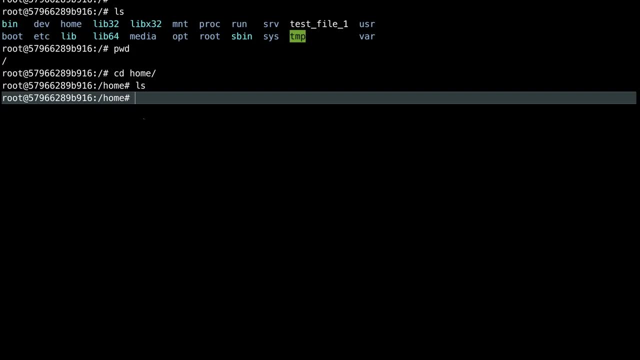 so what i will do is i will do some operations here in my uh home directory. okay, i will do all those file operations. so first i will do uh, what i will do is i will write to some file so i can use your echo command. let's say i want to write hello world to some file. let's say test underscore. 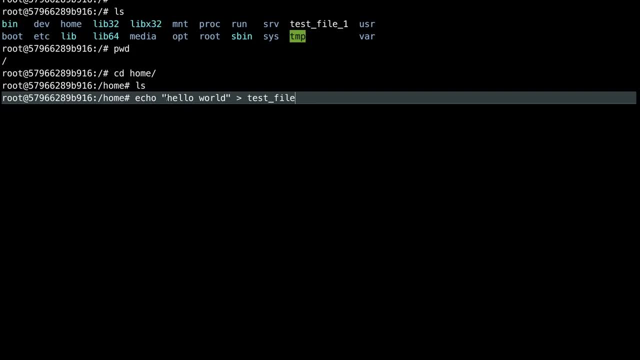 file. okay, so here what i am doing is: i am, i want to write this hello world right, and i want to write this to the file name called case underscore file. i am using echo command if i press enter. so, uh, now this is done. so if you do ls here, ls is used for listing all the files and directories. 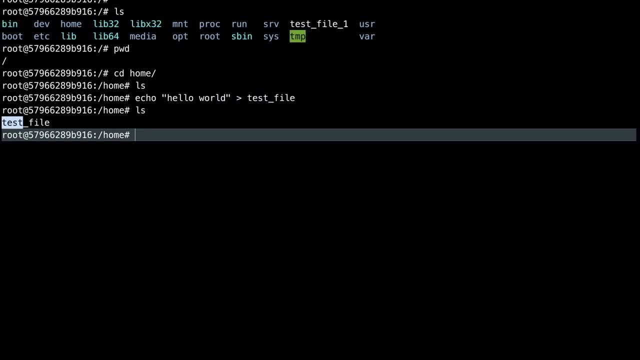 here so you can see a new file has been created- test underscore file- and if you want to read the content of this file, you can use cat command and if you use this, you should be able to read the content. that is hello world. that's what i have written here right. echo hello world to this. 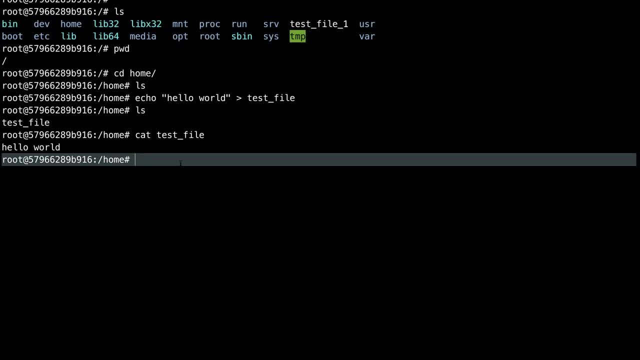 file. and now i can read this. now let's say another operation. let's say i want to rename this file- okay, test underscore file. to test underscore file, underscore one. then i can use move command mv. okay, just by, just by, uh, underscore one. so i'm basically trying to change the name of this file from this. 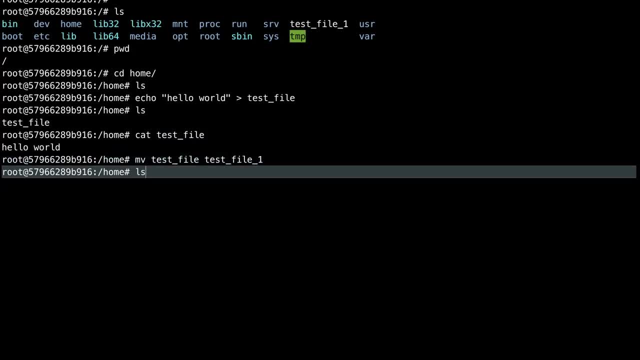 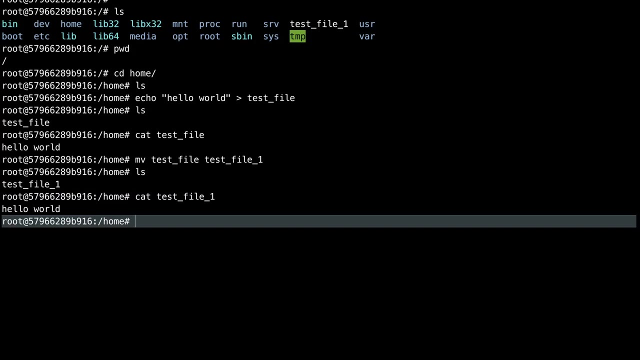 to this. if i press enter now, if i do ls now, you see, initially the file was just underscore file. now it has been renamed to test underscore file, underscore one. now again you can cat this file and after that you will see the same content as hello world. okay, now let's say you want to make a copy. 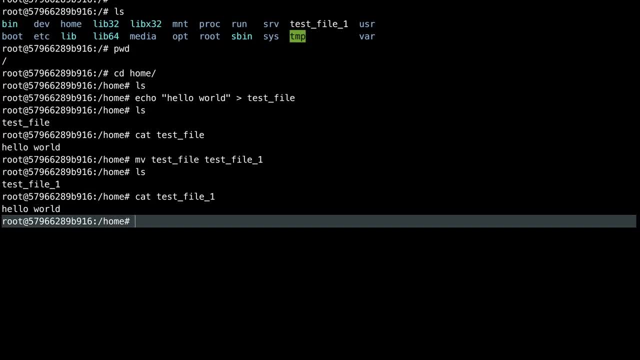 of this file. okay, i want to make one more copy of this file. what i will do, i can use cp command for that, and okay, uh, yes, and let's say i want to uh. so of course i will not uh name this second file the same. so the copy i am making. okay for this file, test underscore file and it's called one. 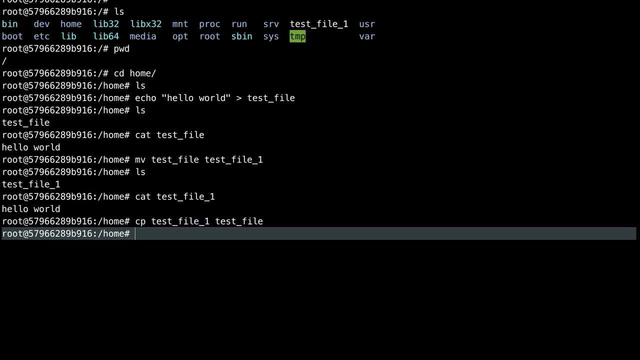 the copy name will be test underscore file. okay, let's run this command now. do ls. now you should have two files, because now we have made a copy of test underscore file, underscore one. that is test underscore file. so we have two copies there of the same file. but if you do cat on test file also, you should see the same content of hello. 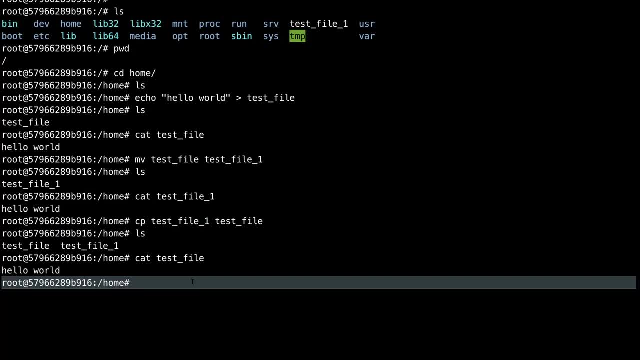 world there. okay, so basically, using cp command, we have copied uh data from one file to another. now let's say, if i want to delete this file now, test underscore file underscore. when i need to delete it, i can use rm command for this. if i use rm command, press enter now. if i do, ls now, you see this file has been deleted. now you 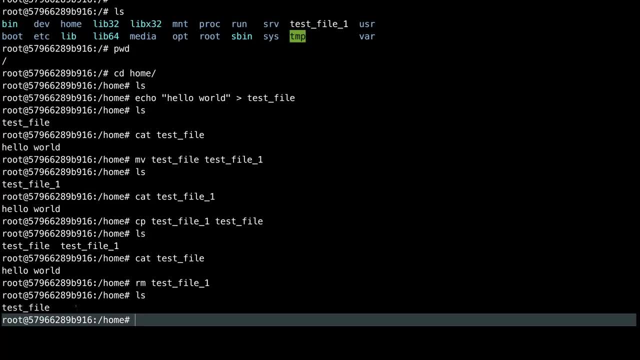 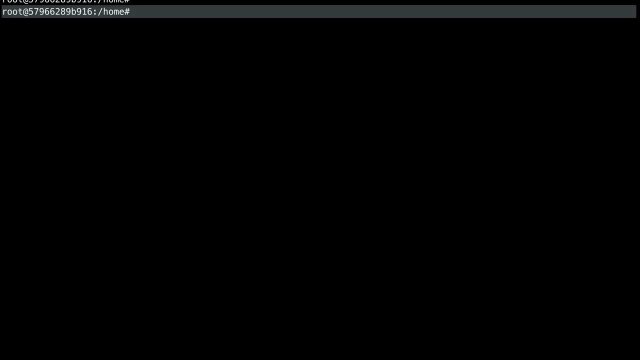 have only one file remaining, that is test. underscore file here, test screen. okay, this this were mostly for like file operations. now let's say, if you want to create one directory, let's say, right, you want to create one folder so you can use mkdir command. and let's say test. 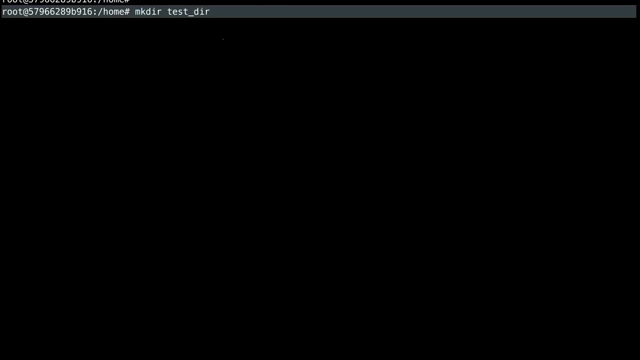 dir. i want to create a folder and let's say test dir. i want to create a folder and let's say test underscore file and let's say test dir. i want to create this uh directory called test underscore dir. so you may press enter and do ls here. so you see, there is of course the test underscore file. 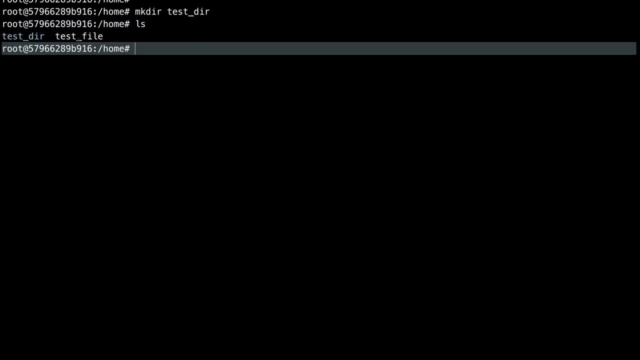 here and, of course, i have a new directory here. okay, and do remember, you cannot create a directory, uh, with the same name, right? let's say, test underscore file already exists in this, right? so if you try to create this, i mean a directory with the same name. let's see what happens. 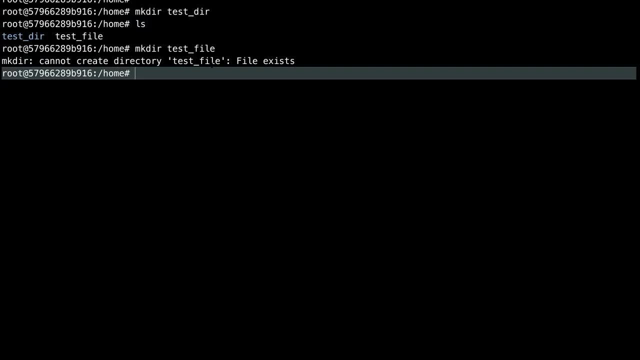 it gives an error that uh cannot create a direct test file exists. the reason is that linux sees both directory and files are same. i mean like both are files for linux, right, and you are trying to create two files with the same name and that's not allowed. basically, that's what uh is the error here. now let's say: uh, you want to delete this. 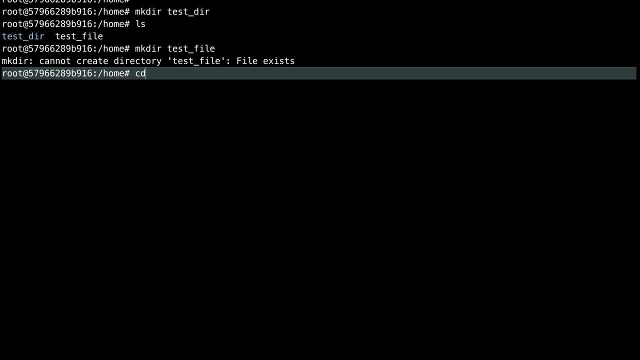 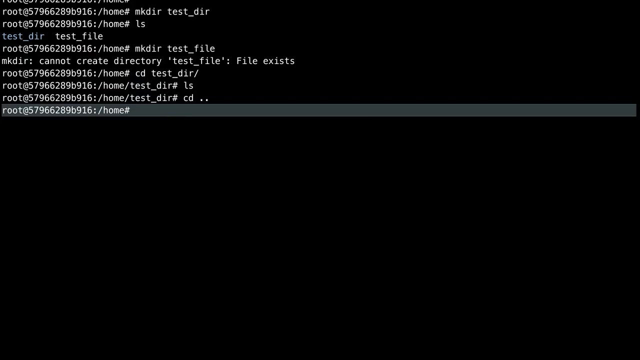 of course we have created this directory and you can again go to this directory using cd command. you can go to test underscore directory inside this. of course there is nothing here. right, i will go back again, uh to, but i i'm from wherever i came from: slash home now. what i will do is i will 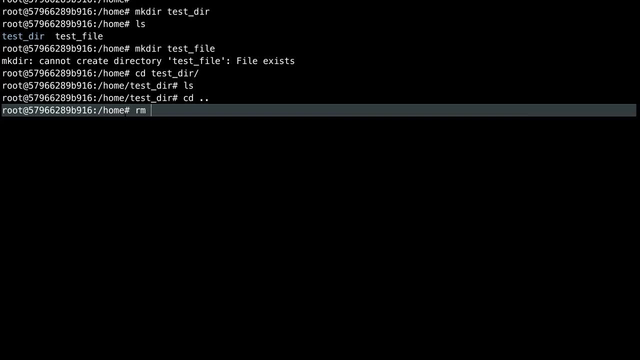 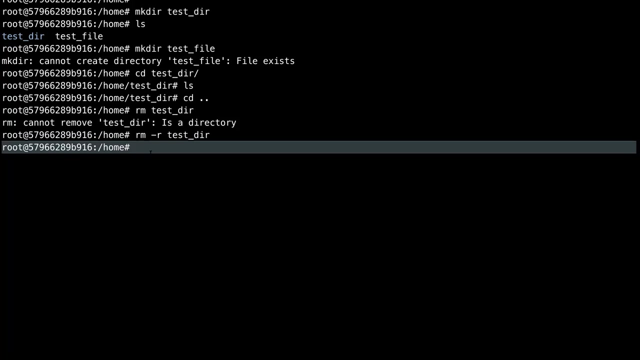 delete this directly. okay, using rm command, rm and test directory. okay, now it is that cannot remove. this directory is a directory, so of course i have to provide a flag here: rm minus r. okay, this is very important. see, when i uh, when i was deleting your file directly, you can use rm and then the file name. it will. 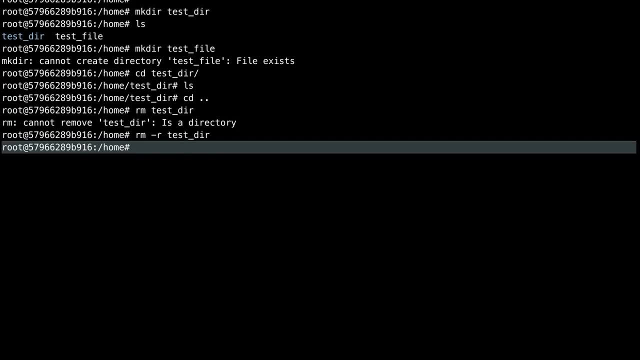 delete it. but in case of a directory, you cannot use it, since the directory can consist of a lot of files and more directories, right? so you have to use this flag minus r to delete the direct. now, if you do ls or you should not see the directory, it has been deleted. now, if you want to change the 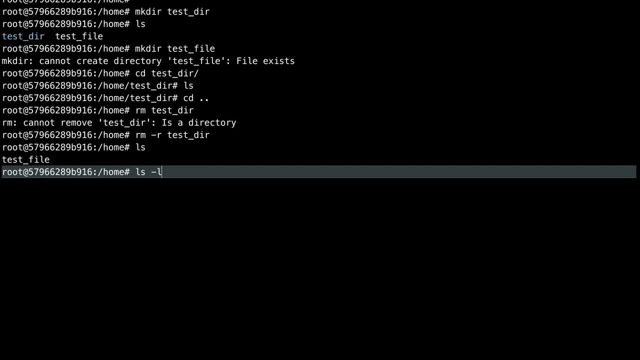 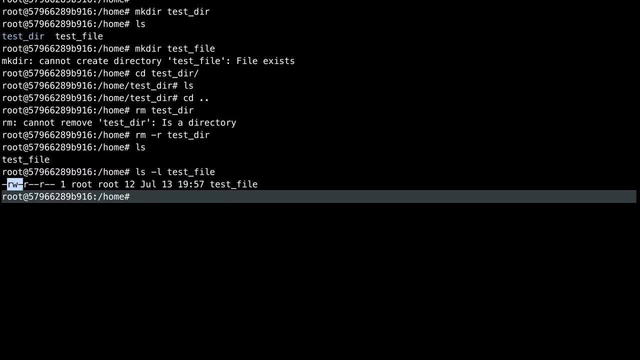 permissions: right, so you have ls. you do ls minus l on test file. okay, so these are the permissions that are there. so basically, uh, if you go into the details of this- i know i'm not going into very details of this- so these are the permissions that read right and this is for execution. so these are the permissions for the. 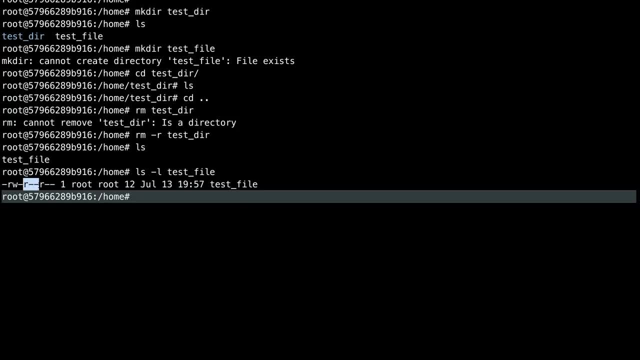 owner of this file. that is root. now, these three are the permissions for the group- uh- i mean group- owner of this file. that is again root here. and these three permissions are for all other users, basically right. so here the permissions are for the uh owner of this file. that is root, this root. 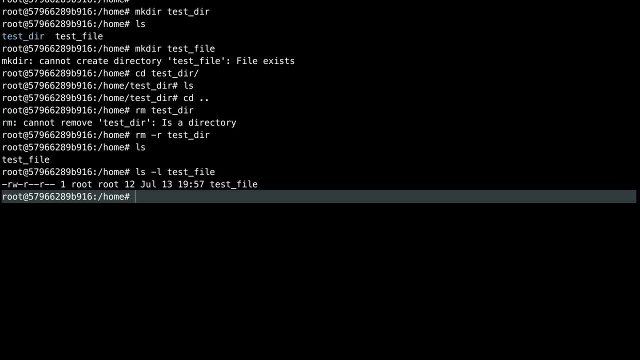 is the owner of this file, the permissions for this router. it can read to it, it can write to it, but it cannot execute it because the third one is for execution and that is not set. so the root cannot execute it now for others. if you see, the others can only read this file. they cannot write to it. okay, now, uh, ch mod is. 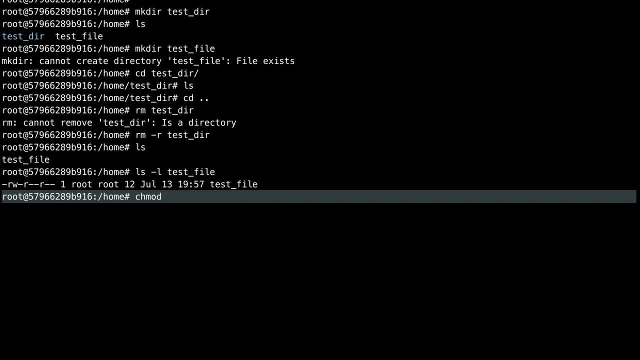 command is used for changing the permissions, and i'm not going details of this command, but let's say, if i want to give a right permission to, let's say, both of these, i mean the, this group, i am. where is the route? no, best way, i'm not going to see it. besides, for example, this is theiji. 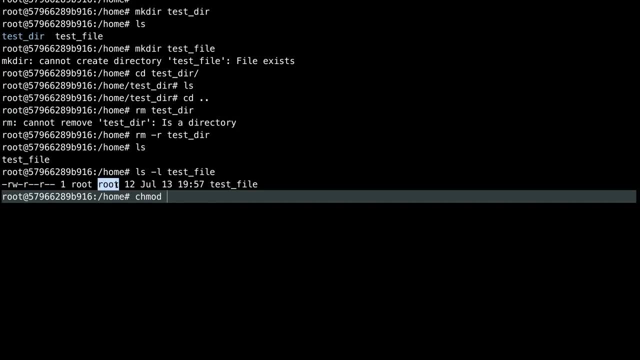 also i'm group users also i'm in the root group, uh users in root group and also other users. if i want to give write permission, i can use chmod and for like, if i i i know the. i mean what. this is right: read write, is there right? so that is basically uh. read is uh three. sorry, read is four. 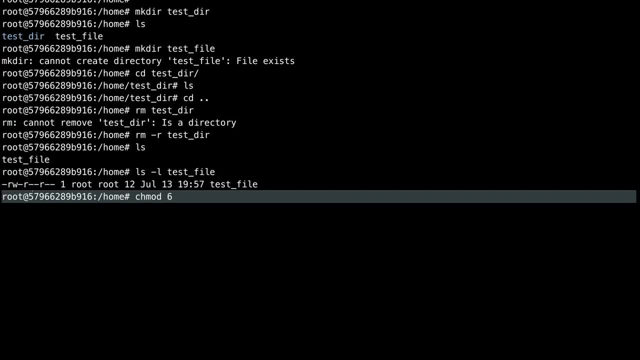 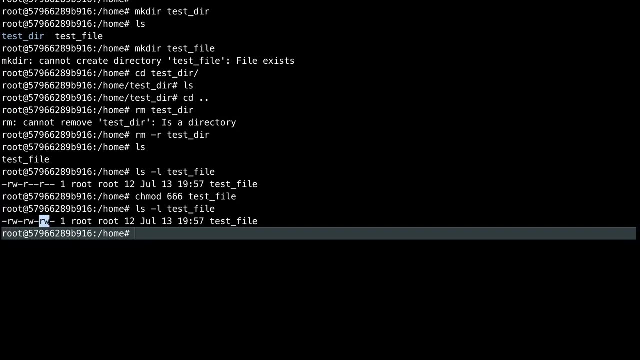 four plus two is six, so the permission is six. uh, this will be basically again six, six, six. i will do okay and test file now. if i do again, lx minus l. okay. now you see other like this group has also got right permission. now others has also got the right permission. like this is one of one way of 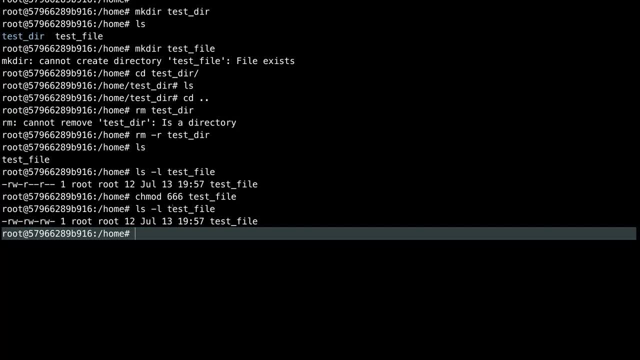 changing the permission and i'm not going to details of what i did like chmod command. it's a bit complex command and i will provide you some references to read about it, but do remember that chmod command can be used for changing the permissions. now let's get back to 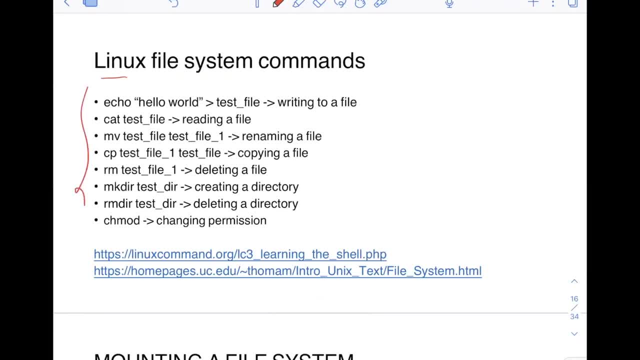 here, and here are same things i have written here, all these commands i have written here, and i've also provided some references, like, if you want to read about these commands, how they do, what they do actually and and what other operations you can do with these commands. 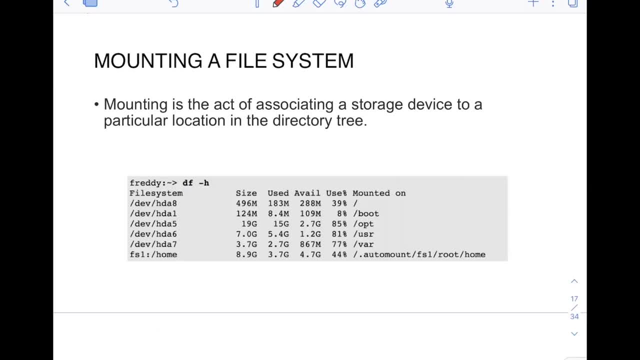 let's uh discuss about mounting a file system, for mounting is the act of associating a storage device to a particular location in the directory tree. okay, so of course let's say you have the hardware device, right, you have this hardware device. now you have to, i mean, mount this at some i mean path. basically let's say, right, maybe let's say if you want to. 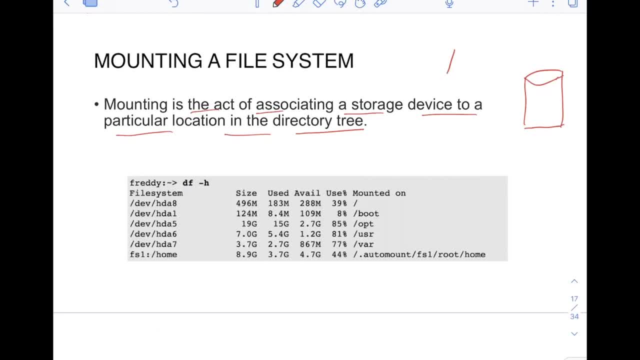 mount this to root path, right? so you have to use. i mean, of course there is command called mount in linux. you can. so why do we need to mount this file system? right? the reason is that i mean, we do not know, right, we cannot directly know. i mean, let's say, if i want to store some, 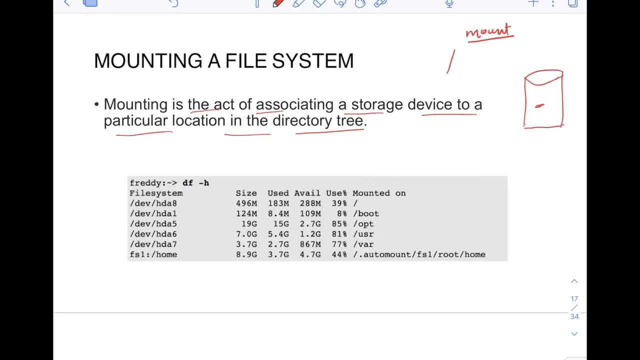 file on this disk, right? so how do i- i mean, reference that right? how do i reference that? of course i need some path, right? and for i'm this path, i need to first mount this on some path, right? so let's say now, if i have mounted this on, let's say uh, root, and let's say maybe, opt, let's say okay. 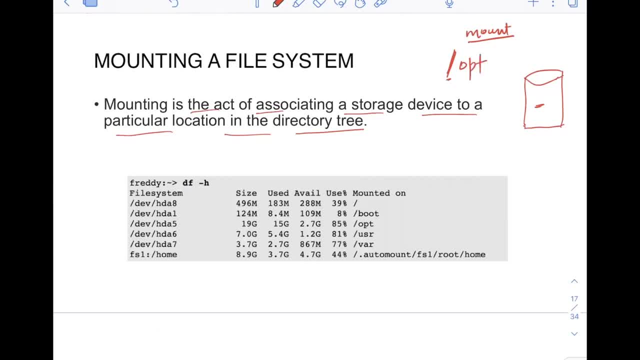 i have mounted this- uh, new, i mean hard disk that i have on this path. let's say, okay, i want to create some new file here. let's say right, and write to it, for example. again i can use the echo command, for example: right, hello world. let's say same thing: right, hello world. and then i will write to some. 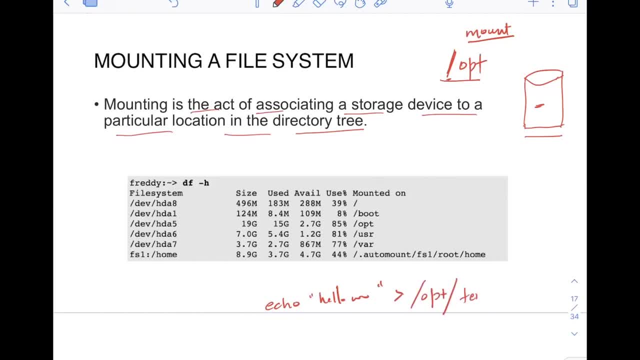 file here, opt and let's say tmp- tmptxt. okay, now what will happen is: uh, since you see this path right, opt defined slash, tmp, txt, and since i have mounted this uh hard disk at slash opt, this file will be stored in this hard disk. okay, so of course you can have multiple hard disks also in a system. 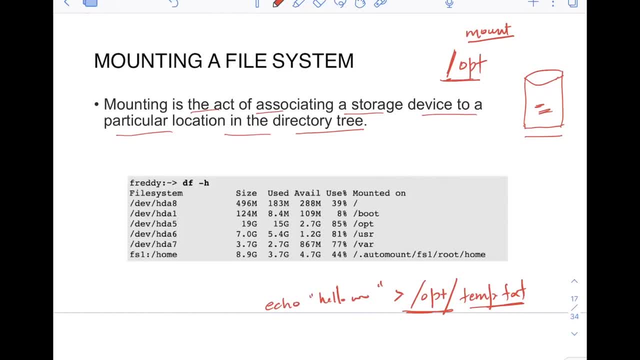 right, even one hard disk, you can partition it into multiple right, multiple smaller partitions. so one of the command you df minus h, which can be used to see all the- i mean i mean all the devices that are mounted here, so you can see here that, uh, you have only one. 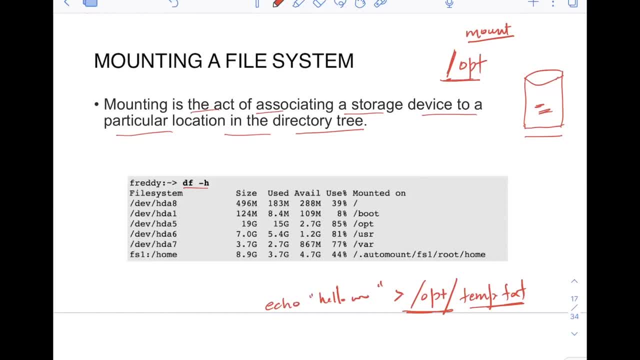 disk and do remember, if you remember correctly. uh, i told you everything in linux is a file. see, all the disks also are represented as file itself. right, slash, div, slash, hd8, slash, div, slash, hd1. right, that's what. that's what i told when i was telling that everything in linux is the file. 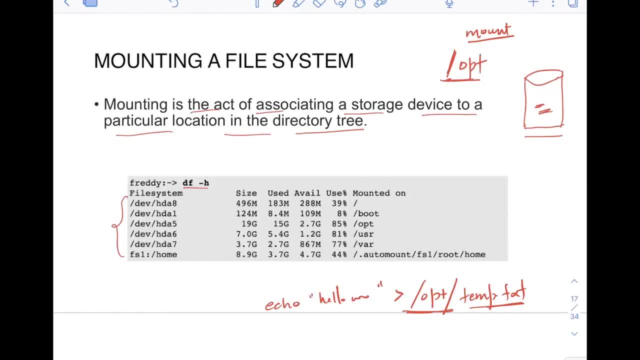 and you see every, every of this. so basically, these are your hardware devices. of course, you have only one disk- h, h, d, a- but this hd has been divided into multiple partitions: one, five, six, seven, eight, right- and all of these have a mount point. if you see, hd8 is mounted on root. 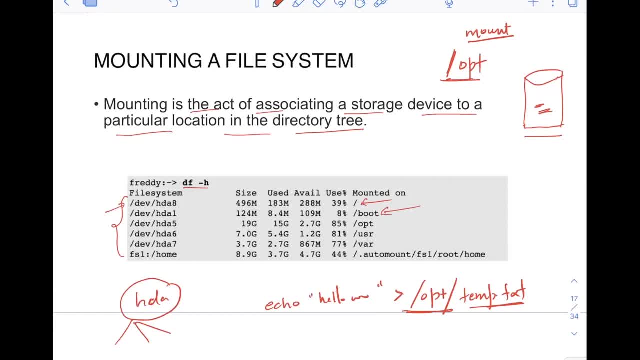 hd1 is mounted on boot. similarly, hd5 is mounted on uh, i mean slash, opt and others also. and also, what is the size of this? uh? uh hardware devices, disk right or obvious partition 496 uh m right. what is used? how much is available? how much? 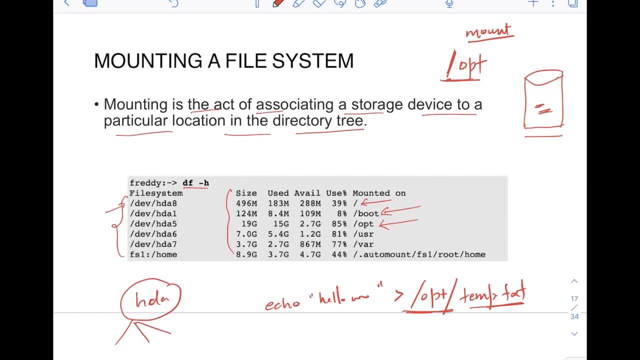 percentage is used. all these stats are you can, you can, you can use df minus h command and you will get it. so if you do not mount a file- i mean if you do not mount a device, right storage device- then you cannot use it. how will you use it? right now? this was all about understanding of files and 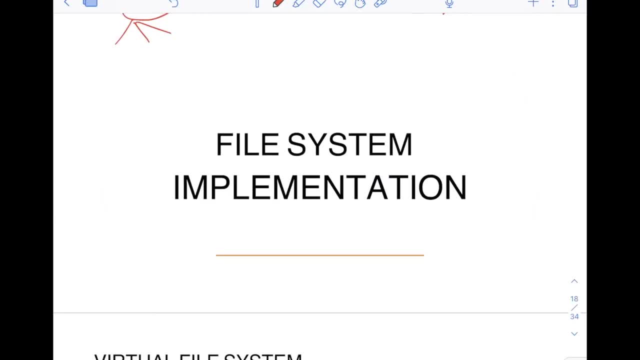 directories and linux i mean commands, for i mean doing certain operations on files and directories. we have also seen the c code, also right- for opening a file, closing the file, reading and writing to it, for example. and these are mostly very closer to you, right? you are doing most of these operations in your day-to-day. 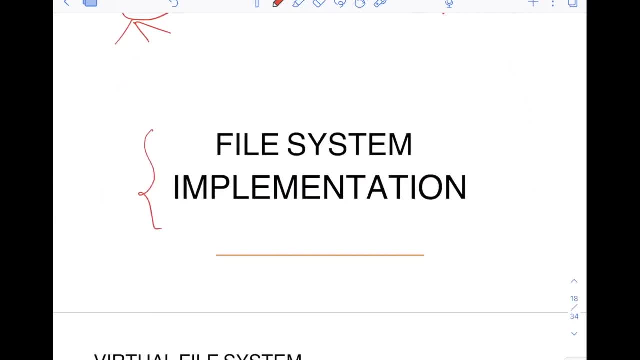 work. but let's now go to file system implementation. so of course, you are not doing- i mean, you are not seeing this in your day-to-day work- but this: the concepts of file system implementation are very important. so how this file systems are implemented internally. so what happens actually when you do? 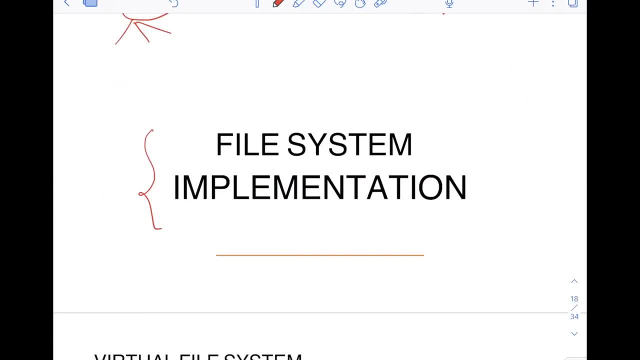 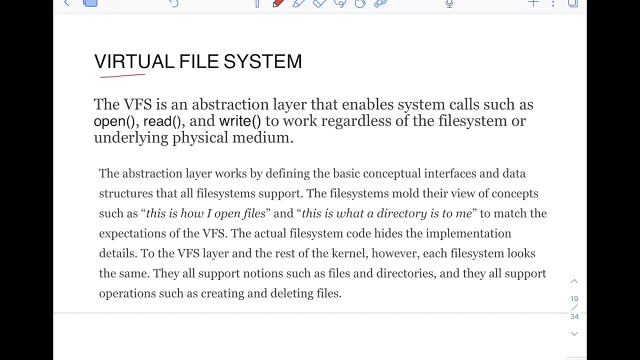 this: read operations, write operations, what- what actually is happening on the background? you can see this in the background. right, that we are going to see now. so in linux operating system, okay, virtual file system is used for implementing the file system. so it's the virtual file system, or? 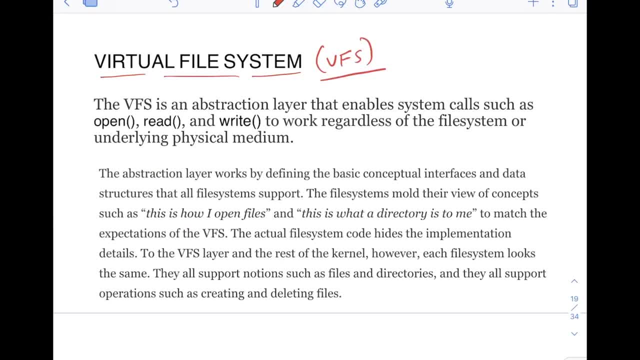 this is also called as vfs. that makes everything possible, right, the reading, writing, uh, whatever you're doing, all the operations that we are doing. so this virtual file system makes all of those possible. so the vfs is an abstraction layer that enables system calls such as open, read and write. 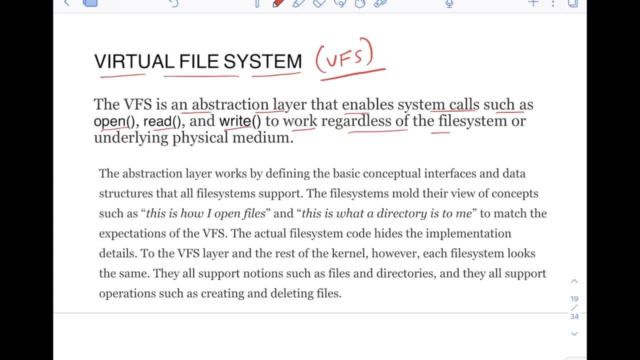 to work regardless of the file system or underlying physical medium. so these three lines are very, very important lines to understand what vfs is. so vfs is a kind of abstraction layer, okay, and you would have heard this abstraction layer a lot. so if you have done object oriented programming, you would 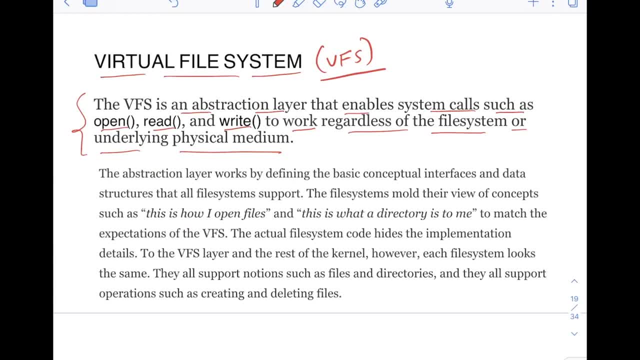 have seen the concept of abstraction there, right? so in object oriented programming you have something like: uh, abstract classes, right? for example, abstract classes you have in there, right i, i? i do not remember a lot about this, but you do have something like you just define. that i mean. 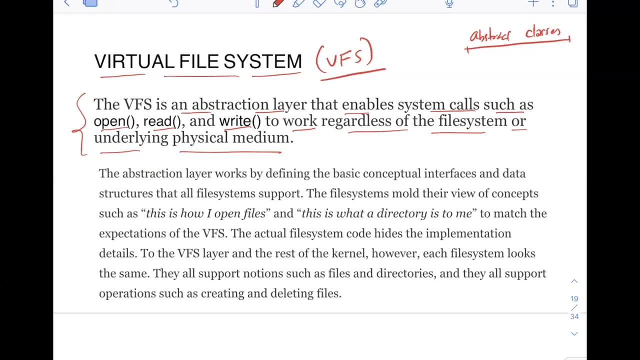 some classes. right, you define those classes, you define some functions in those, but you do not provide the implementation of that right abstraction layer works by defining the basic conceptual interfaces and data structures that all file systems support. okay, so basically, this vfs is going to define all the interfaces and data structures that all file systems supports but do. 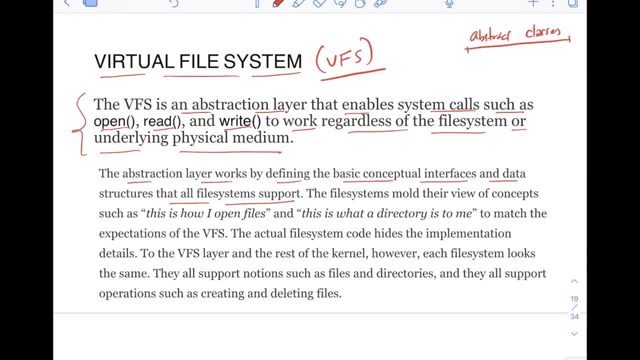 remember- this is important. this vf is not going to implement these data structures, interfaces- right, it is not going to implement those. it's just abstraction layer. it defines those data structures and interfaces, but then each file system has to implement this. basically, okay, the file systems mold their view of concepts such as: okay, this is how i open files, okay, and this is what it. 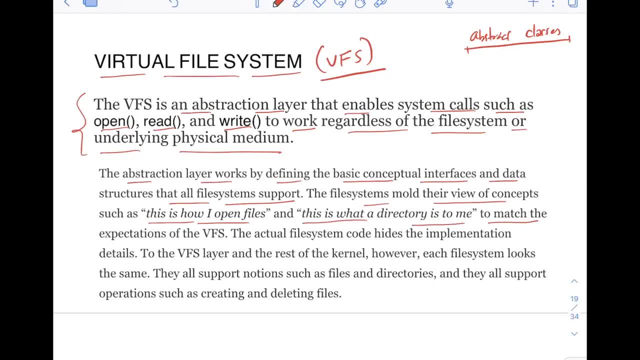 actually is to me to match the expectations of vfs. okay, so vfs has already uh provided a data structures and functions. now all the file systems has to match the expectations of what vfs wants. okay. so let's say vfs wants something like: uh, if let's say create i nodes, okay, let's say just. 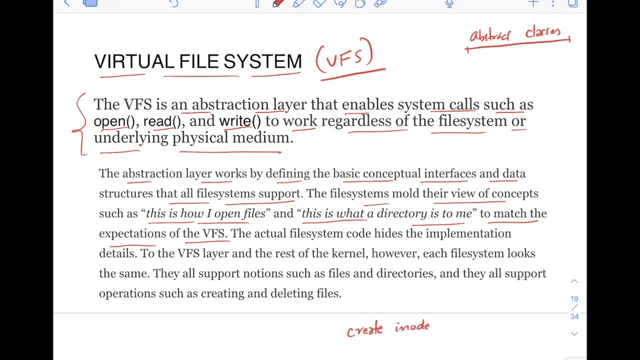 example, vfs has a function called create i node. okay, now there are multiple uh different file systems. let's say: you have fat, is there, okay? and the uh fs is there. let's say: ext score is there, okay, all of these five systems are there. now, all of these file systems has to 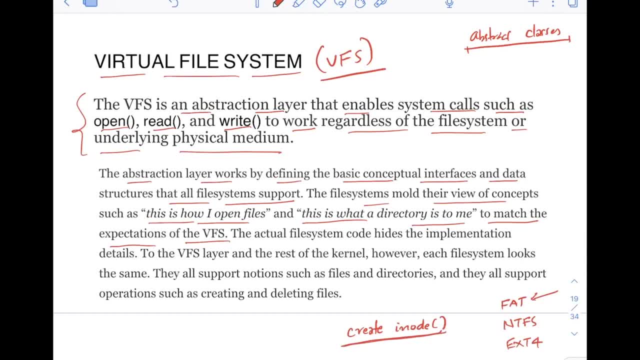 implement this method. okay, now, vfs will not implement this. it is just an abstraction layer. now this file systems have to implement this method, create i node. so this vfs is not concerned with how this file systems are implementing this method. it is only concerned with: okay, this would be returning kind of same thing. basically, what is it expecting? right, of course. 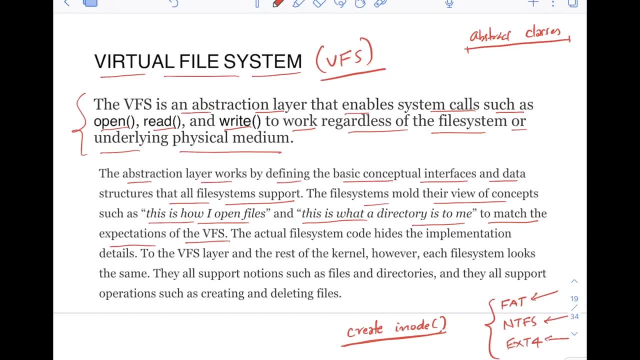 it is expecting some uh uh results after this function is implemented. right, that's what it needs, nothing else. it does not care about how you implement this for different file systems, of course. i mean, all the file systems are different, right, so they will typically implement this in a different way. but the vfs is only concerned with the answer of that: uh, how they are. 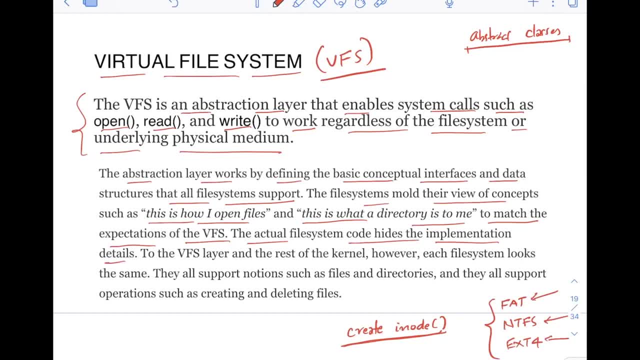 implementing that. what happens through the use of vfs? okay, it is not seeing all this, whatever code they are doing right, whatever code they are running on the background to implement this. so, basically, it is getting hidden from that, and that's what is the importance of having an abstraction. 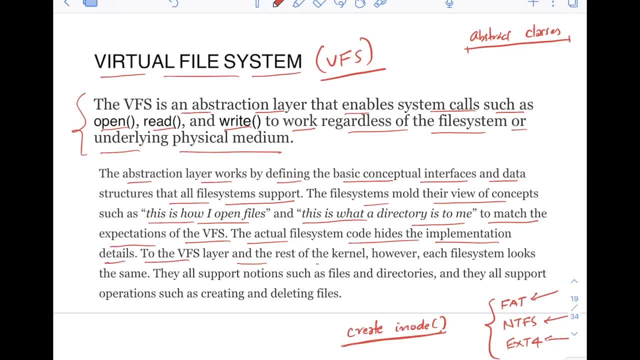 layer, to the vfs layer and the rest of the kernel. however, each full high system looks the same. of course, these are not the same file system. they are very different, fat is very different and tfs, the xt4, are very different, but to the kernel and to this vfs, every, every of this file system looks 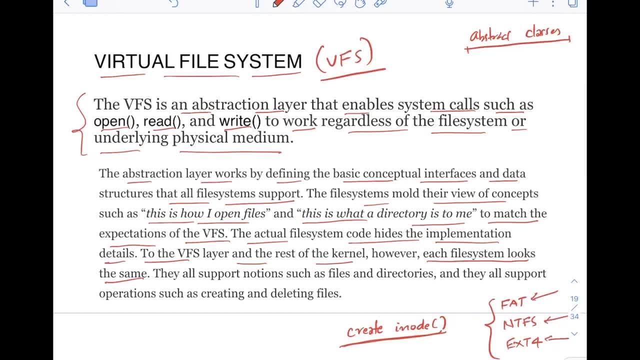 same. the reason is again same, because it is only concerned with that. okay, each of these file systems would implement this function and give it, give it an answer. that's what it is concerned with. and if they are, if they, all these file systems, are supporting this function, then they look the. 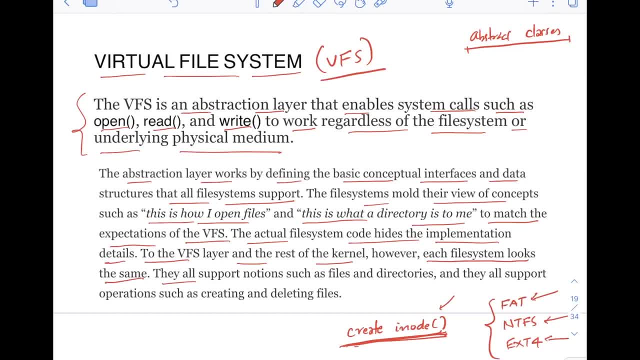 same to vfs, basically. so they also support the notions such as files and directories and they all support objects such as creating and deleting files. right? so all these files, see, all the file systems, do the same thing: they create files, they delete files, they they help in reading the files, they help in writing the files. now, how? 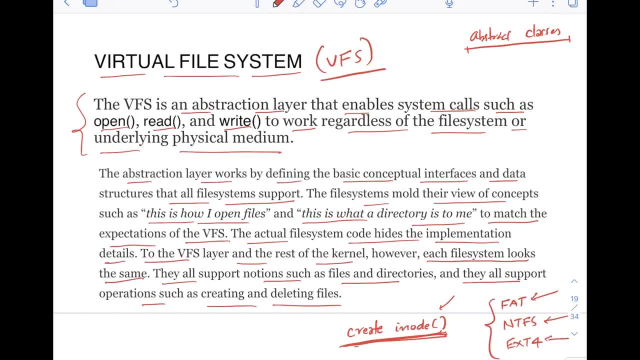 they do is different. right, that can be different. they may be reading. i mean they may be using some different code for reading the file. like, let's say, fat can use some different- i mean code for reading a file, and if and tfs can use some different code. ext4 can use different code. 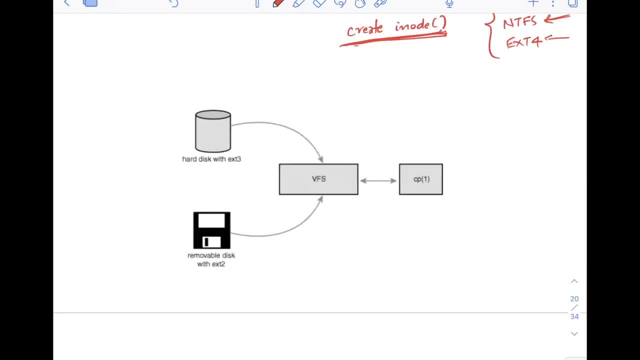 but finally they are going to do the same thing. now take this example to understand more about vfs here. so let's say, if you want to, so this cp, as i told is, is a command in linux are used for copying files, right? so if you want to like, for like this the format of our cp: a file name one, file name two. 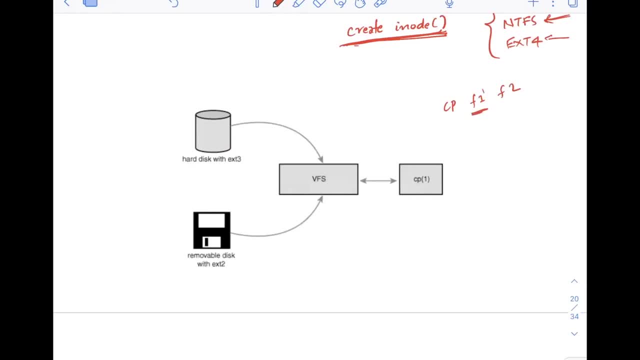 right what this will do. it will copy the contents of file. one this command will do is it copy the f1 into the new file, f2. okay, so here. basically, let's say you have one file on this hard disk that is using ext3 file system. okay, this hard disk is using ext file system. then you have another. 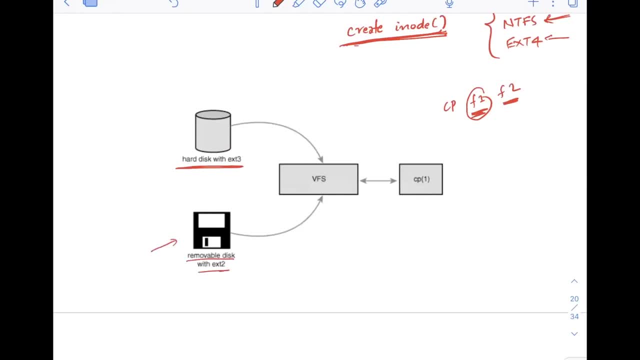 uh, removable disk. that is using ext file system. of course both these file systems are different and let's say: if you want to copy file from, let's say, if you want, let's say here is, let's say there there is one file temp here. let's say: okay. okay, now let's say if you want to copy this file, okay. 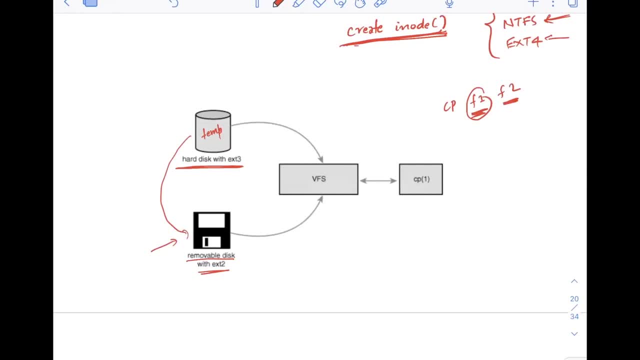 to this uh revolver disk, right? so of course these are different. i on both of these devices. the file system itself is different. okay, now if because of vfs, what happens? it makes possible to copy file from one uh device to another device. if bfs was not there, this would. 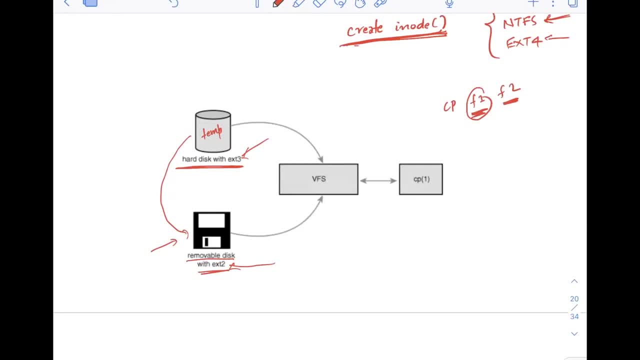 not have been possible because both the files except. so this ext file system is also going to implement read right, right. similarly, this, this uh removal disk, is also going to implement read right, how they implement uh, it can be different. the vfs does not care about how they are implementing it. 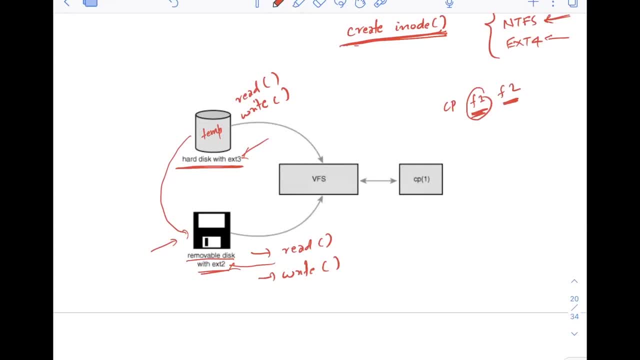 you just care that both are implementing these functions right. and of course, in vfs also read and write are there. okay, these are some functions of vfs and all the file system has to implement this. now, once both the file system has concept of read and write, it's very easy to copy files, right? 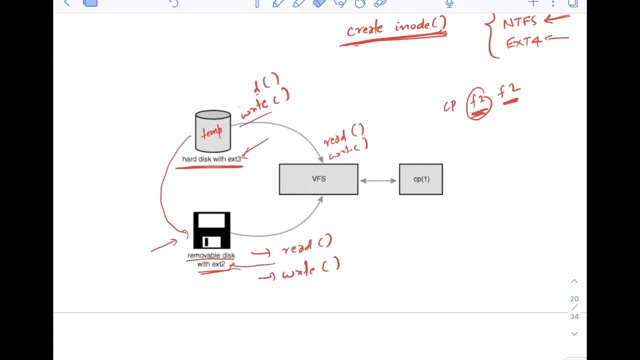 now let's say, let's take the other case, okay, this. let's take the case that vfs is not here. okay, vfs is not there. so what will happen? let's say, maybe this hard disk was maybe have some other function called. let's say, read, uh disk. let's say okay for reading or and write disk for writing. okay. 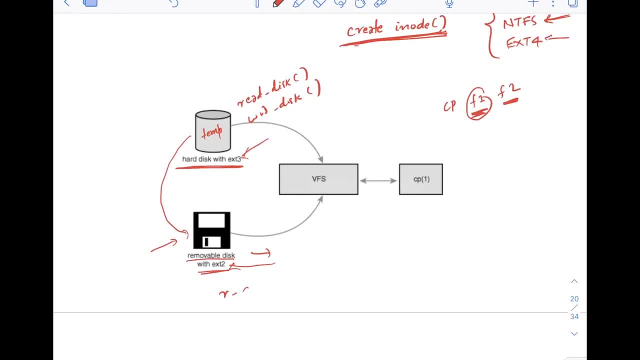 similarly this: this removal disk has something like r disk- r disk read for reading, let's say okay, and r disk write for writing, okay. now you see, both are implementing. like both have different names, right, uh, for reading and writing, and i do very different i. it will become very difficult for the operating. 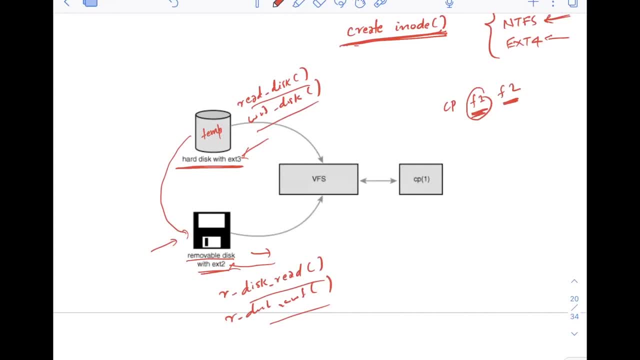 system to remember. i mean different names for different devices, right, and for different sites. really very difficult for the operating system to remember these different functions for different file systems because they can be multiple file systems. now, because of vfs, what happens? it makes it easier for the operating system to uh implement like read operation, write operation, because 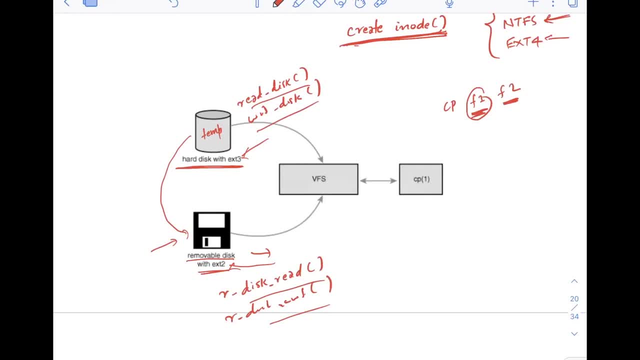 vms or bfs has already defined. okay, that read is there, write is there, and now all of this file system has to implement this same read and write in any way, whatever way they want. okay, that's how i'm. copying between different file systems is possible in linux because of vfs, and this is the abstraction layer that makes it. 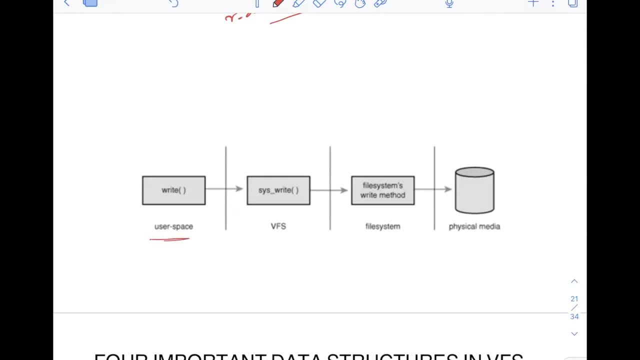 possible, for example. so what happens actually? so let's say: uh, if you remember right, uh f scan f, uh printf we have used in that, if you remember, in the c program we have used this f printf to write to a file. so what happens is this f printf actually calls. so this is also in user space. 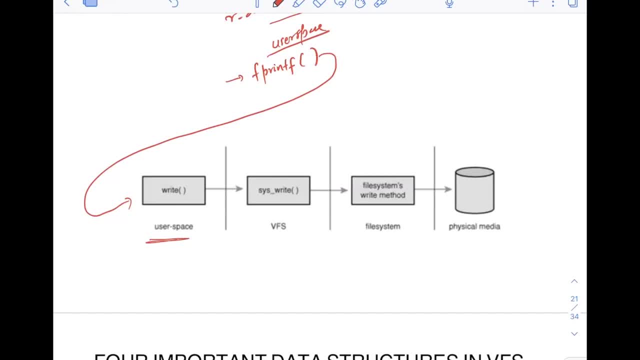 user space. so this app printer will call right. okay, right is also called in user space, so this right is basically the system call. now, once this right is called, we use system call now, the- i mean now the flow will change. now you will, you will enter the kernel space, basically from now onwards, so once the system call is called, you. 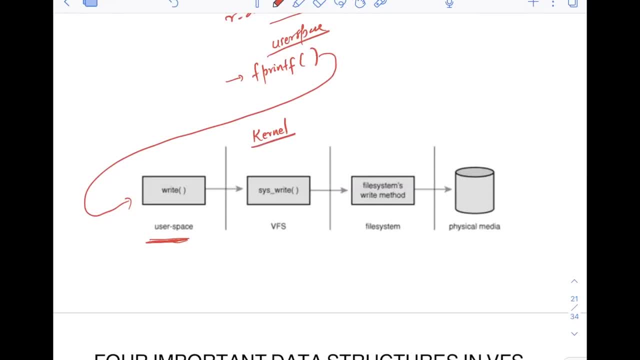 enter the kernel space. now in the kernel space you will have the vfs. okay, now this vfs will have the implementation for this right called this underscore right. okay, now, this is underscore right. should be implemented by all the file systems that are supported on this operating system. so then it will ask basically a file system to. i mean with this call syswrite to this file system. 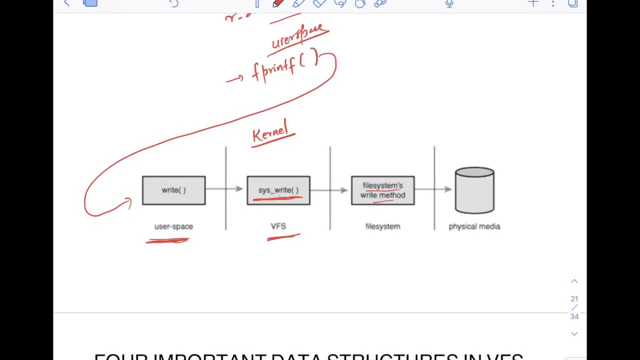 now, of course, system will have its own right method. it does not matter, it will. just file system will see that the vfs is asked for sys underscore. right, okay, now it- if file system can, of course can have its own method. let's say, uh right, maybe some file maybe. let's say, this is 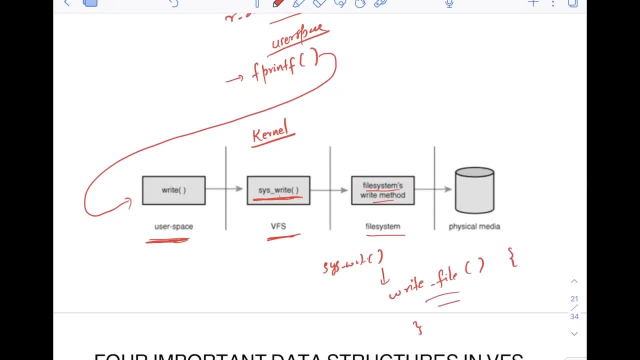 the method of the file system itself. right, some code here now, file section, will run this code. okay, whatever code is here and finally, whatever i mean you are writing, this will be written to this file media. right, that's how, uh, the operations happens. right, the reading and writing operations. 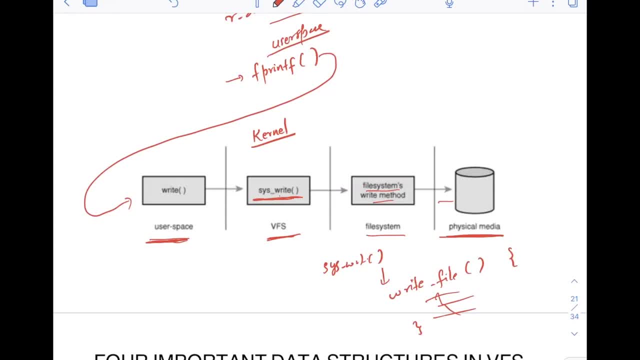 so even if you have a read operation here, then in that case it would have been app scan of in c programming. right, you will have a scanner. this is again in user space. now this will call. i mean, instead of right, it will call read here. okay, here it may be a sys underscore: read in the vfs. 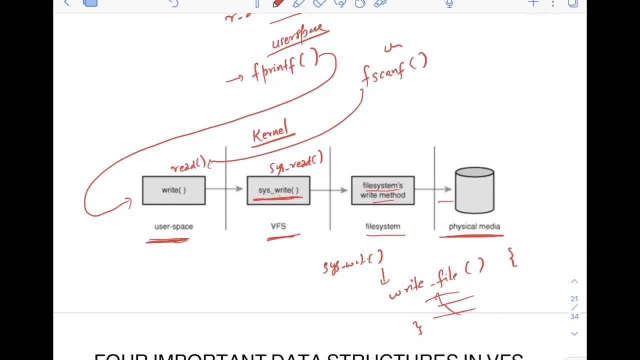 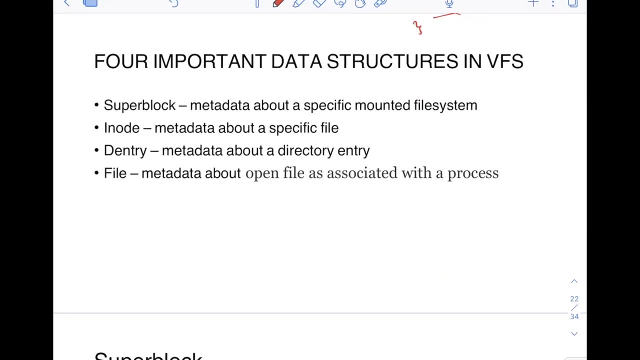 okay, now this will call the file system right to read and file system will have its own implementation reading. okay, it will execute that code and finally, i mean you will read from the physical media. now there are four important data structures in vfs, which makes all this possible, right. 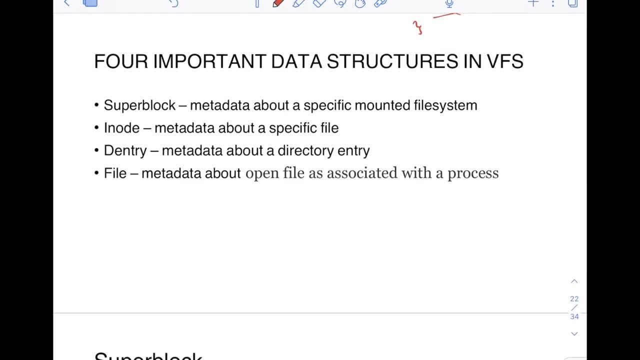 so, as i told, right, one of the important uh use of vfs is that, like there can be multiple file systems using multiple uh, so they can. so one of the one of the important use of vfs is that you can have multiple file systems. right, you can have multiple file systems on your operating system. so 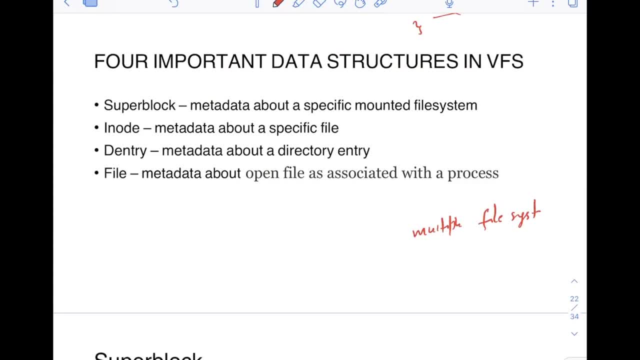 you can have multiple file systems and these multiple file systems can be there on multiple devices, right? so one file system can be there on a floppy disk, right, copy disk. one file system can be there on the, let's say, hard disk, okay, one can be on the ssd itself, right, and this vfs makes it. 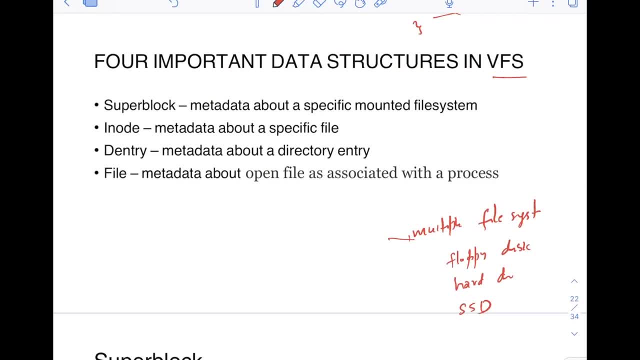 possible to communicate between all of these different file systems and different types of devices. right, and that's the magic of vfs. actually, now, how does this magic actually help you? right? so this magic only happens. so this magic happens with the help of four important detailed structures or four different objects. okay, if objects are basically- i mean concept of object oriented. 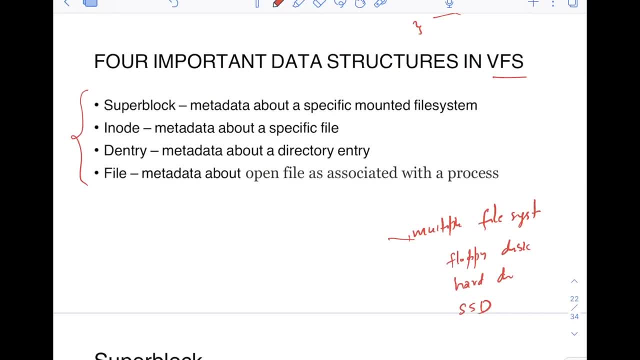 programming right, and that's what is happening here. right vfs is also, of course, the code of uh. vfs is written in c programming language, in linux, and c does not have concept of object oriented right, but still it tries to go into that way- basically right- and define these objects. 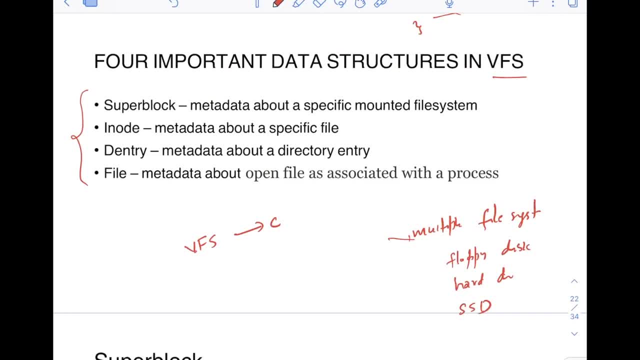 basically, of course, in you use a structure, right struct, for defining this right. you don't have concept of creating classes in c, so you have super block. i know dentry and file- we will discuss in details about this- but these are four important data structures in vfs. so super block stores the. 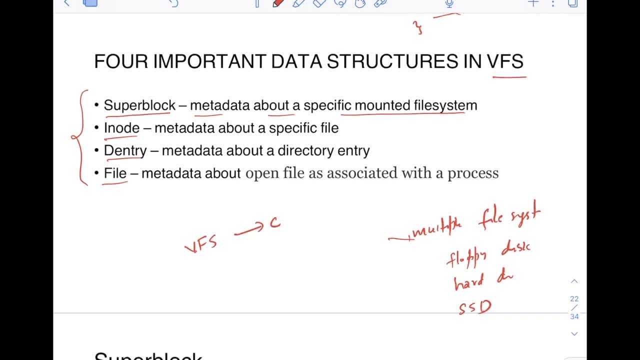 metadata about a specific mounted file system. okay, i know. store data metadata about a specific file. dentry stores a metadata about a directory entry and file stores metadata about open file and associated with the process. of course, for now i have just read this, read this definition, but later on i am going to go to details of all these four important data structures. so 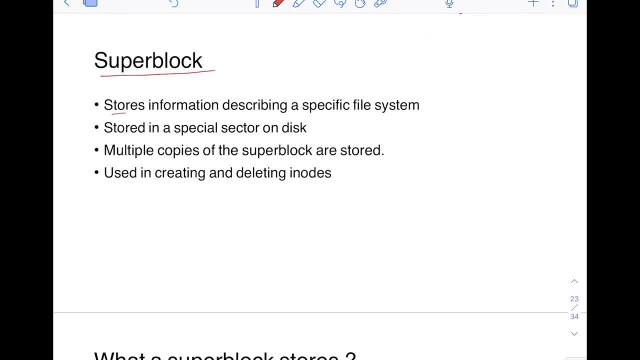 let's first look at super block. the super block stores information describing a specific file system. okay, so, uh, if you remember right, we have a concept of mounting the file system. okay, so let's say i mean, i mean, if you have a specific file system, okay, so let's say i. 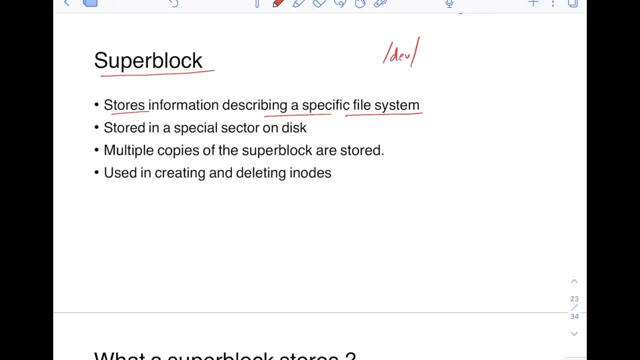 have. let's say something like: uh dv- right and s d a one right. let's say, this is mounted at the root. let's say, okay, this is the point. and let's say, of course, first you also have to format this disk using some file system, right? let's say you are using, for example: 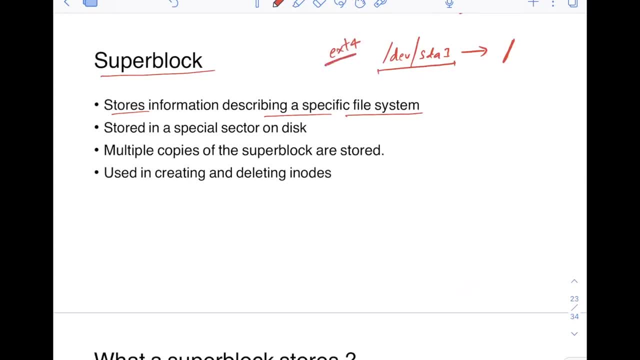 ext for file system. right, you have formatted this disk using ext for file system. so, basically, this: this is using, uh, uh, this file system- ext4. okay, now a lot of information has to be stored in the file system, right? so let's say you have a file system, right? let's say: 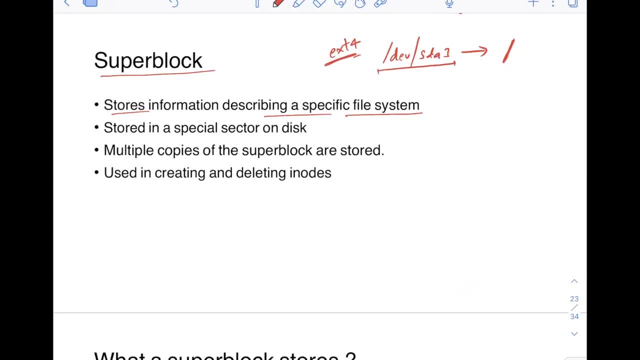 record this, right, so you can see this file system, right. maybe this the code regarding this right, regarding this, where this uh disk is actually mounted, for example: right, and you can also remove this mount. right, you can later on, let's say, you can also remove this mount and you can change it to dev sda one, maybe some other, let's say this thing okay. 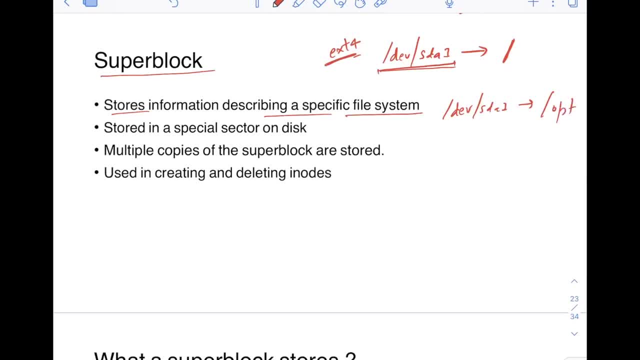 you can, of course, do this and you can change the mount points also in the future. so these are all. information are stored in super block and this is stored in a spatial sector on a disk. so, of course, this deev underscore- sorry it is, it is exactly what we have. let's say: 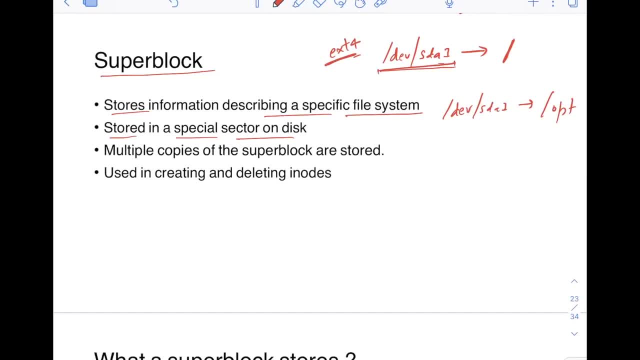 code. sorry, slash, slash, div, slash, hdl1 is there, right? this is. this is a disk, okay, and this information, the super block, is a data structure, right? the this is actually stored in a particular spatial and place in this disk somewhere and, of course, multiple copies of super block are. 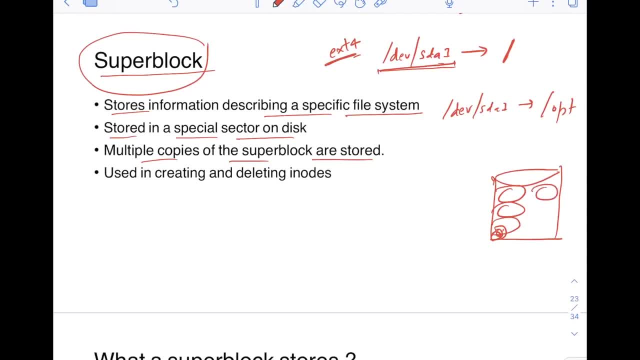 stored. of course, you have different sectors here, right? a lot of sectors are here, so multiple copies are stored of this. the reason is that this super block is very, very important for the operating system, for the file system itself. so you need to like, if one of the- uh, let's. 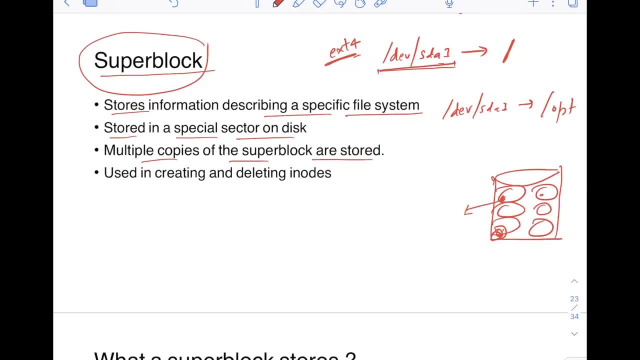 say it is stored here, right, and this becomes corrupted right, so you can use other copies of this. this is also used in creating and deleting i nodes. so i will discuss about, i know, say later on, later on, but this is used, super block is used for creating this, uh, and. 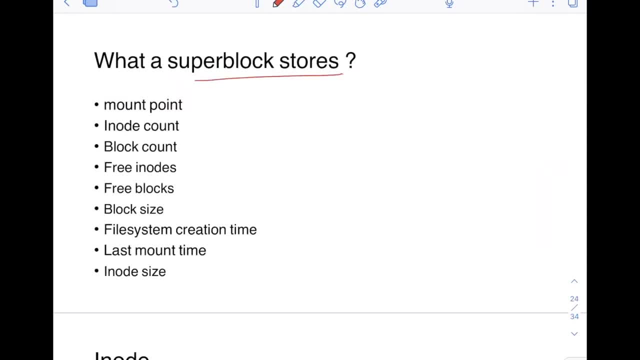 deleting these, i nodes. so what does this super block stores? so of course i told right, it stores the metadata about the mounted file system. so these are some of the metadata it's stored. the store the mount point where the file system is mounted. it stores how many. 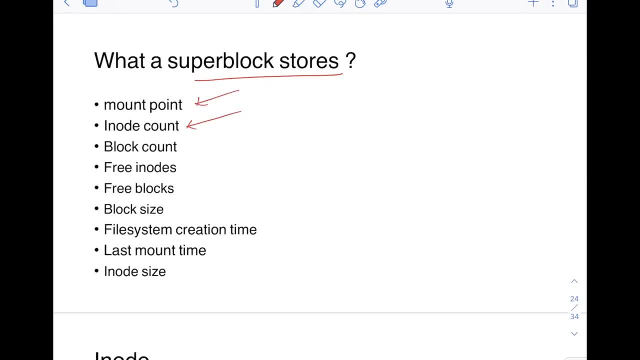 i nodes are there in that file system? how many blocks are there in that file system? as i told you, right? uh, for the file system it will see. i mean, for the discourse it is offended, right, it is sectors. but for the file system it will see all of. 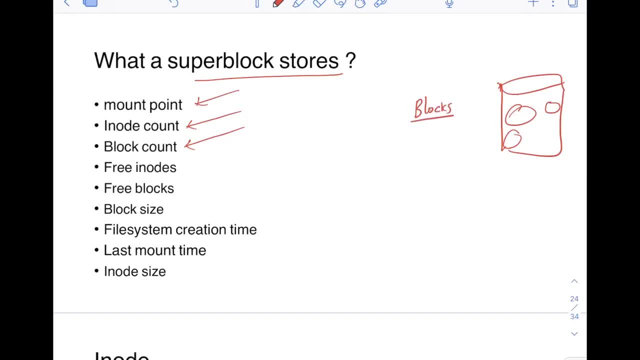 them as blocks. okay, basically right. so it will basically store how many blocks are there, basically, how many of them are free, how many of them are occupied? right, all of those, all of those information will be stored in super blocks. so, how many i nodes are free, how many? 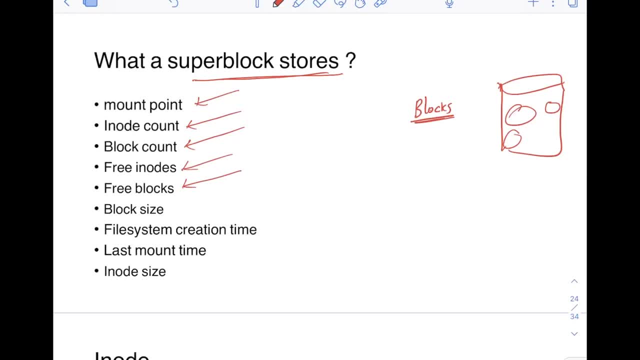 blocks are free. yeah, everything is stored. gustado. so here next drop something like player. so basically, whenever blocks are free, it will write to those free blocks, basically right. it will basically ask the disk to write to those free blocks and then, of course, for those free blocks, there will be a mapping to three sectors here in the disk and then the disk will write to. 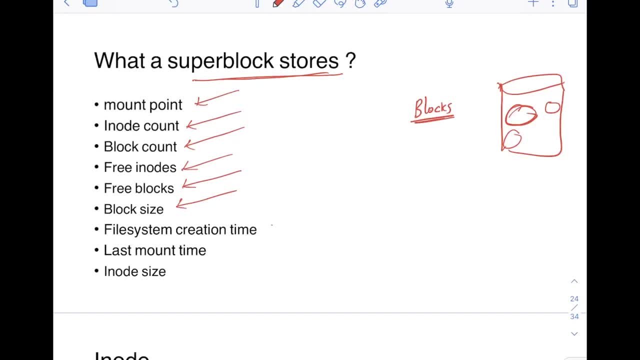 it then? what is the block size here? when was the file system actually created? or what was the last mount time? i told you right. the mount points can keep on changing, right. so what was the last mount time? what is the size of the inode? of course i am telling a lot about inode, but i will discuss. 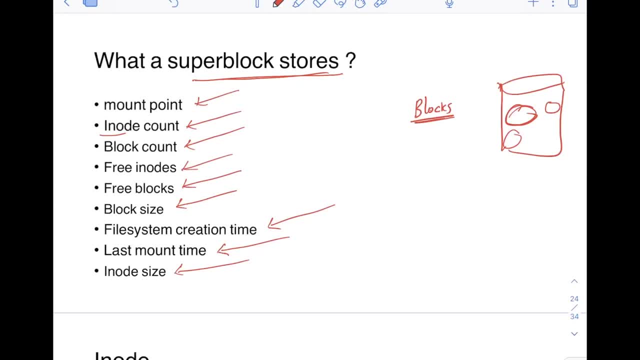 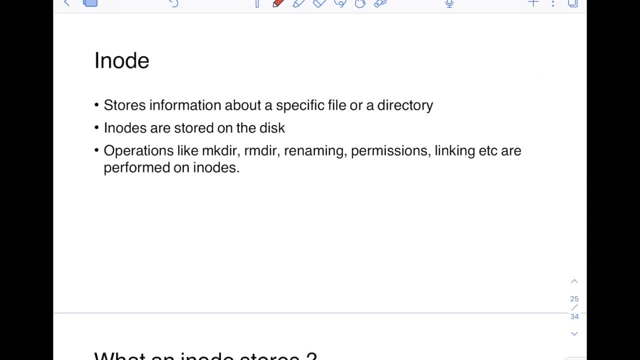 inode next, so you understand what inode is. now let's discuss about one of the most important data structures: uh. in a linux file system or on a bfs that is inode. you will hear this. inode terms a lot, so this stores information about a specific file or directory. now see uh in linux files and 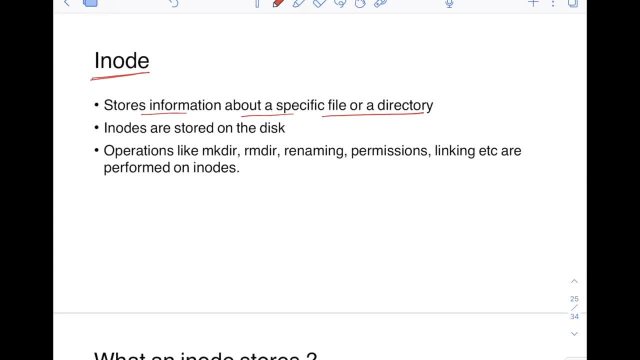 directories are treated as same. okay, both are treated files itself and this inode stores information about these files and directories. okay, i notes are also stored on disk. okay, these are also stored on, like some sectors on this. now, operations like: whenever you do those operations, remember right, mkdir, rmdir, de naming. 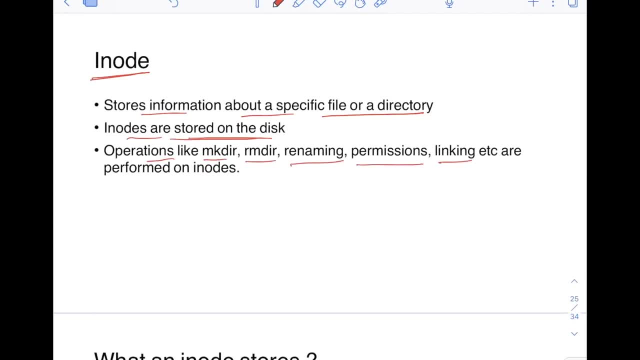 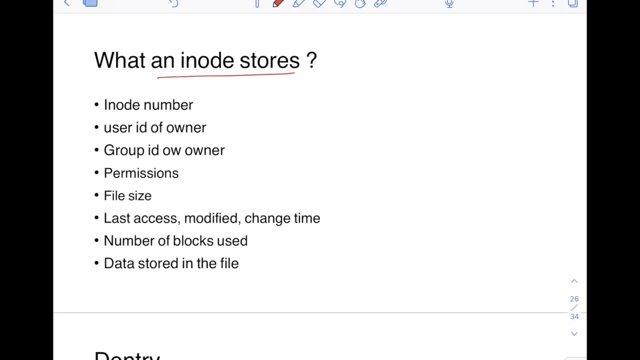 permission, changing, linking right. all of those are performed on inodes. you remember that. okay, now what an inode stores? of course it stores information about a file. so what information are these? i notes are itself, and so i notice that when the data is stored on a directory, 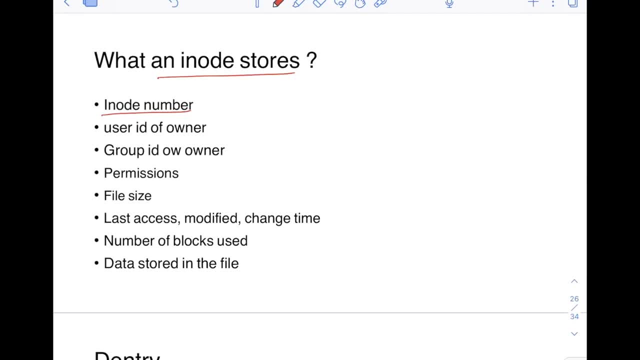 and all of the data is stored on a directory. so we will see that inode and linux files are need file. of course. i know number is there because you need to uniquely identify. there can be a lot of i notes so i know numbers are there to identify each i note uniquely but then a file can have the 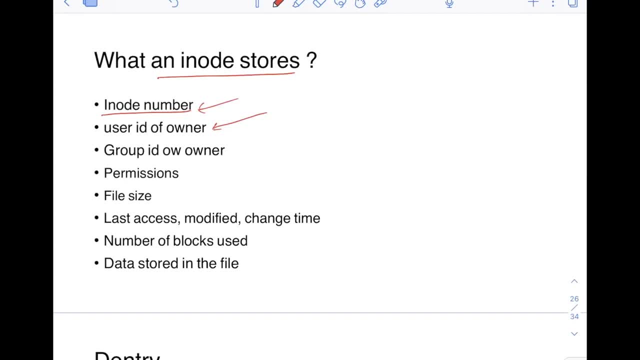 user id of the owner, right, who is the owner of this file? who is the- i mean- group owner of this file? right, that is group id of the owner. then, what are the permissions for this file? uh, what is the file size? uh, what is the last access, modified, change time for the file, right? this all will. 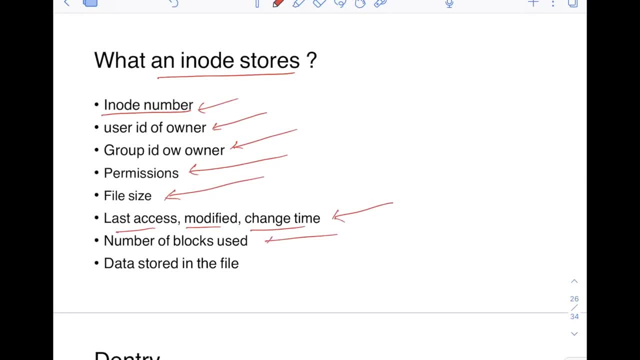 be stored in. i know how many blocks the file is using, right? uh? what is the data stored in the file, so that all will be stored in i notes? of course data will not be directly stored, so, again, data will be typically stored in: uh, some blocks, right, some blocks data will be stored. let's these three. 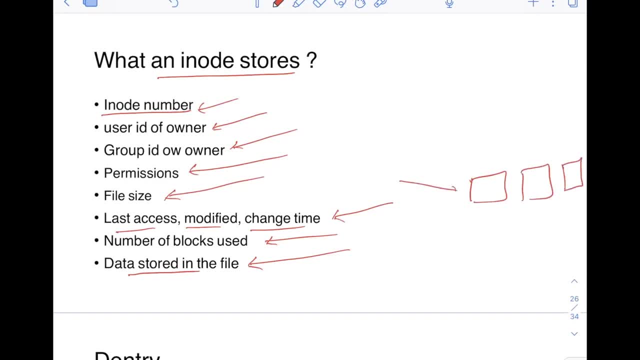 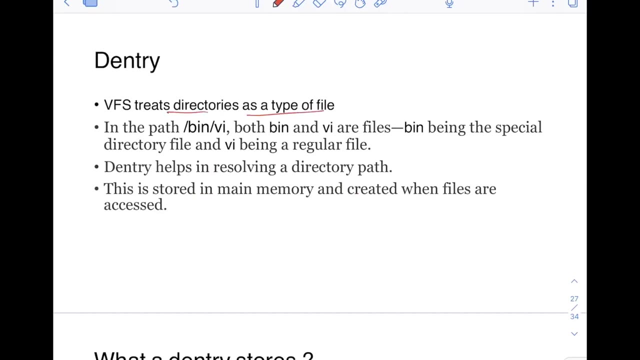 blocks. so this i node uh will have pointers to this. okay, i know, will store the pointers to this basically. okay, that uh, the data is stored in these three blocks. it will store the pointer stories, basically. next one is dentry. dentry is also very, very important for vfs, trees, directories as a type of file, as i have told you. 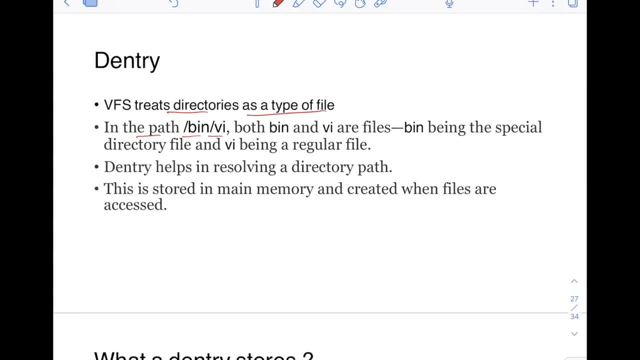 now in the path. let's say, slash bin, slash vi. both bin and vi are files. of course bin is a directory, right, and vi is, let's say, file, okay, so basically here bin is directory and vi is the file, but for vfs it will treat both of them as files itself. you will not treat bin as 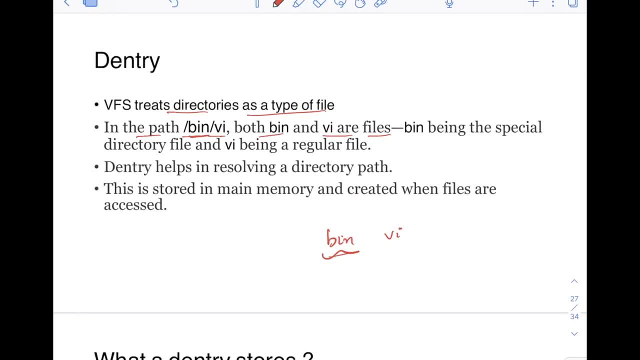 straighter directory or something, you will treat that also as files, bin being the special directory file, of course, and vi being a regular file. of course bin is also a file, but it's a special directory file and vi is just a regular file. so let's say, if you have a uh path, 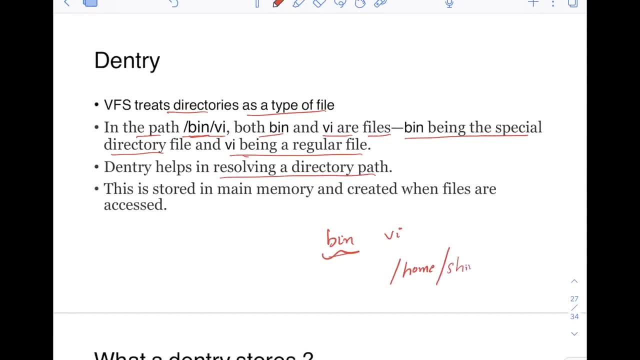 like home. okay, shivam okay, and some uh temptxt here, okay, or you need to resolve it right. so basically, the main aim of uh see all of the data, right about this. so i want to access this file, okay, i want to access what is stored in this file, right, temptxt. so of course, i know that. 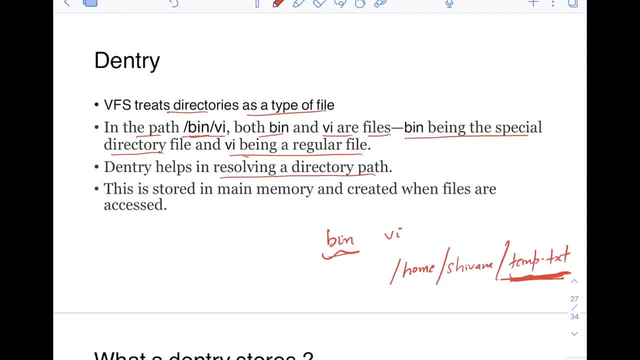 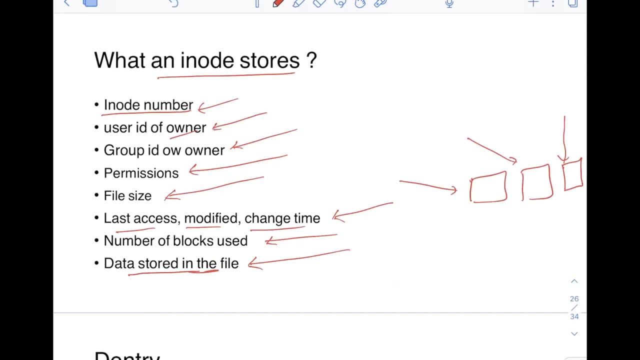 all the information about the. this temptxt is stored in a i node. okay, because i know it stores all the information about this file, like who is the owner of the file? uh, everything right as i told here, right? uh, user id group on the permissions, file size and also data, right it? 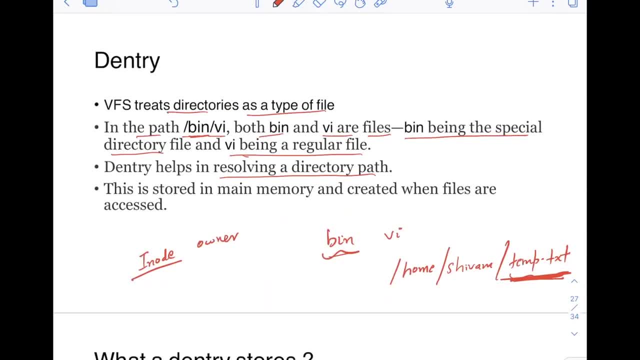 also stores. i note also stores. so i note for this file right tem dot txt. m dot. it will also show where data is stored. you will have pointers to where the data about this stem dot x is stored. then we can read it right. so first we need to find what is the i node number associated with. 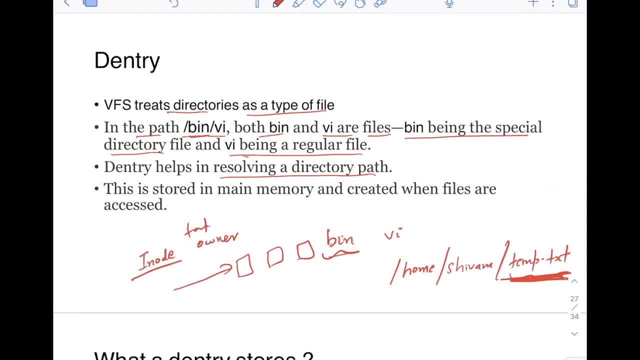 this file we need to find first, so for that you have to resolve this path first, right, so we will discuss about that later on. how this is done, we will discuss in some time, but this is done with the help of dentry. also, dentry is stored in the main memory and created. 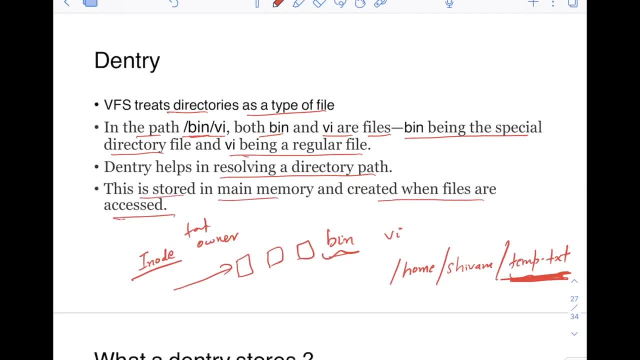 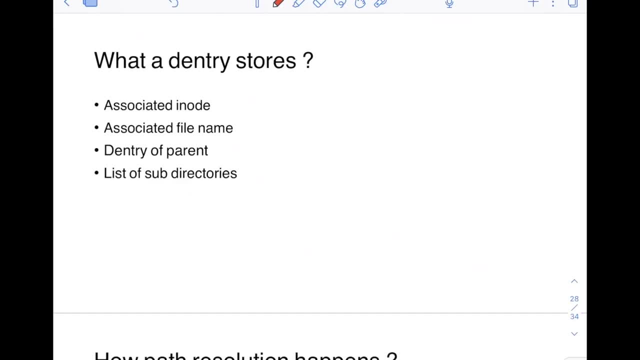 when files are accessed. okay, so the entry is not stored on the disk, it is stored in the main memory and created only when the files are getting accessed. now, what a dentry stores? it of course stores the associated i node. okay, it also stores associated file name, of course, with this i node dentry of the parent. so basically i mean: 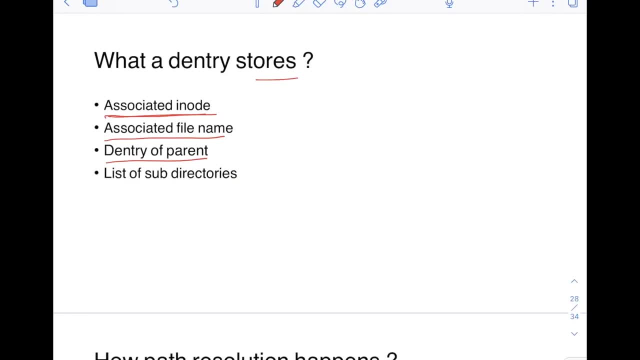 for this. i mean, of course you are. you are at some path, right? so so see, this dentry of object is created for all of this. so you have slash bin and i a slash vi, for example, right? so here here it can be broken down into four components. 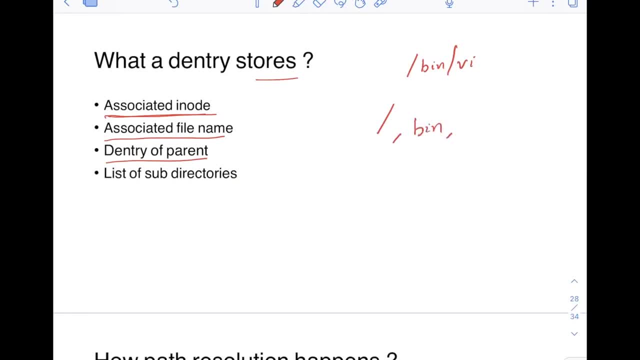 slash bin- slash is again, i mean same as this- and vi. okay now, of course, the unique ones are slash bin and vi. okay, now for each of this. there will be a dentry object created when you are accessing this files. okay, now for each of this. for example, flash, right it? 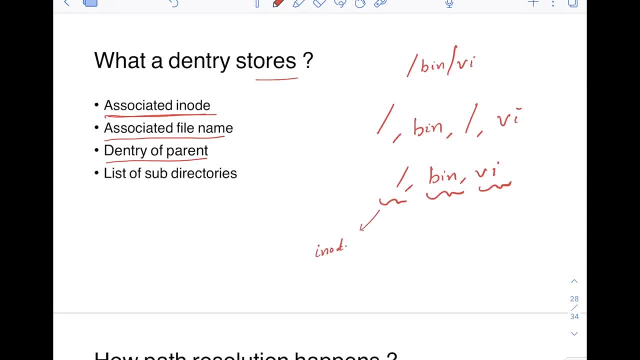 will store. okay, what is the i node associated with this slash? okay, because, for example, if, as i told right, slash is kind of a path itself, right, what is i node with this then? what is the isolated file name with this? okay, so of course that is slash here. it's the right this. 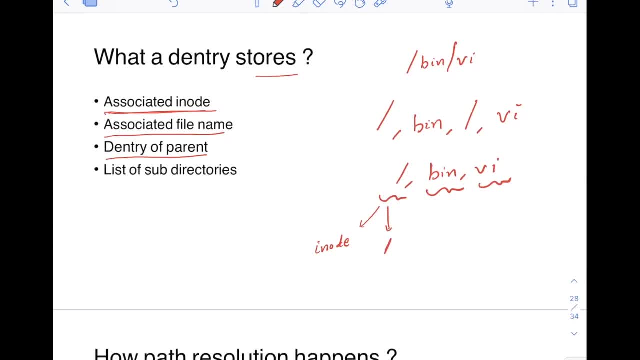 is the name dentry of the parent, so of course slash does not have a parent, so there will be no pointer here. okay, now list of sub directories. so there are a lot of sub directories inside that right. like you have: bin is there, home is there right? it will store this also here. 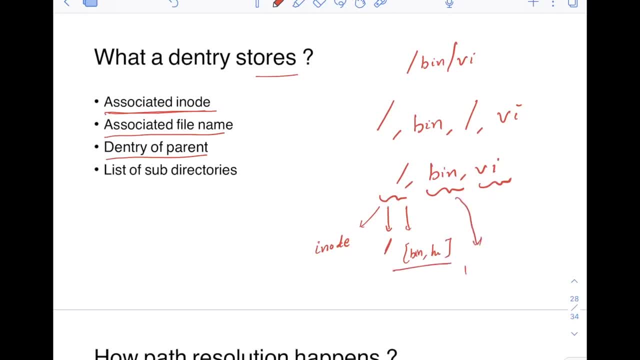 or similarly for bin. again, it will store what is the i node number, right? so of course bin is a directory, right, and directory will also have a i node, as you did with it. so which is the i node, as you do with this? what is the file name of this? okay, i mean of course bin here, then dentry of the. 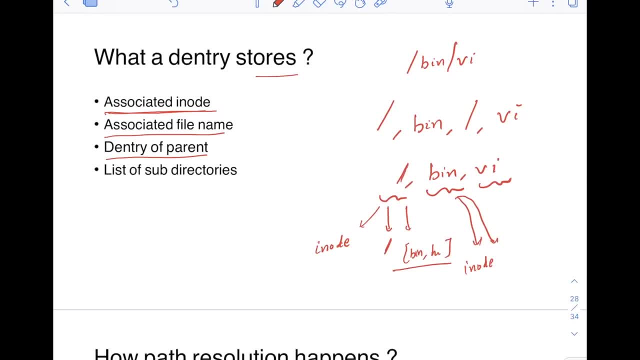 parent here, right? for example, here, if you see parent is this one, right, so it will also store this dentry of the parent also here. similarly for vi also. these all information are stored in dentry. okay, and we will see how this is very useful in resolving a path. 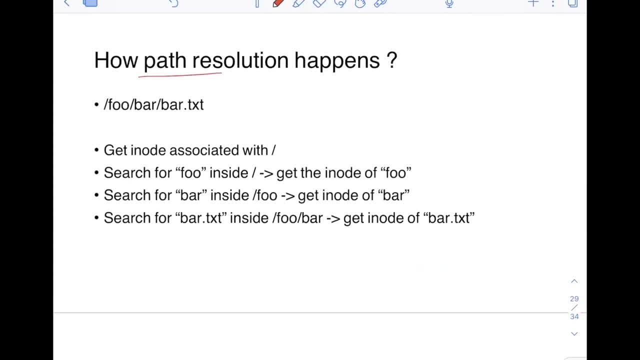 now how path resolution happens using dentry. this is very, very important. so let's say: if you have something like this path, you have resolved this part right. slash foo, slash bar, slash bar dot txt. okay, now what will happen? first, you have to get i node associated with. 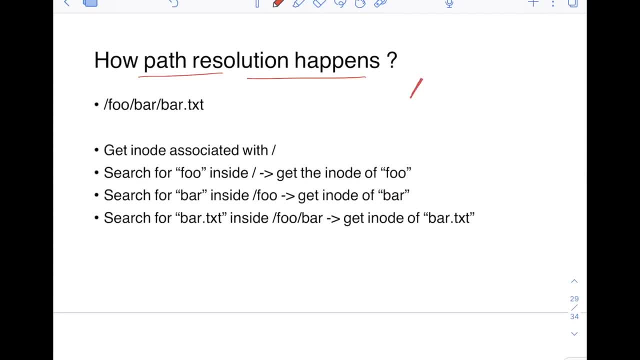 i mean this one. so basically, this path is: first, this slasher is there, right? so you have to get what is the i node associated with slash. so this is typically hard coded and stored in the opening system. so there will be some inning. so in our system, where the 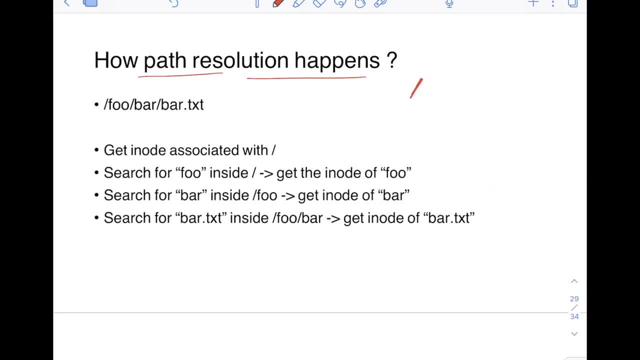 dot dot dot is that means the path, path, type, path, like this: dot dot, dot, dot dot dot with hard-coded uh inode number for this. okay, so let's say you have got this right now. you have to. so once you have got this, now you have to search foo after. after this, you have the foo directory, right. 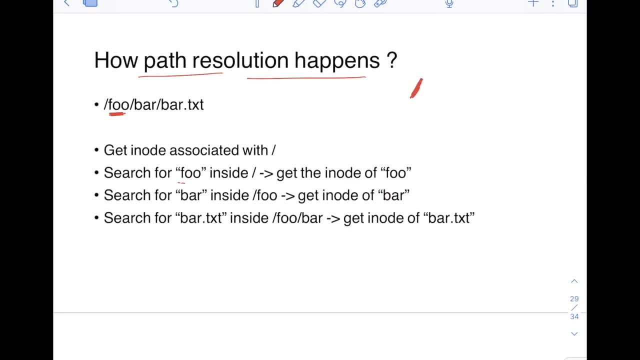 so you have to search the inode for foo directory, right? so you will search for foo inside this. uh, i mean slash, right? so this i mean, if you get the inode for this, and then you will have the pointers to the data, right? what is stored in this? so, of course, in 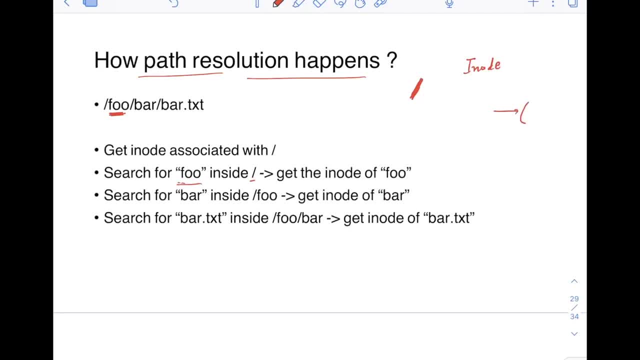 slash. you have a lot of directories are stored right, so they will be stored something like: uh, maybe something like maybe zero one- i'm just giving an example here: bin, comma zero two, maybe lib, okay, and other directories also are stored here, okay, so basically it will also search for foo inside this. so somewhere there will be maybe foo. foo is also there somewhere. 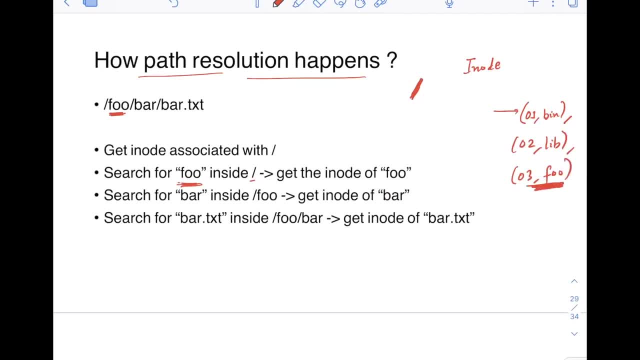 right now it will get. get the. using this entry, it will get the inode number of foo here. okay, now it knows. okay, what is the inode number for foo. now it knows this. okay now, once you have got the inode of, i node of foo, but now in the foo, 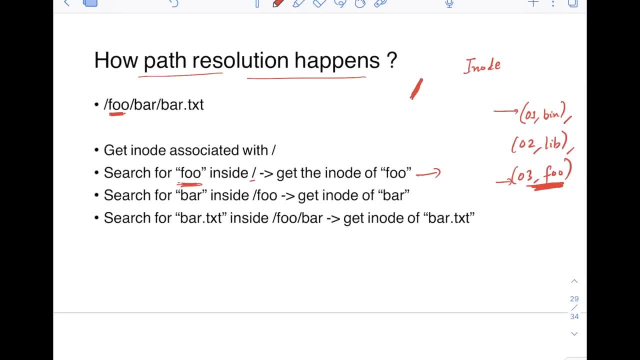 now you need to search bar, okay. so again, let's go to i node of now you are in i node of foo, okay, and of course this i node will also store the data, okay, and pointers to the data again in. i mean, in this i node, this is of foo, you will have a lot of direct trees here, okay, like of course, let's say, 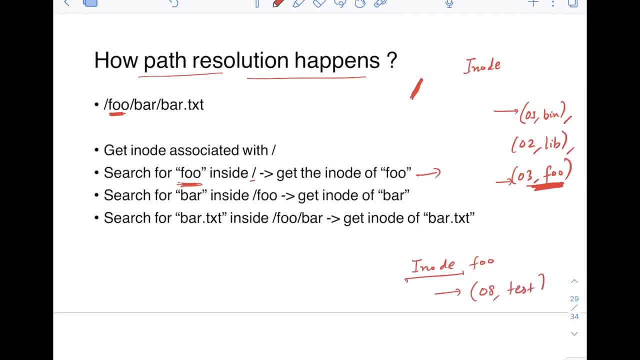 something, maybe test, is there? okay, and zero nine, uh, bar is here, okay, okay. now, basically, we are searching for bar. okay, where is what is the? i know number for bar and we see that, okay, zero nine is the. i mean, we have found bar inside this foo directory, right, and 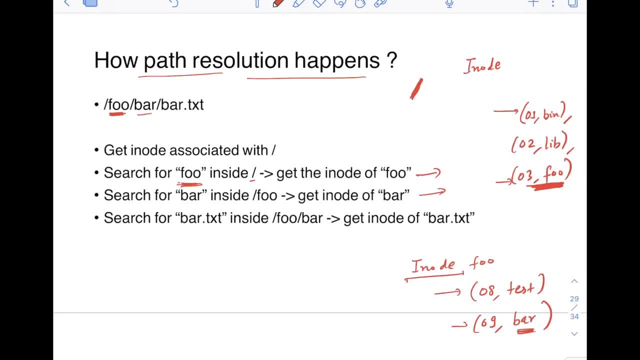 we see that zero nine is the i node, so we have also got the i node number. let's go bar here. okay now. now we know that. okay, now we are in the i node of, basically bar. finally we are here. so small bar. now we have the i node of bar. okay now. of course, it will also contain all the data about, uh, this bar. 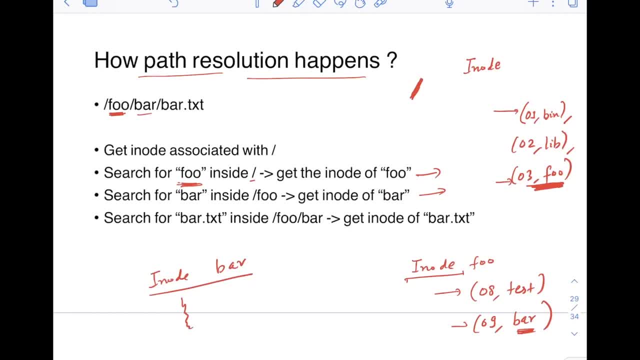 directory, right. what are the permissions and everything. i don't number. everything will also contains pointer to the where the data is stored, right in bar. also, there will be, i mean, a lot of files and a lot of directories, right. so again there will be something i mean again in brackets. 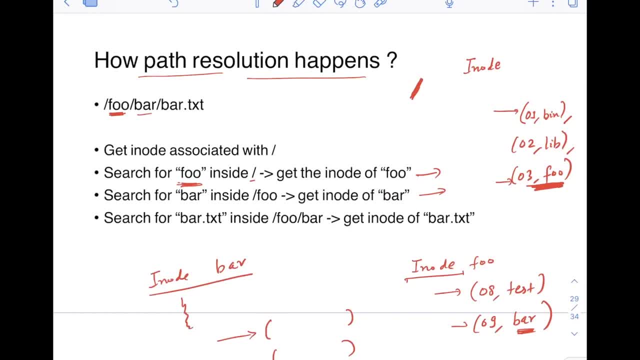 there will be there, right? let's see, i'm just taking this example. i'm not in this the actual way it is stored, just taking an example. so there may, may will be something like you know something maybe. uh, let's say 11 for something like text dot txt. okay, that's the 12 for bar dot txt. okay. 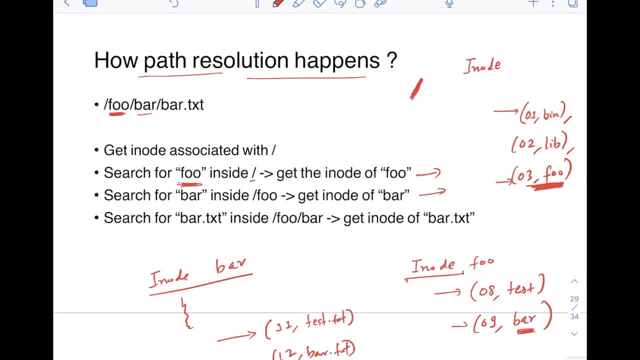 now it will see that. okay, uh, why do you see that? uh, 12 is the i node number associated with this bar dot txt. right, so we know that. okay now, finally, finally, we have got what is the i node of bar dot txt. okay, so we have basically. 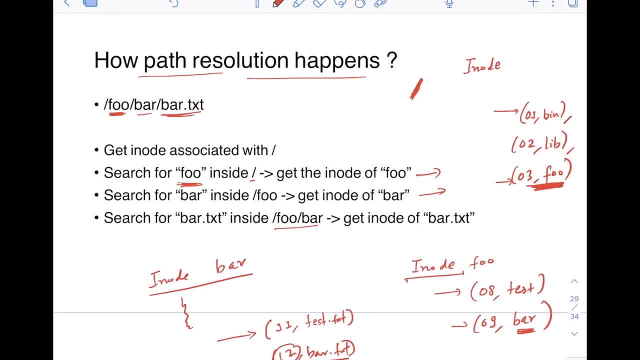 we have gone into this slash, full slash bar folder. now, right, and we have got the iron or bar dot txt. so once we get the i node of this right again, there will be again i node of. finally, we go to i node of bar dot txt. okay, and of course this will again have a lot of information here. but finally, 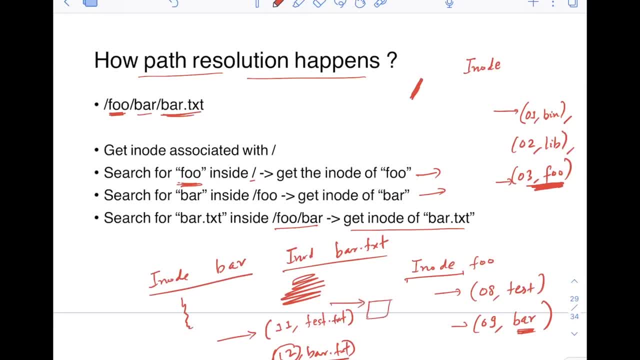 it will have a pointers to the blocks where the data is actually stored. okay, maybe two or three blocks, whatever blocks it is taking, and finally, the operating system should be able to read this blocks, right, whatever data is stored in this and on whatever device it is stored, it will ask: uh that, uh that device. i mean help of this, help of 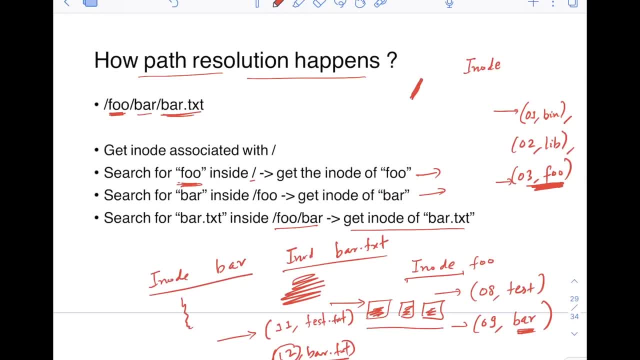 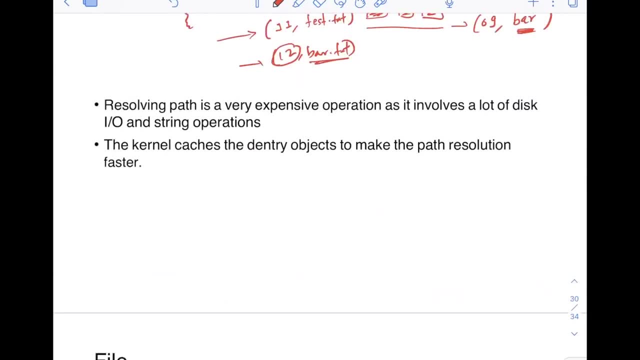 that device, you'll be able to read these blocks. okay, and that's how everything- path resolution- happens. okay, and you- this is very important, right? resolving a path is very expensive operation as it involves a lot of disk, io and string operations. so we have- we are doing a lot of. 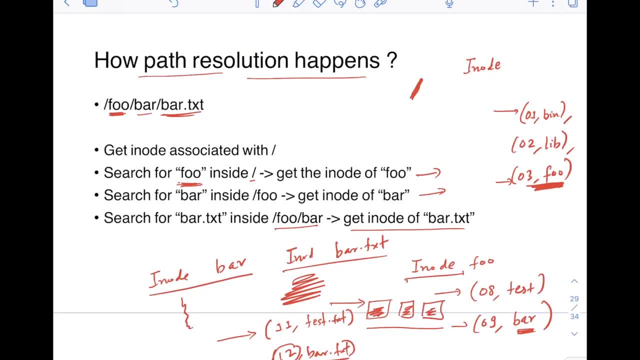 string operations: right, we will be comparing, right. for example, when we are searching for foo in slash, right, we will do a string operation. is this equal to foo? no, is this equal to four? no, this is equal to four. yes, so these are string operations. right, you're comparing strings. 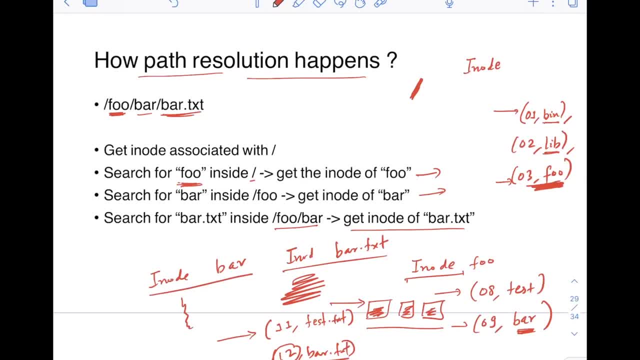 and these are very expensive actually. and also you are doing a lot of io operations, right? because these i nodes are typically first i stored on the disk, so you have to go to this, locate this, read this right. so a lot of i operations are there, so these operations are very expensive. that's why the 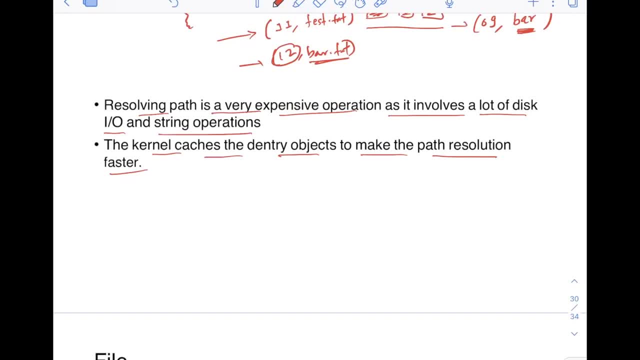 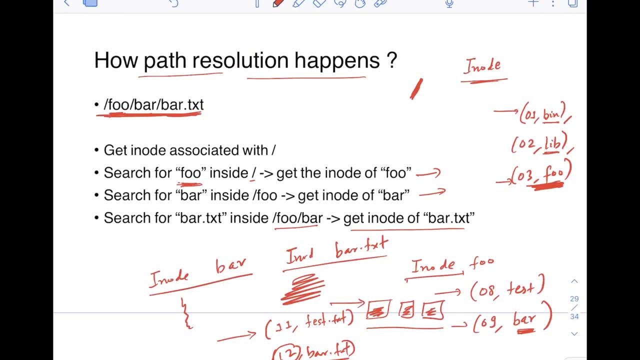 this is very expensive, right. so these are very expensive, right. so these are very expensive, right. so let's say, for example, here: find you would have got i node number associated with this path. right, slash who slash bar. slash bar dot pxt. right, of course, you have got iode for a lot of path here. 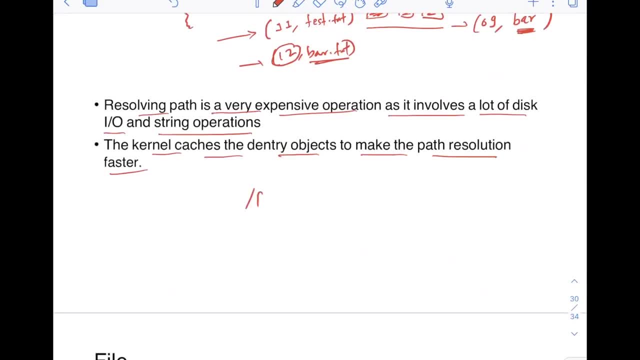 so some of the- for example, you have got i node number for this. what is the i node for this? okay, you have got what is the i node for this? you have got the i node for this. i've got i node for this. right and this mapping basically slash foo. is this i node? 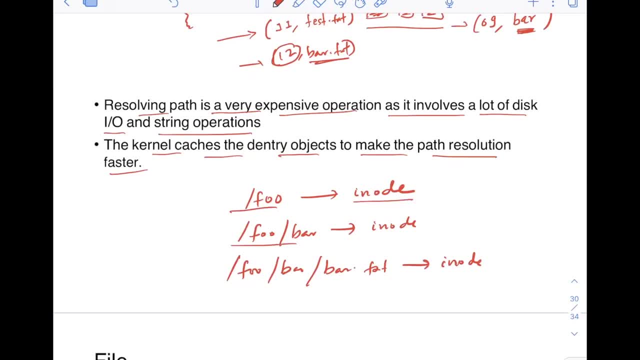 this is this i node. now the kernel does not want to waste this effort that it has done right. it has wasted a lot of time in finding the i node for this right. and what happened? let's say i mean some other user again opens this same file, let's say for reading right. 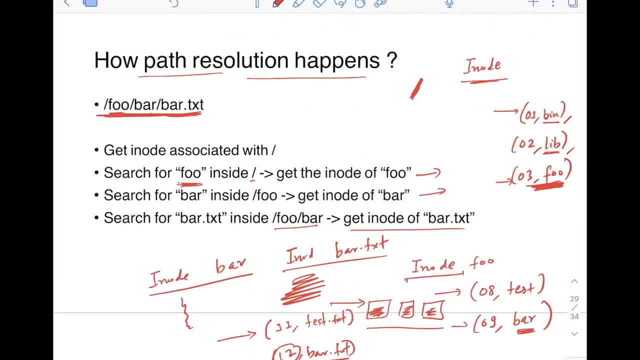 so does the kernel needs to again do this all operations? no, no, because it will. so. does the current again needs to do all these operations again? i mean, it can do, but it is very expensive, it will take a lot of time. so kernel will cache all of this, all of this mapping and 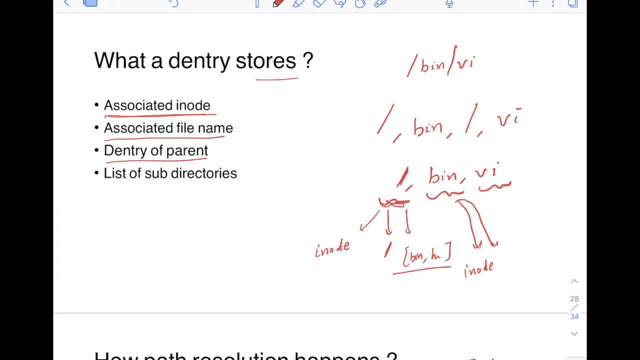 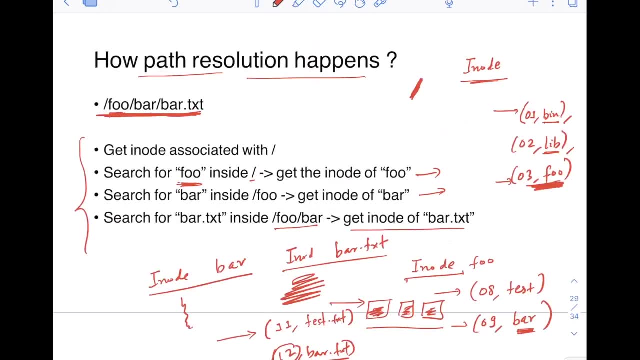 that's what your dentry is, then it is basically uh. if you see what adn提 stores, right, it stores the accelerated file name- and i know these two are very important. it stores the associated uh uh command. i node with particular file and these three entries will be stored. 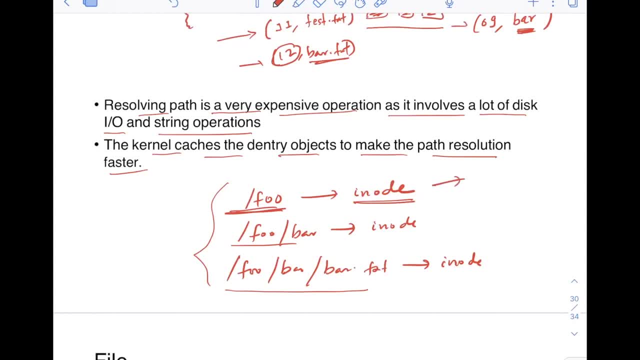 in the dendry right as different. so this is one dentro d1, this will be aнетケ, and this is going to be a separate entry right, they are all by Philosophical Futures and so, and another dentary d2, dentary d3, okay, and this is stored in the main memory itself. this will be. 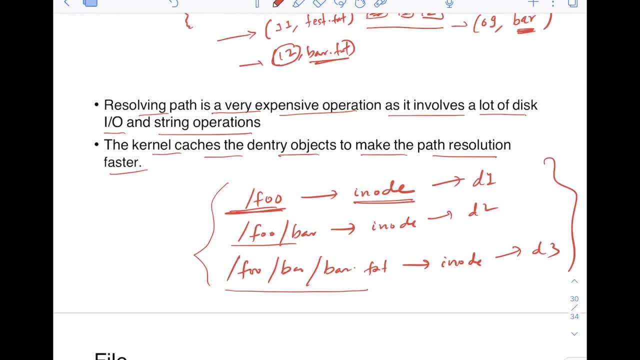 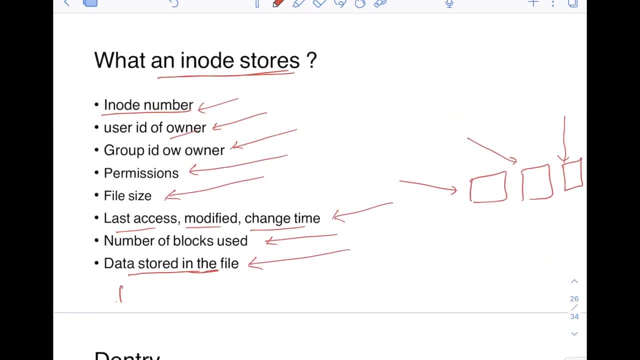 caged. basically, okay, and one of the important thing you would have seen- i'm not sure if you had noticed that, but i know- does not store the file name. okay, what is so? i know it stores a lot of information about the file and directories, right, but it will never store the file name. uh, in this, 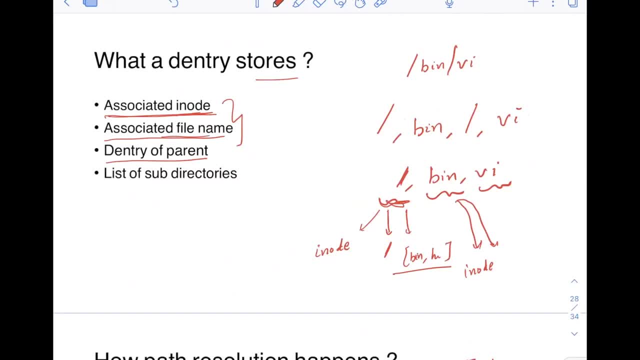 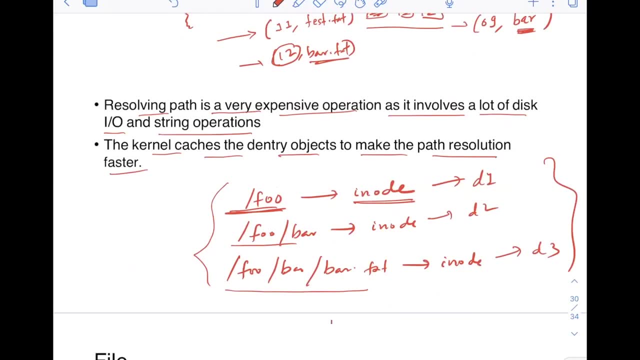 okay, the that is stored in the dentary itself. in the dentary stores the actual file name and then then the inode. so the reason is that because of this, links are made possible in linux, like soft links and hard links. i'm not going to cover it here, but that's the reason that, uh, the in i know. 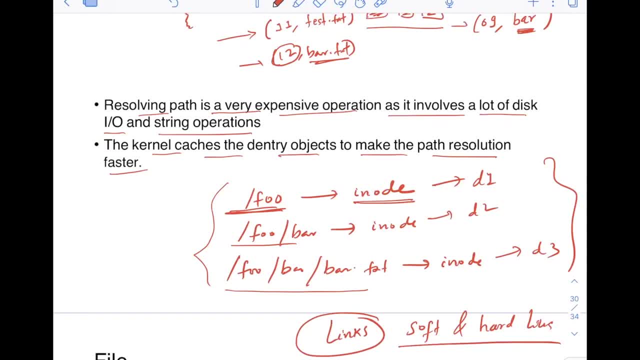 file name is not stored. uh, those are stored in the dentary itself. and i mean maybe in some other video i can discuss more about what links are- soft and hard links- and maybe you can also go online and read about this. and this is made possible because 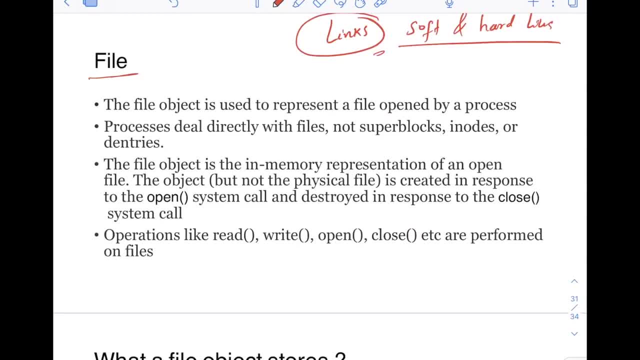 of this dentary. now the last and the important data structure in vfs is file. okay, now, file is basically very closer to you because you mostly operate on files. now the file object is used to represent a file opened by a process. so if you remember right in the c program that we have seen, 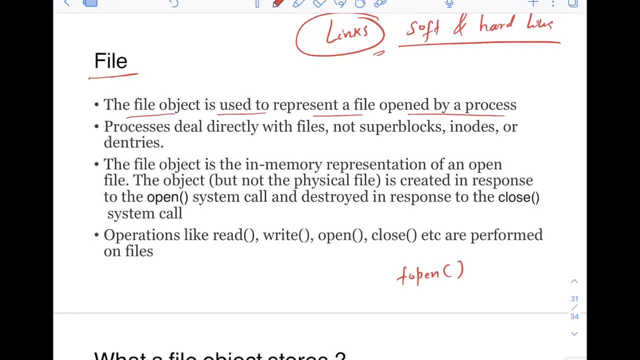 we have used app open right. so whenever we we are using app open, it is actually creating a new file object and of course, this file object will have a unique file descriptor that we have already talked right. so if you, i mean if you- create app open with some file- let's say i mean f1- right name f1, so it will have another uh. 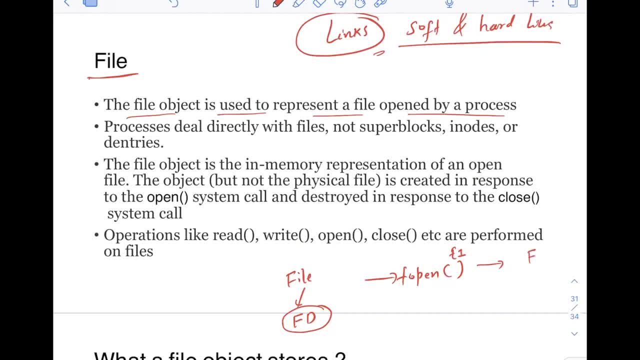 unique file object created for it. let's say, okay, capital f1. now if you do for f2, right file f2, it will have another unique file object created for this. of course these two will be differentiated by the unique numbers will be there for that. those are called file descriptors. 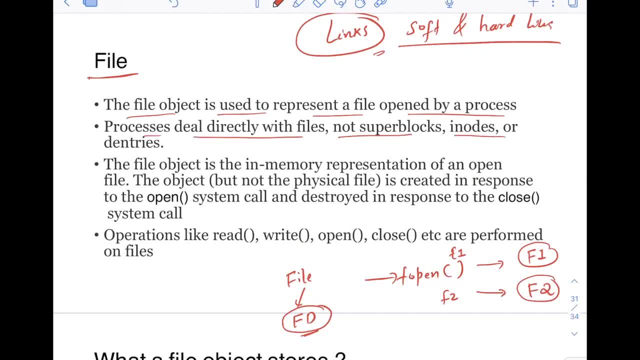 process deal directly with files, not super blocks, i notes, or dentaries. this is very, very important. right, your process, right. but in the let's say you are running this c program now it becomes a process when you run it. right now it only deals with this file object. whatever operations it will do, it will. 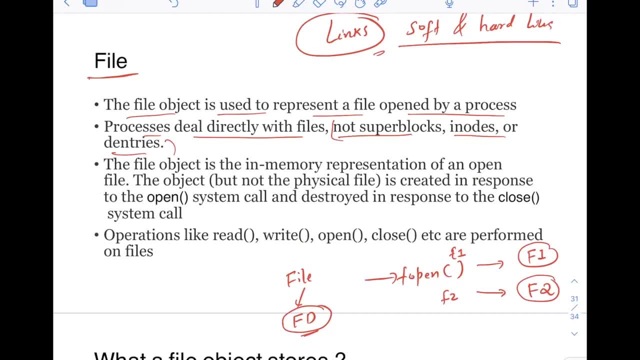 do on this file object itself. it does not know about super blocks, i notes or dentaries. it will not see that the file object is in memory. representation of a file. the file object is the in-memory representation of an open file. the object, but not the physical file, is created. 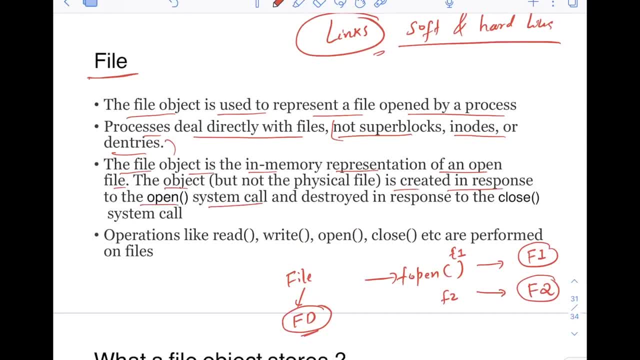 in response to the open system call. do remember. so, basically, app open will then call the open system call. and do remember: in this open system call, not the actual, i mean the file is created, not the physical file is created, it is only, i mean, in memory. right, you are actually representing a. 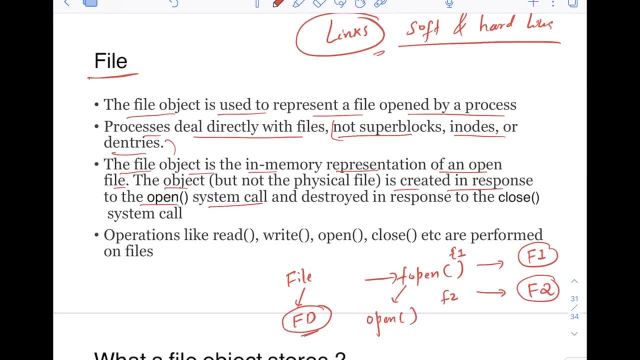 file. so that is getting created. that object is getting created and it is destroyed in response to the close. so when you- so basically when you do open this f1 file object is created, when you do close on this file f1, then this will be destroyed in them from the memory operations like read, write. 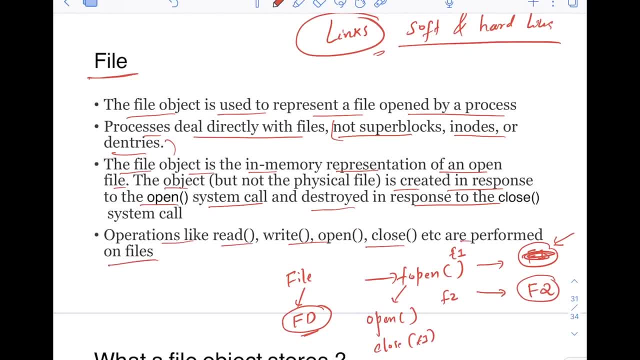 open, close etc. are performed on this file object itself, basically. so, basically, whatever you are doing right, read, write everything you are doing on this file object. this is the closest to the user also, and you typically will never see super blocks- i notes or dentaries, i mean whenever you. 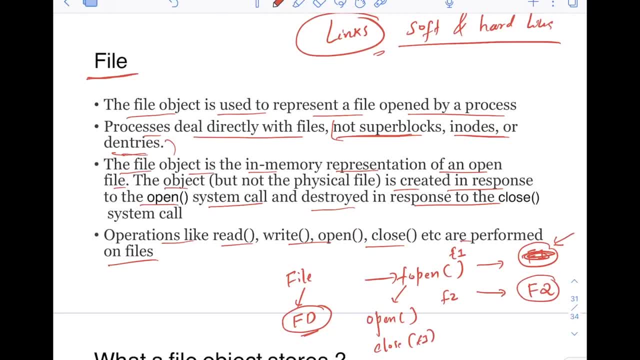 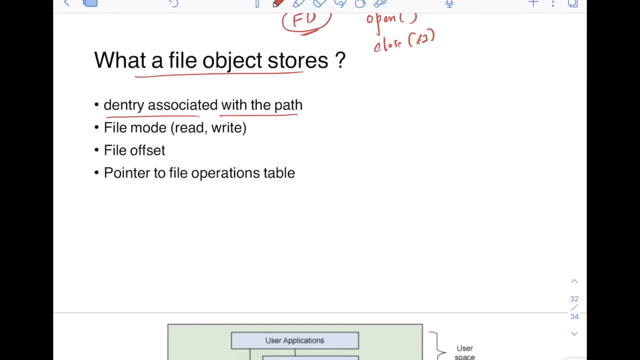 are dealing with process right, writing code or anything. so what a file stores? what are this file object stores? so it will store dentary associated with the path. okay, it will show the file mode, whether it is read or write. so whenever you do app open, right f open, you also tell right whether you are going to read or write, write or. 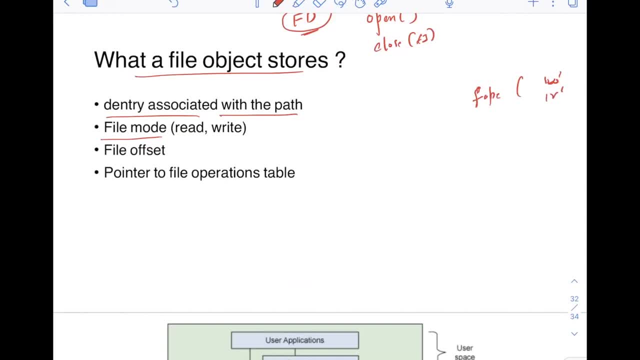 read, let's say: okay, so you are also providing that. so this file object also stored this. it also stores file offset, right? so if you are reading a file, if you are reading a file, so let's say: this is a file file. initially, maybe you will start with zero. i mean, if you start reading from zero, i mean 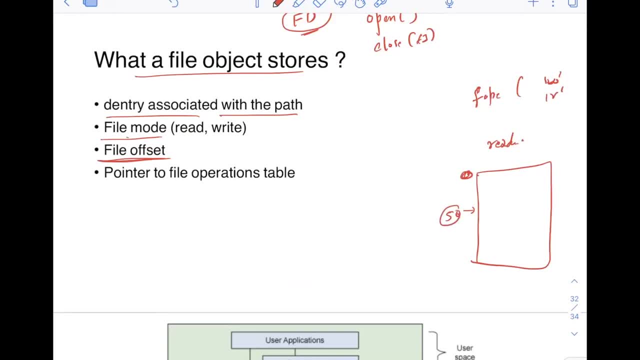 starting from zero, then you may reach 50 right. so this: now: once you have reached 50, the offset becomes 50 right. now it can again change. for example, it keeps track of where actually you are there in the file right. use it with the help of file offset. it also stores pointers. 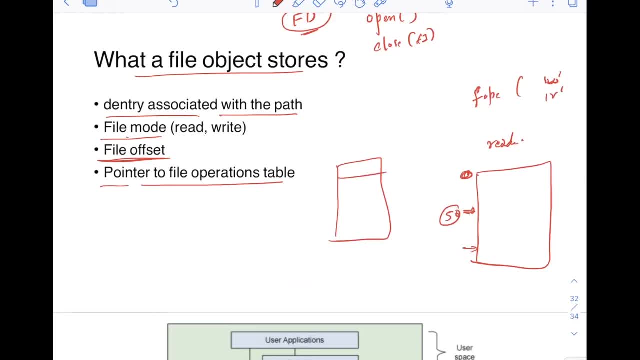 to the file operations table. so there will be table right for operations like read, write and all of this. so there is a pointer, uh, this, i mean this. let's say f1 is there right object. i love that this is store a pointer to this and then you can call this: read, write and. 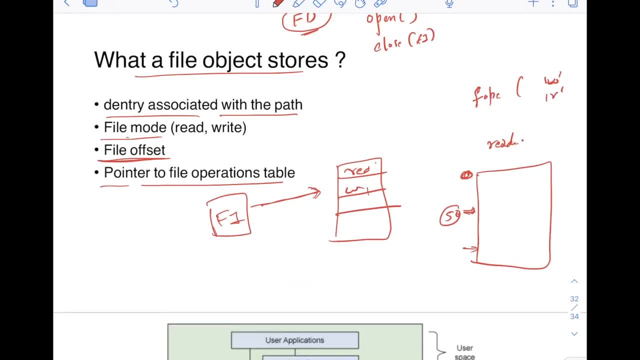 all of this, basically, i will again at last go into details, uh, i mean, and also at last, what i will do. i will, i will connect this four, basically. basically, when you are actually uh reading or writing a file, what actually is happening, i will connect, uh, this four. 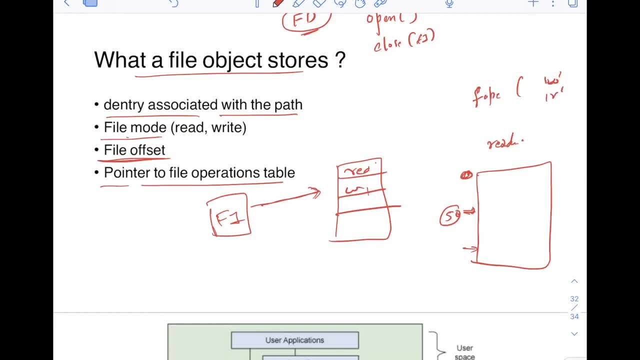 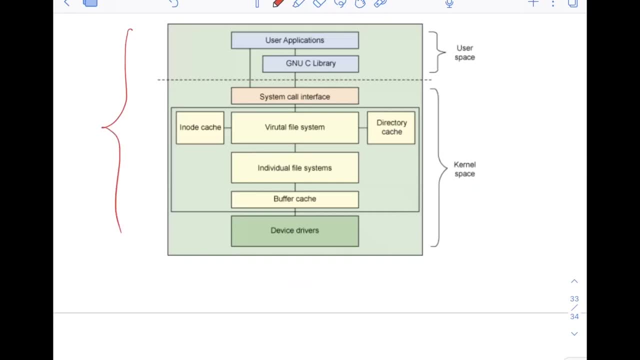 with that, basically like file object entry. i know that super block with that. oh, this is the uh kind of, i will say, diagram for uh, this i mean how i'm in the file picture right, uh is interacting with others also, of course, one thing is left here. let me draw. 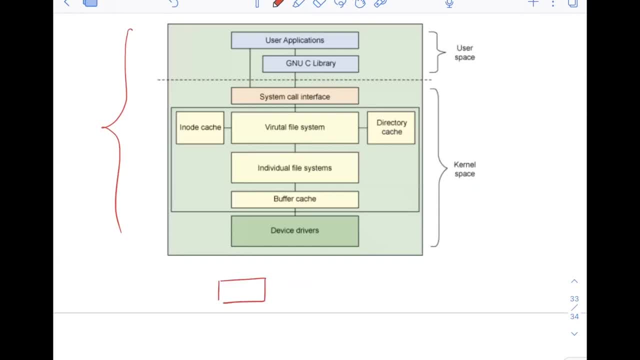 that also at the bottom. you will have this uh, devices, basically that is not drawn here, but you will have devices like maybe hard disk- is there, um, um, maybe you have keyboard also here, maybe floppy disk. let's say, if you have floppy disk you will have at the bottom. you will have also devices that is not shown here, of course. 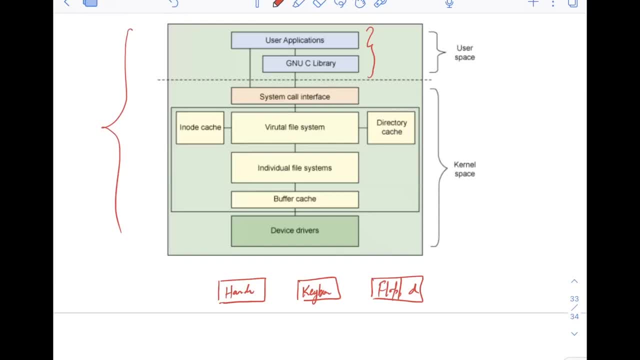 in the user space. you have user applications and uh c libraries or whatever libraries are there and you are writing the code here. so whatever code, the c program that i have written, that is uh executed in the user space here right, using some libraries, for example. and then, for example, when i uh use, for example, right uh app, open right in that program, right. 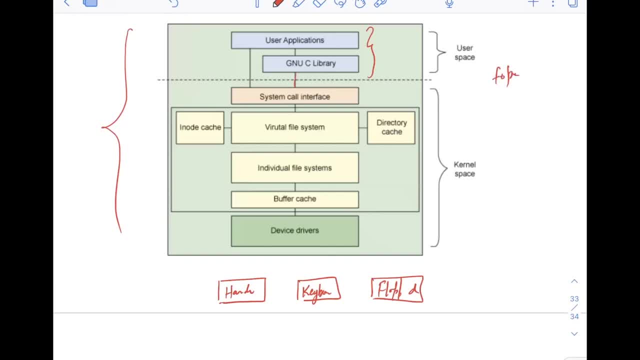 in the program, right in that program, right in that program. now app open basically, and of course, if f opened will be, will run in user space, but then it is going to call open system call. so when open system is called and system call is called, now the trigger 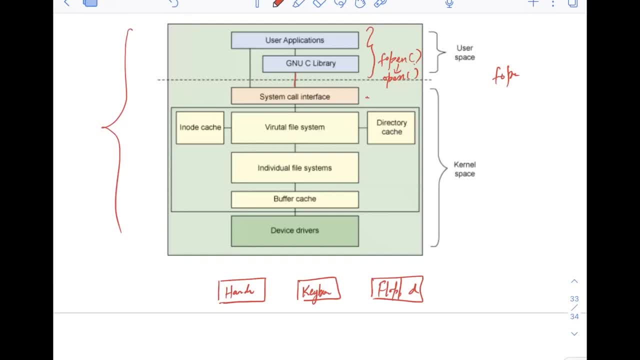 will go to the- i mean system call interface which is there in the kernel space. basically, now, okay, now, basically system call interface. so for this and all this file, uh, operations right, like open feed, right, okay, right, close, okay for this, what will happen? all these calls will then go to virtual file. 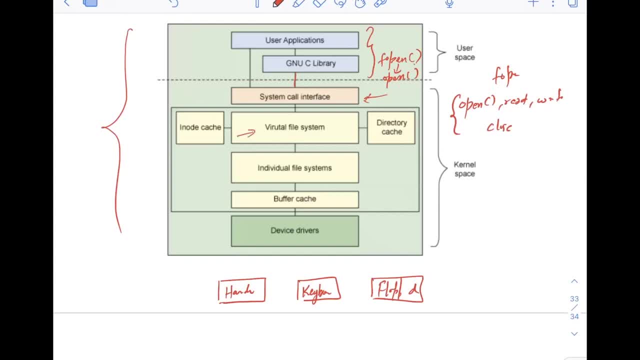 system. okay, i mean, if the system call is different. okay, let's say it is fork system call. okay, then fork will not go to vfs. vfs is only for file system, uh related system calls. okay, so for this four, six term calls. now the control will go to the virtual file system. but for 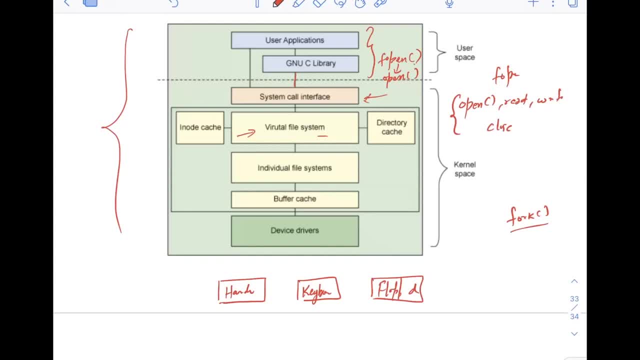 fork. it will be different. it will not be same. this virtual file system also has this directory cage. that is dentary case that i discussed right. you also cache all the mappings of files and inodes. inode cache is also there, so inodes are typically stored on the disk. but again, 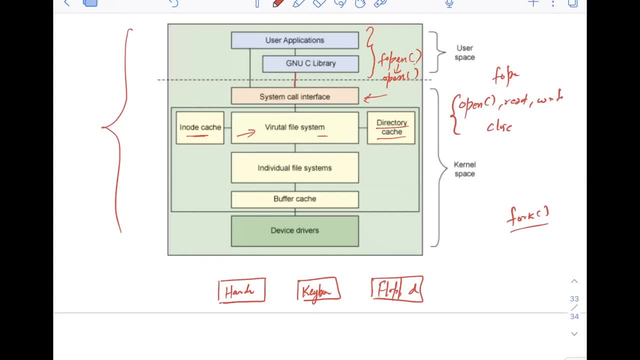 accessing disk every time, uh, when you need data about files, is not good, right? so the kernel also caches all these inodes in the main memory. then, after vfs, so once the open, as i so, if you remember, uh, one of the diagram, right, sys, right, that diagram. okay, now once. 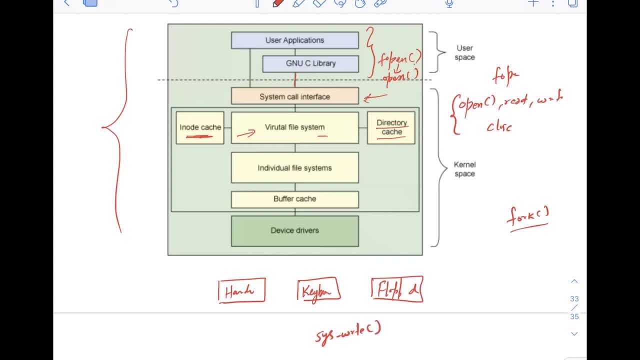 you do sys right here, right, then it will go to the individual file system, right? the individual file system has to implement this, right? it can implement it anyway whatever it wants to. right, then there is also concept of buffer cache, and buffer cache is again to uh. so if you want to cache this data, right? 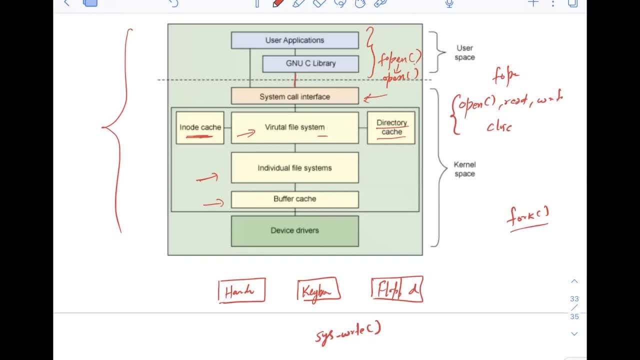 some data will be uh written in the disk. some data will be getting uh uh read from the disk, right, so that can be cased in this buffer cache. i am not going to discuss more about buffer cache here, but you can read more about buffer cache, right, so you can read more about. 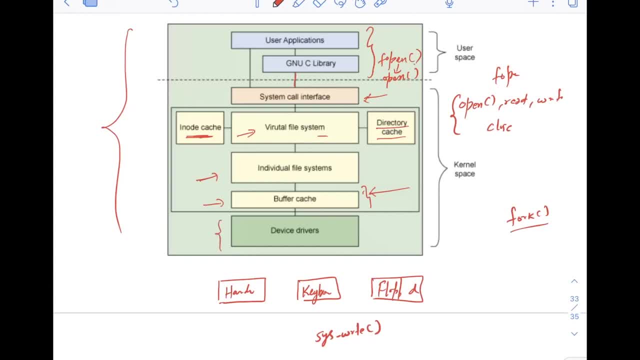 this, then device drivers are also used, which are again closer to these devices. for every uh device, there will be a separate device driver and become, i mean, basically, device drivers are used to communicate between, i mean, this device is right- actual devices itself, and then, uh, they will be used with the help of device drivers. you will be able to read: 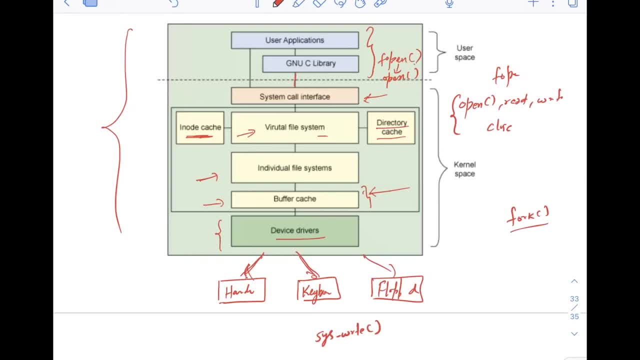 or write or do anything basically. so this is a basically flow, right? so virtual file system will call the individual file system. okay, the individual file system will also file system of the buffer cache is used for performance. then individual file system will call the device drivers of those file system. i mean of those devices and then device driver. 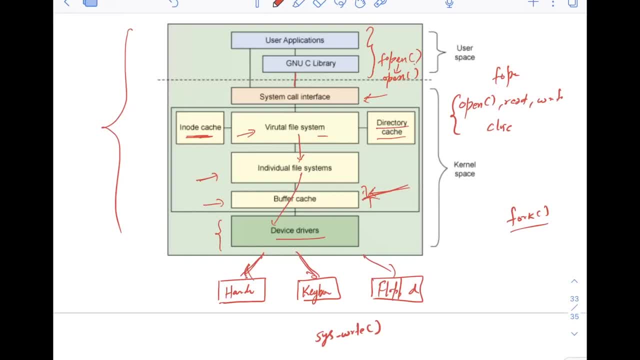 will basically talk to this devices, and that is the kind of eye texture of the linux file system, basically how everything connects to each other. so now what we will do is we will try to connect like how dentry, inode, superblock, right and file object- all of them helps in. 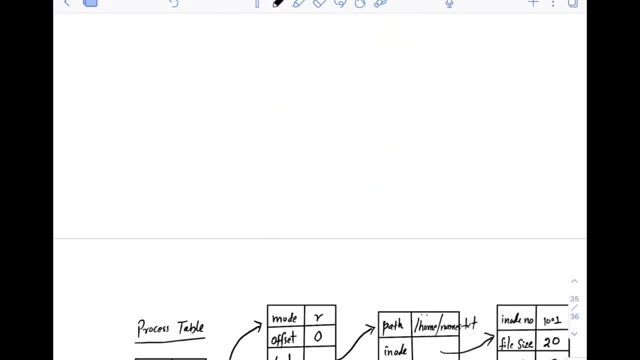 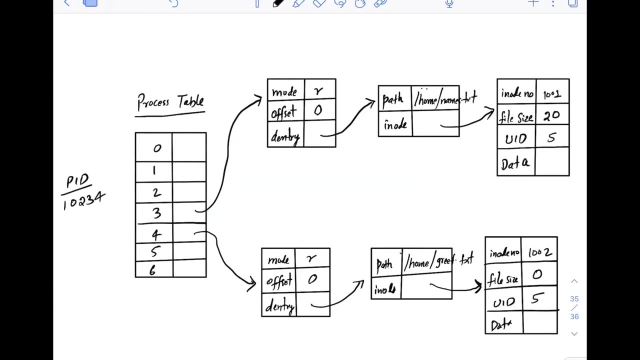 actually reading or writing a file. so this is a diagram here that i have drawn here to make you understand it easily. so if you remember the code of that c code, right where we were opening the file, like two files- one was namestxt, okay, another was greettxt, okay. so we were. 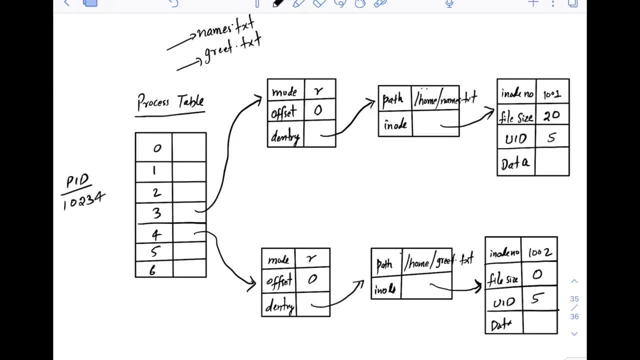 reading content from this file and then writing to greettxt. that's what we were doing. then we will run that c program. so let's see how using vfs that is done. right, how, with the help of vfs that is done. i mean all the vfs objects, basically okay. so, of course, when you 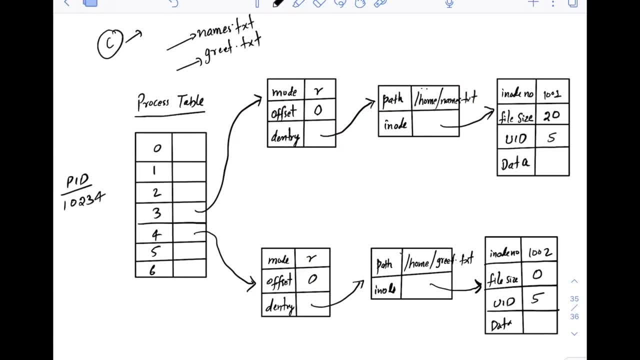 run that program- that c program was there right. when you run that program it will become a process and it will get a process id. let's say the process id is one, zero, two, three, four. and this i mean if you remember from the uh on my discussion on process right when i was. 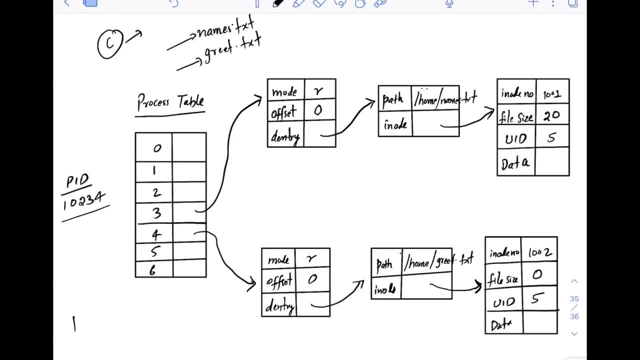 discussing, discussing about process. i told, for each process a process control block is created, right, and in this process control block a lot of information about process is stored. so one of the information is also called, known as process table. so basically this process or you can call this process file table, basically right, so this is stores like these are basically. 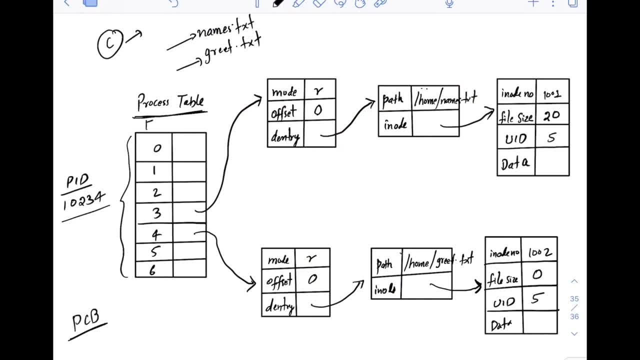 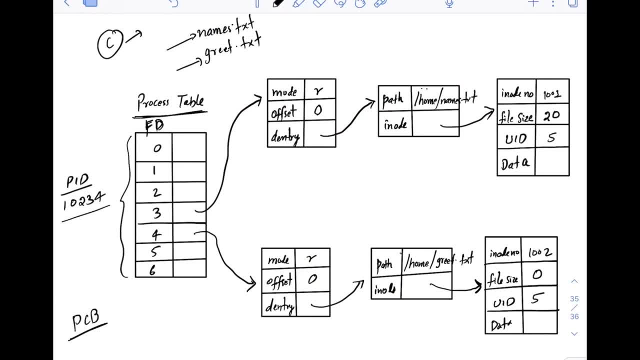 right, more files you can read. also more files you open uh in this process. this list will continue to go on. similarly, each process has this process file table. okay, these are the file descriptors here. so 0, 1, 2 are typically reserved. so these are reserved for uh zero. 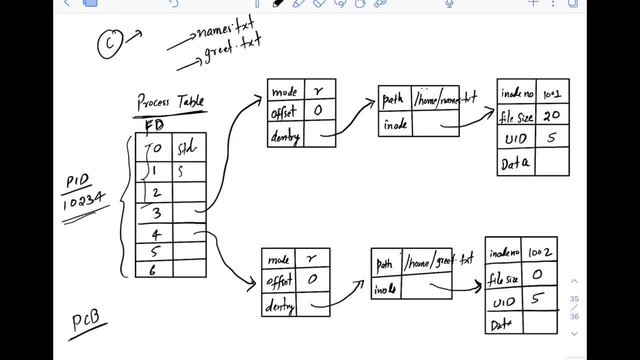 is for standard input, one is for standard output, two is for standard error. so these are reserved, zero. one and two are reserved for this: uh, this input output error. so all output and a standard input, standard output and standard errors. but from three, four, five, six, seven, you can like open any file in the, i mean c program, right? so when you open the 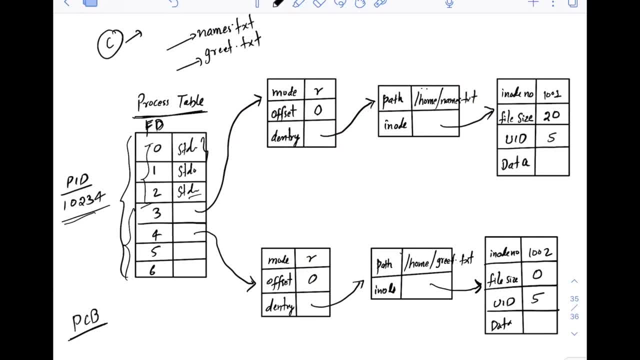 first file that was names docs txt. it will typically be given this: the first uh file descriptor that is not taken. that is three here, because zero, one and two is already taken, so three is the one that is free. so three will be provided for the uh names dot txt file descriptor and three. 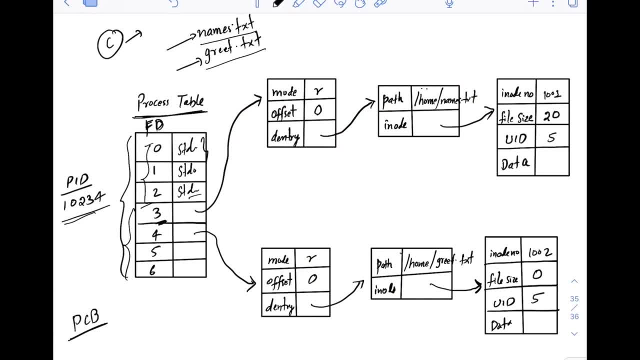 will be provided for it, for grid dot txt. the next one, that is four, will be provided now, for i, as i told, like which object is closest to the user or to this program. it is the file object. so this is your. now you have the file object here. of course, this is dentry, i'm not. 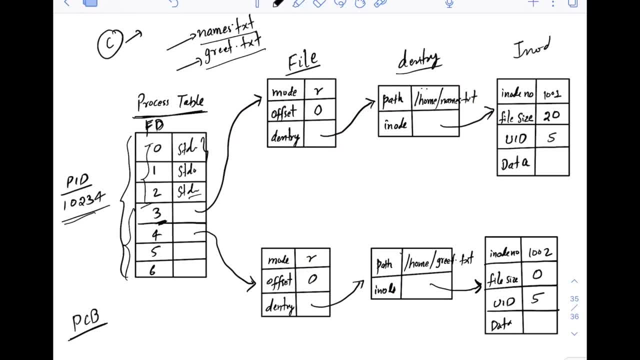 linked it, then you have, i know. so the closest object to this process actually is the file, so a file object will be created for both of this. so of course both are different. right, you are using app open on both of them. you are using app open on name search txt. then you are using app open on. 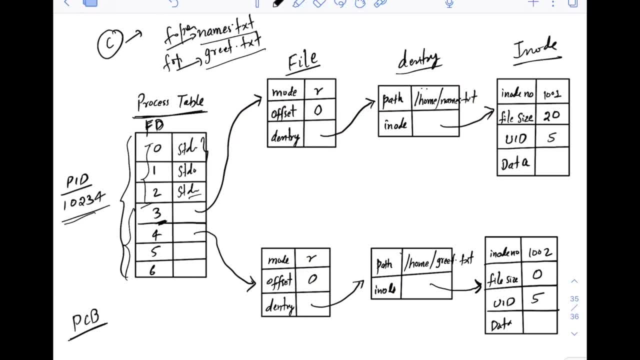 gridtxt and for each open call a different file object is created. so for for the first, first one, this file object is created and, if you remember right, we have opened using. we have passed r here and w here. so basically, first file we are opening in read mode and second file we are opening a. 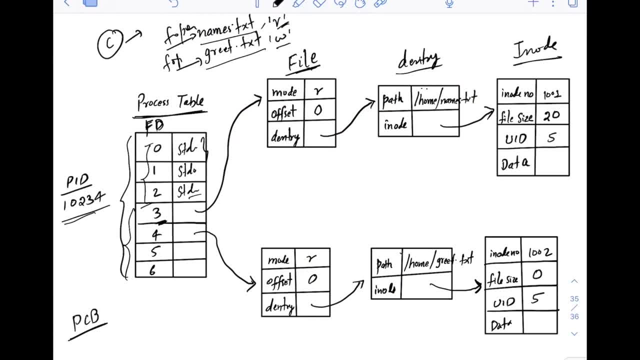 write mode. that's why you see mode is read here for the three third. third means the first five txt and offset is zero because we are going to start reading from start and then in this file object there will be a pointer to dentry. basically right, which is a dentry for this? uh, i mean. 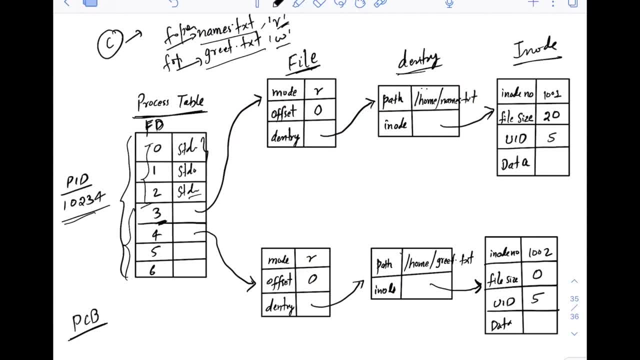 associated with this file, named txt, and this dentry, the important- uh, i mean important- parameter, and it's dentry. the important metadata are the path of the file and what is the i node for this? uh, i mean this file, basically right, so this dentry will store the path and all, also the i node, and 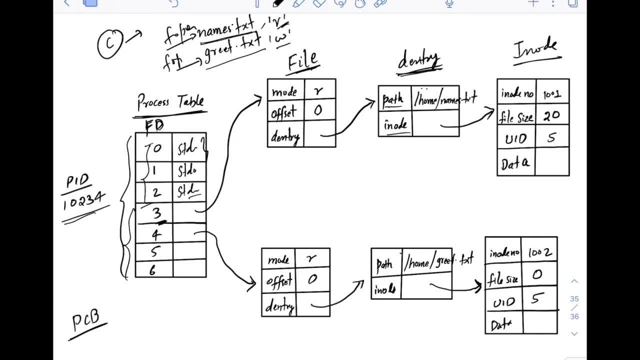 let's assume that the full path for this names of txt was slash home, slash name dot txt. okay, and of course, what is the i node associated with this file names dot txt. that i mean this. i not only pointing to that similar thing will happen for this. i mean the file descriptor 4. 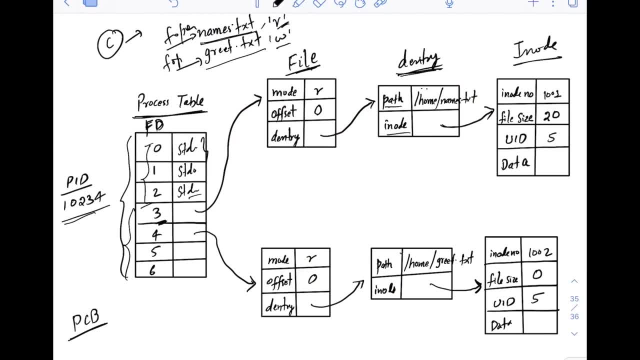 which was opened for. of course. sorry, this will be right here, not read, because second one was gridtxt. right, that was used for writing purpose, so that the mode will be right. offset will be zero. it will again point to a dentry object. dentry here. path will be slash home. slash gridtxt for second. 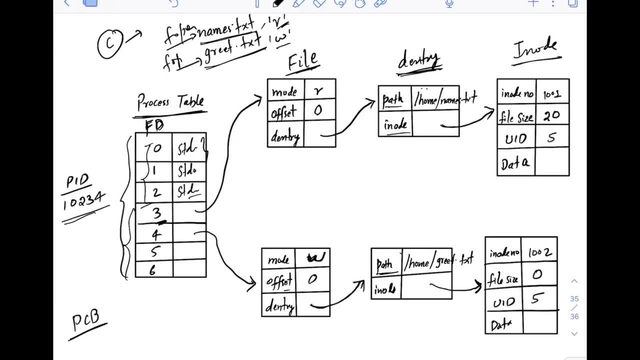 file and again it will point to the i node. finally you will have the i node, basically where actually the information about this uh file names of txt or gridtxt will be stored. so see the i node for first file names dot txt. so there will be some i node number. 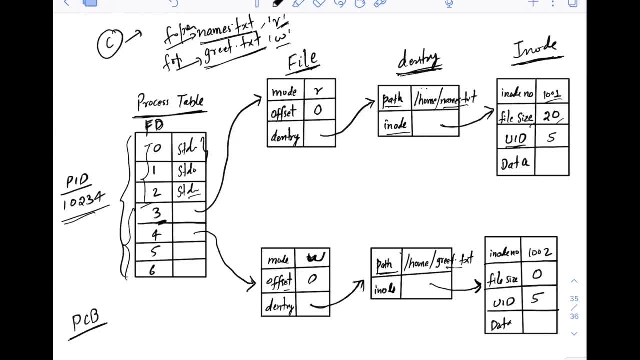 what is the file size? let's say it's 20 bytes. what is the user id of the own owner? let's say let's. let's say five. is the user id of the owner? then the actual data in this file. of course i have not drawn it, i didn't have a space here, but then you will have the. let's say you will have the. 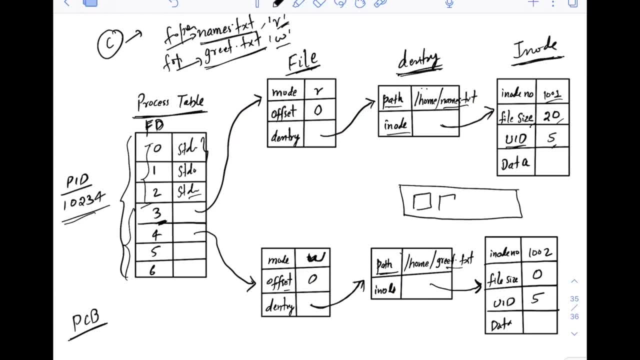 i mean disc here. right, a lot of blocks will be here on the disk and if this data will be pointing typically to this, i mean they can be multiple pointers also, it's not a single one. maybe there can be, let's say, in these two blocks, let's say this: uh, names of text. data is stored, so this data will be. 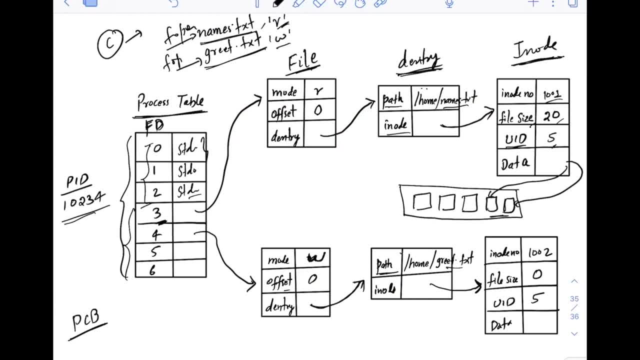 point to this similarly. uh, you have, i node here of the second file, grid dot txt. i know, number is there. files are initially zero, since, let's say you have not, you have just opened it, but you have not written anything. you user id is again, let's say, file data again. so once you start writing, right. 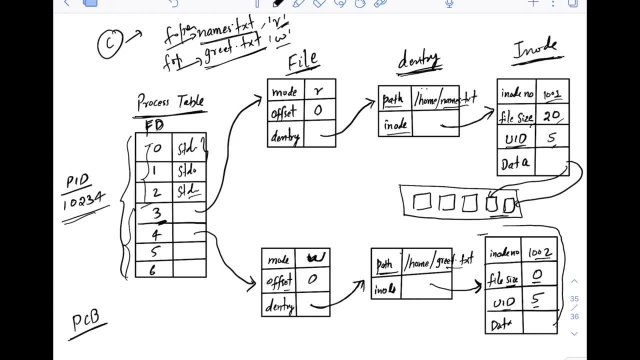 once you start writing, then kernel basically will allot some blocks for this. let's say maybe this, and i mean, when you have finally written this and let's say this one, okay, we will point to the data block. these are the basic data blocks, data blocks on the disk. okay, so this is the overall structure. 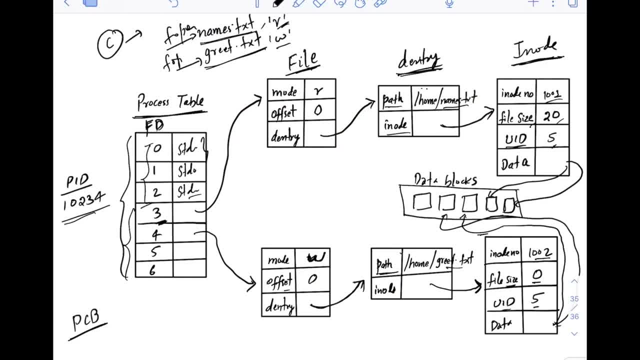 of what happens right when you open a file for reading or writing. so similar thing will happen when you do this in the shell itself. right in the shell also, we ran cat command. okay, we ran echo command right for writing and cat for reading, right. similar things will happen in that case. but 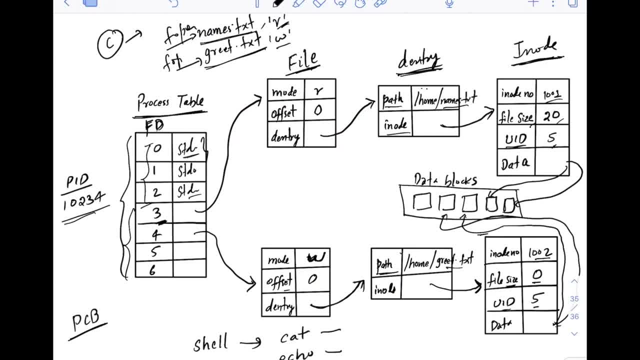 in that case, typically, what will happen? you you can use a standard input and a standard output, right? so in that case that's will be used for shell. but if you're writing so, even in the case of cat command, echo command, similar thing is going to happen. 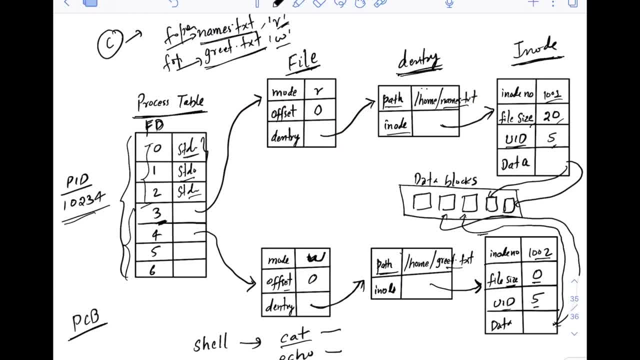 so you can read a file even from shell, right? you can read a file even from your code itself. you can use even python programming language for reading writing file, java, right. in every, each of these same thing, things are going to happen on the background in line of operating. 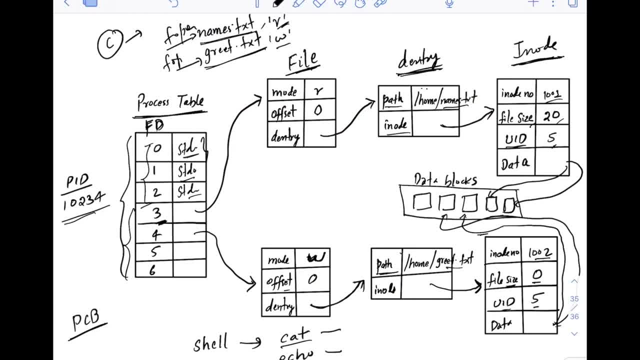 system. so i hope that now you have understood how this i mean four important data structure like file. dentary discussed much about super blocks here. the reason is super blocks are mostly used for, like, storing information about the file system itself, right? how many inodes are free? how many blocks are free? uh, what is the mount point? and all of these, right? so that's why i have 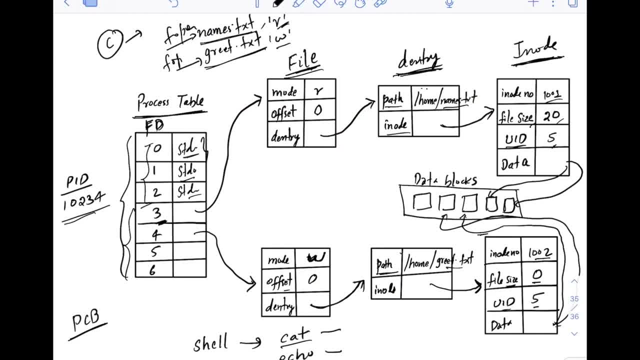 not connected much with super blocks here, but that is also important. basically, i hope that right now you will be able to explain, if somebody asks you right, what happens actually when you open a file or close a file or read to engine management. you will have to do all of that and the thing that is so important is that it can be�ed out once or twice, right. but if I have a very specific data space, i don't think there is enough data space to measure it right. so there will be a lot of data space in the system of? ¿don't know what that would work, and so it has been processed and the tools that unten 효bel are. 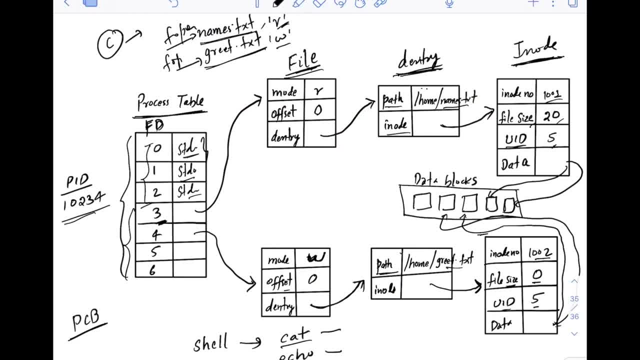 or read to read a file right, file right. you will now understand what's happening on the background with the help of vfs objects: what's happening, what's happening on the background right, you can connect this. so this is very low level and this is again. i mean, this is more kind of not. 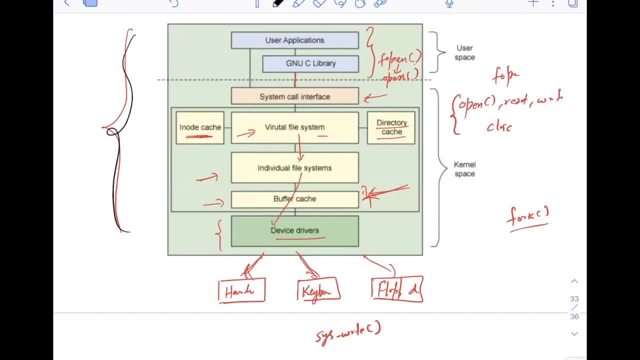 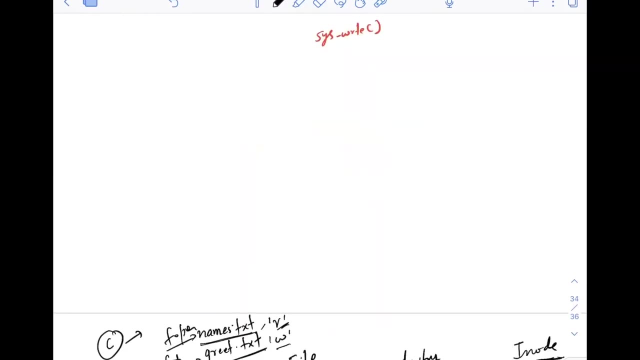 very low, but this is more of a higher level architecture, right, how everything is happening. so now this vfs i have broken down here, for example, right into different component that is not there. this is kind of high level architecture diagram of what actually happens when you read or write to a file, right? this is a very low level of how actually vfs helps in reading. 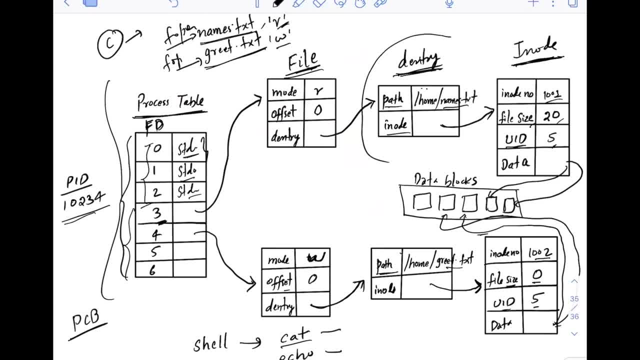 or writing to a file and this dentry would have been created, right? i have not discussed here how so karnal would have created this dentry object. as i told you, right, these are not stored on disk, these are. these are created and stored in the main memory itself. so, uh, i mean while resolving.